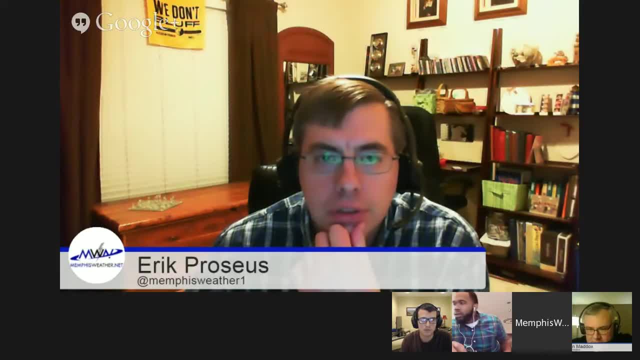 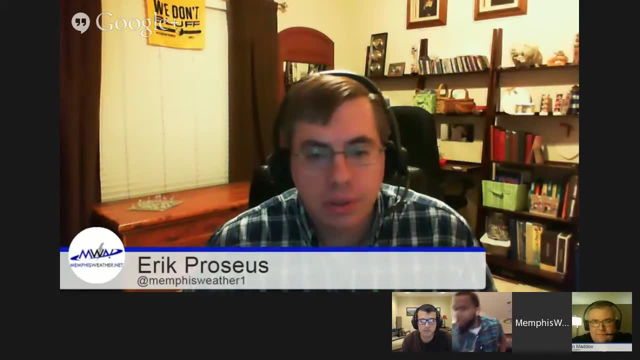 I'm still waiting to make sure we're out there here. Yes, we are. I think I've lost my hand. All right, we should have Patrick joining us here in a little bit. I guess I'll keep an eye out for him. 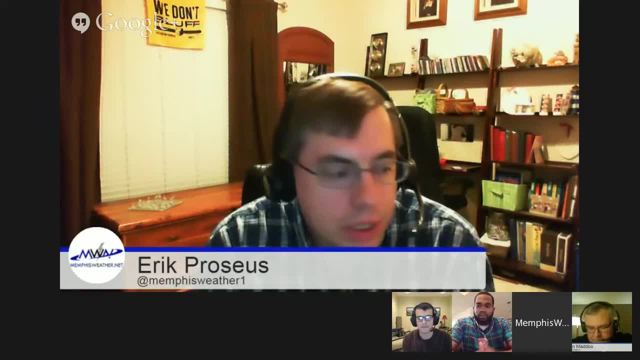 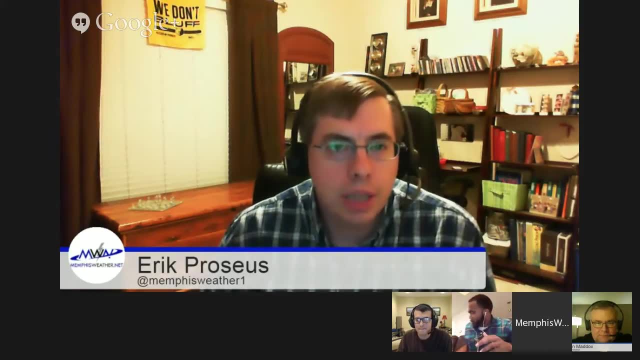 Good evening to everybody who's going to be joining us tonight or watching this, perhaps an archived version on YouTube. I am MemphisWeathernet meteorologist Eric Procius. I'm having a hangout tonight with you all to talk about some interesting topics, mainly related to winter weather. 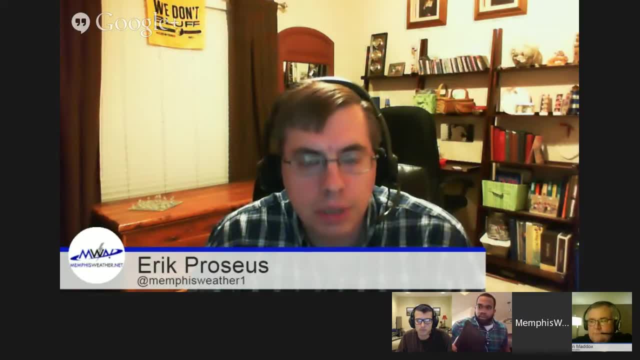 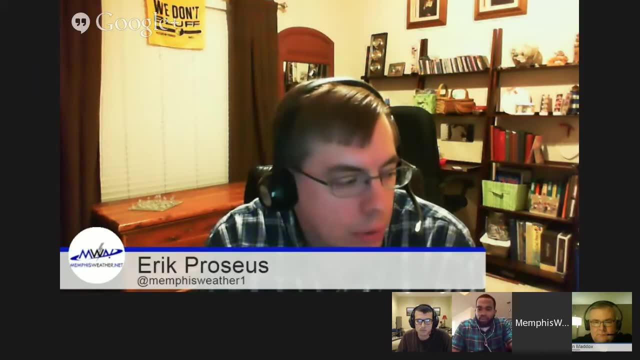 although we'll try to apply that across a broad spectrum of events that we might encounter throughout the year. This is the first of a couple hangouts I'm planning this month, and we'll talk more about the other one later on, but Tennessee Severe Weather Awareness Week is coming up in a few weeks as well, and we will be doing another one of those. 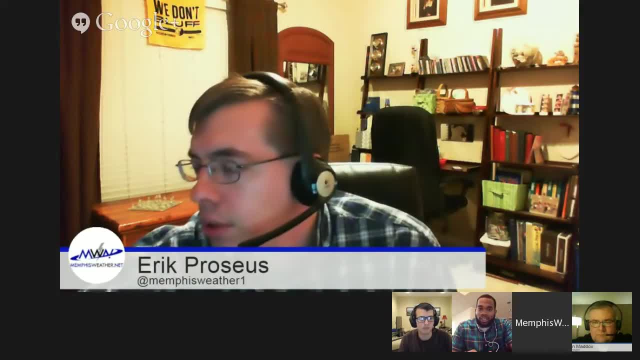 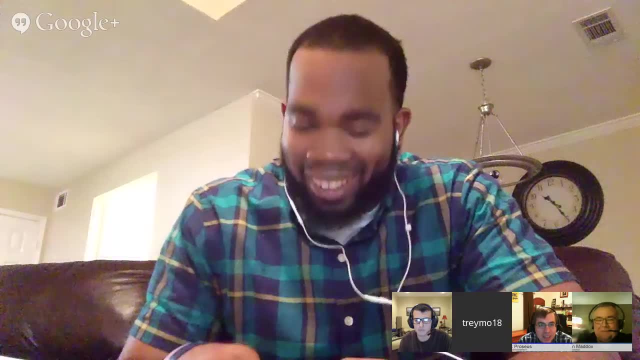 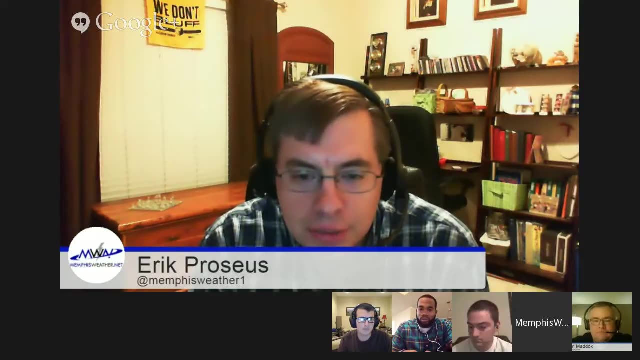 Is that going to be the third week in February, John, Do you know? Yes, it is there again. I've got to talk to you about that. All right, excellent, Good, We'll plan some great stuff. But, yeah, glad to have everybody with us tonight and we will start off by introducing our cast of characters here tonight. 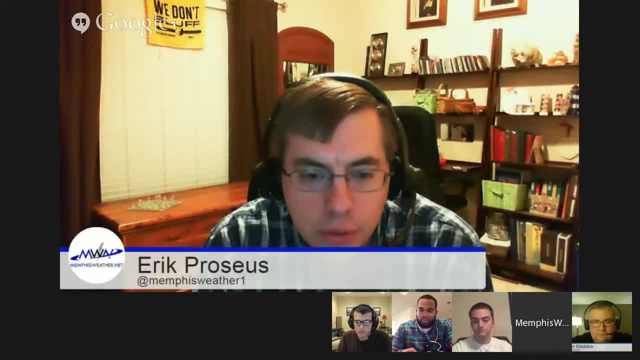 I'll start off down on my end. I don't know how you guys are seeing it order-wise, but John Maddox is down on the end, a veteran of MWN Hangouts and here with us to talk a little bit tonight as well. 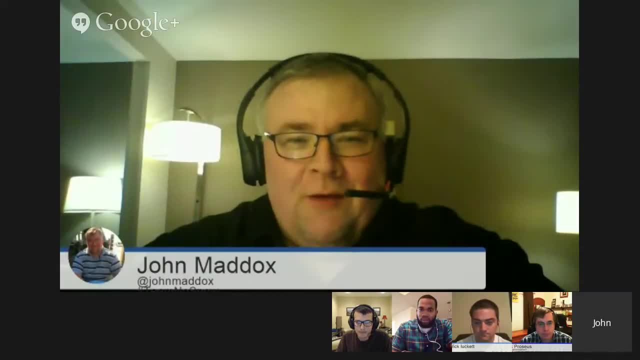 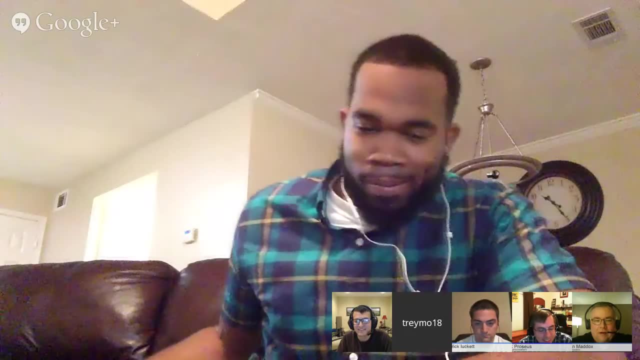 Welcome, John. Thank you, sir. I'm John Maddox, a veteran of MWN Hangouts, and I'm here calling in from the Tupelo Mississippi office, Memphisweathernet. this evening down here for a trade show. Other than cold, it's not too bad down here. 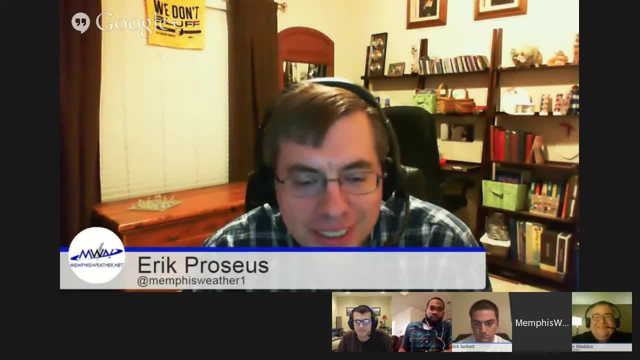 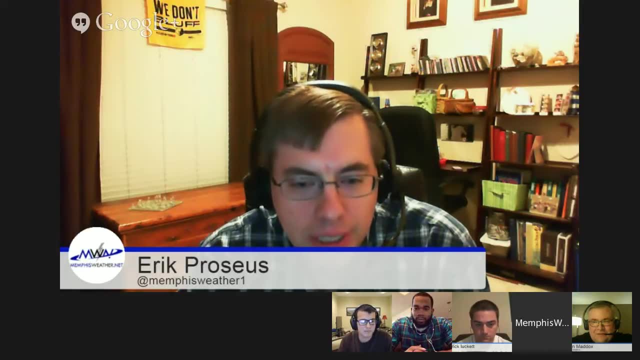 Excellent, Yeah, the eastern office that we have down there in north Mississippi. Glad to have you dialing in. Thanks for taking some of your time, away from what you're doing down there, to join us tonight, And next I'll go to John Moore. 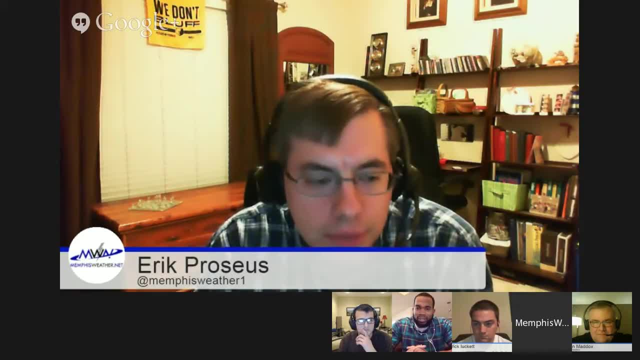 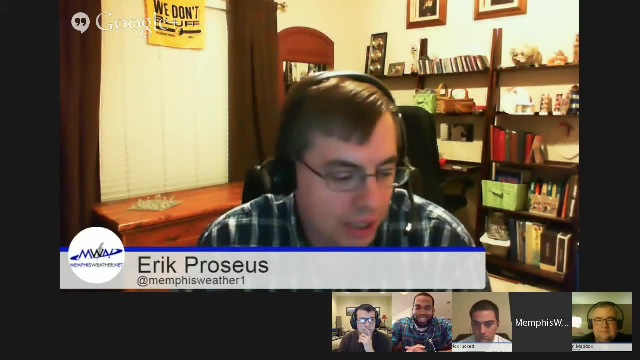 John is a meteorologist with the National Weather Service here in Memphis and it's the first hangout we've had a representative from the Weather Service on. that wasn't the Storm Spotter Talk, so we're glad to have John on. Good evening, John. 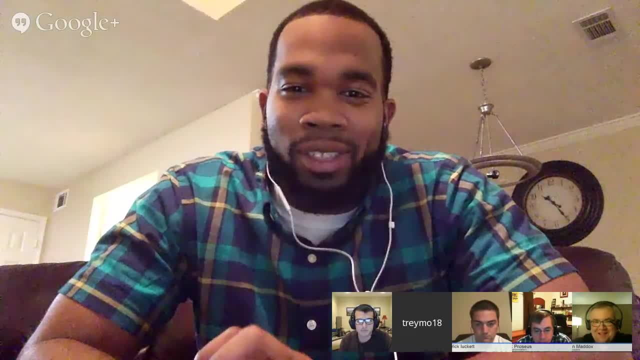 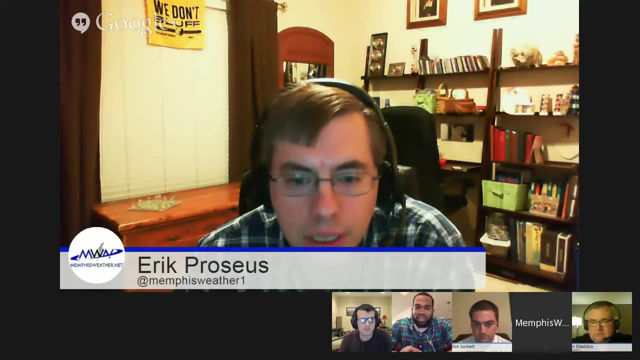 Good evening, Eric. I'm glad to be here. Thank you for the opportunity. Yeah, you're very welcome. Look forward to having the public sector side of things tonight as we talk through several different things. So thanks for being with us. 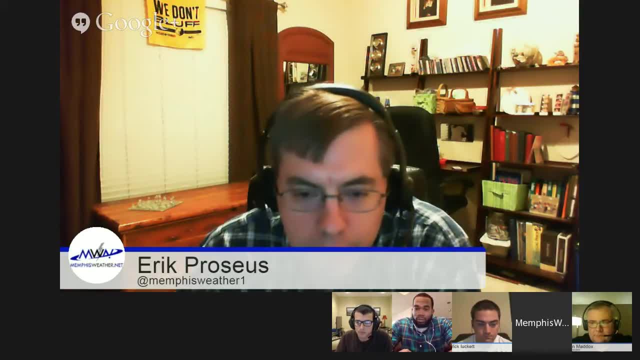 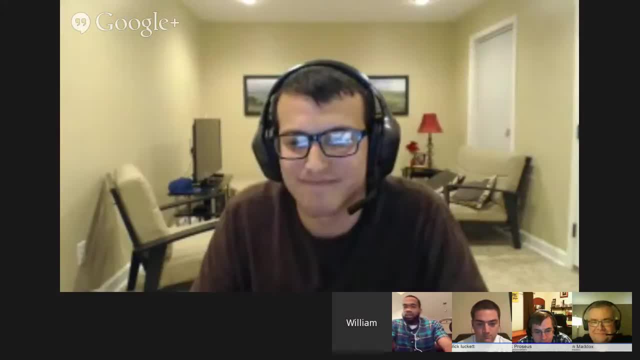 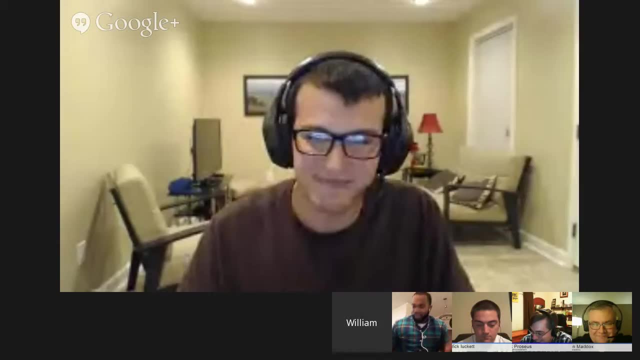 Chugging on along with grad school. so glad to be here tonight, Glad to have you. I hope it's a few degrees warmer down there than it is here, Just a couple. Yeah, You're closer to the beach, I got that to say for you, so that's kind of nice. 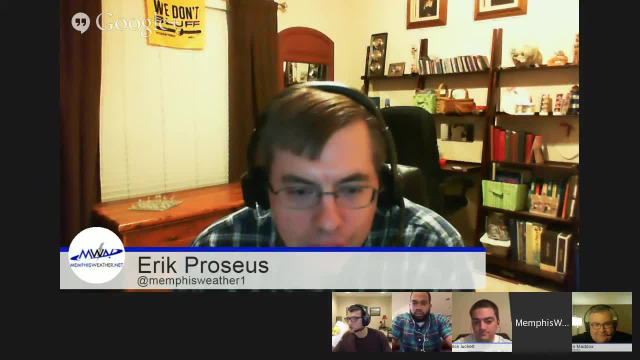 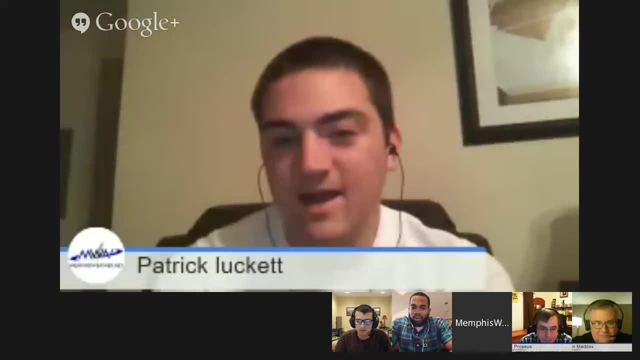 And also joining us tonight. MWN intern. Mississippi State grad student, Patrick Luckett. Good evening, Patrick. Glad to have you join us here. Not actually a grad student yet. Well, I'm going to promote you two. You're on your way. 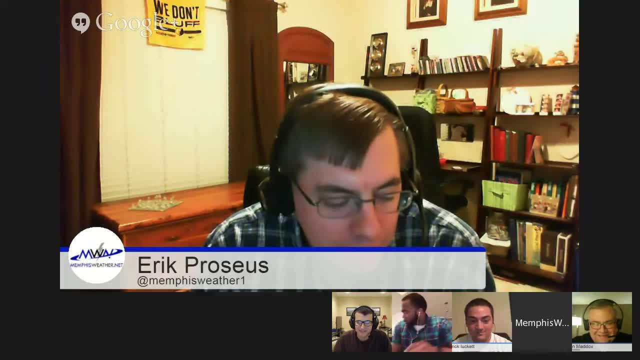 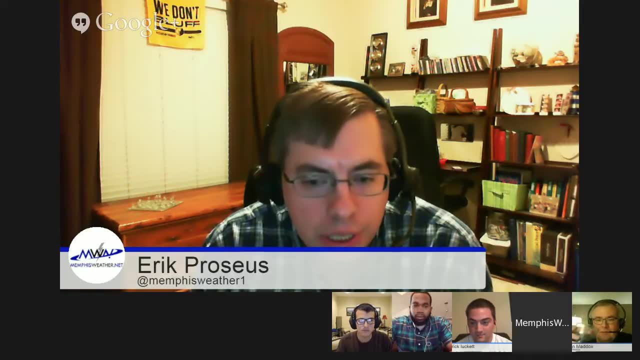 We know where you're headed, That's right. Glad you were able to come on tonight And hopefully you'll be able to take care of some live tweeting for us as we go through this evening. For those that are joining and watching, we will be using the WXChat hashtag tonight on Twitter. 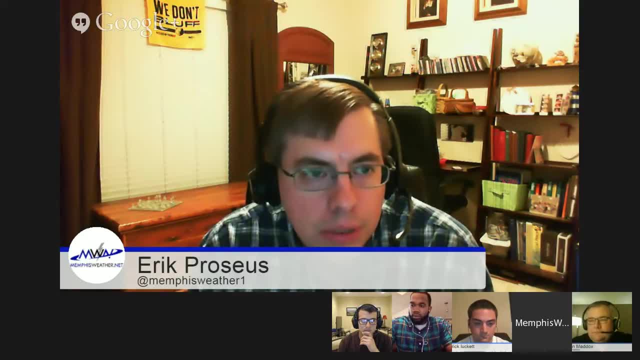 So if you have any questions or comments that you want to submit or just kind of follow along with the tweeting, you can submit those using WXChat or send them right to us at MemphisWeatherWeathercom. We'll be happy to answer those as we go through. 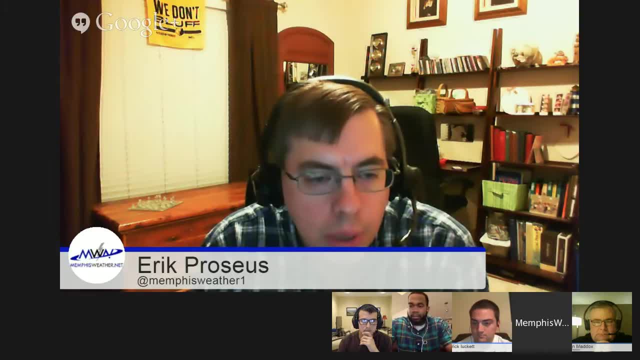 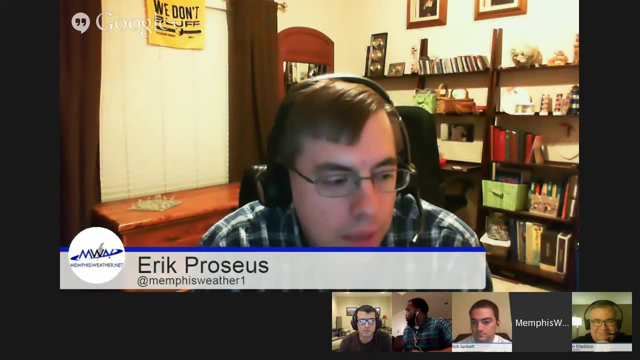 And we also are running this through the MemphisWeathernet website. If you're watching on there, you will see a chat window down below here below the video. Feel free to chime in down there as well. We'll kind of keep an eye on that. 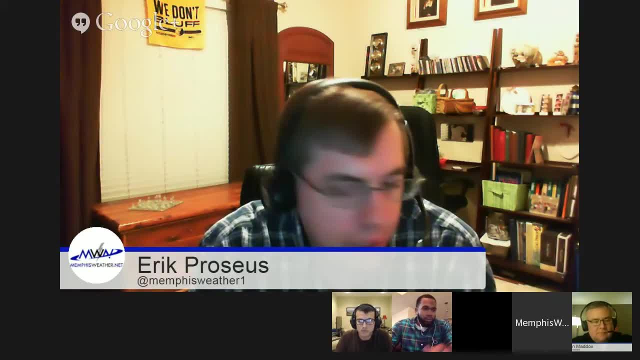 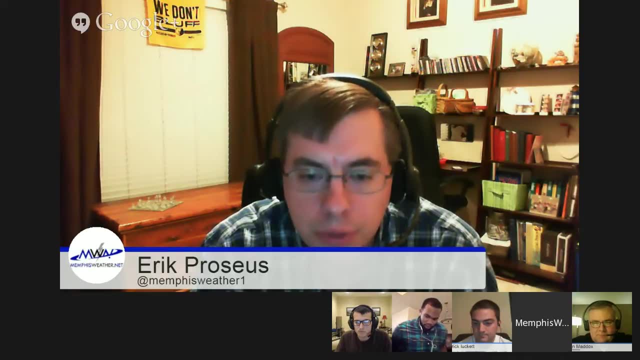 So, without further ado, we will have one more guest hopefully joining us in a little bit. Ryan Vaughn from KAIT-TV in Jonesboro is hopefully going to be able to join us for a little bit this evening as well. He's got a previous engagement and a 10 o'clock broadcast, so he's going to try and squeeze us in. 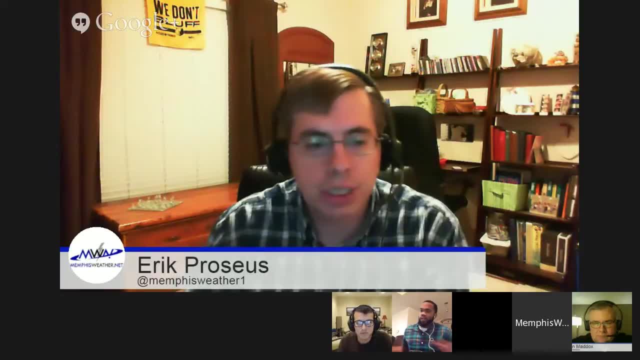 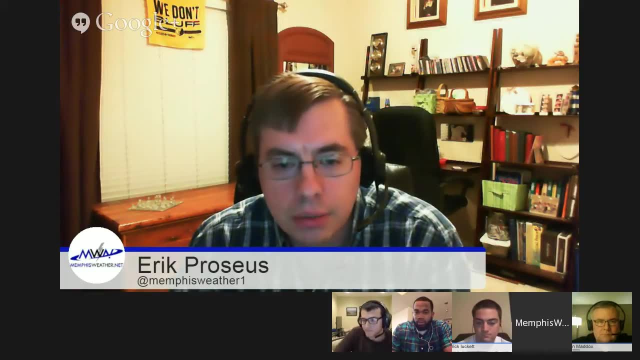 But we're going to jump right in to let William share a little bit. We want to talk first of all about possible snow chances tomorrow evening, and we'll see how that plays out. So, William, would you go ahead and take it away. 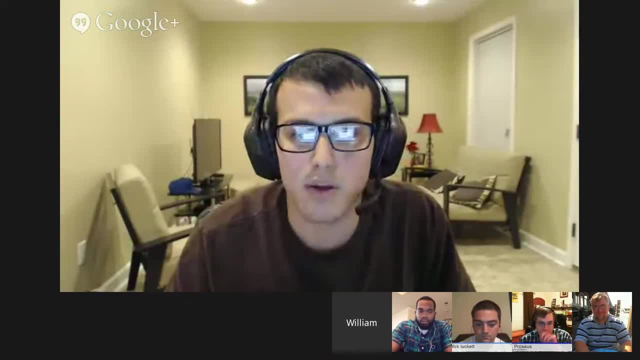 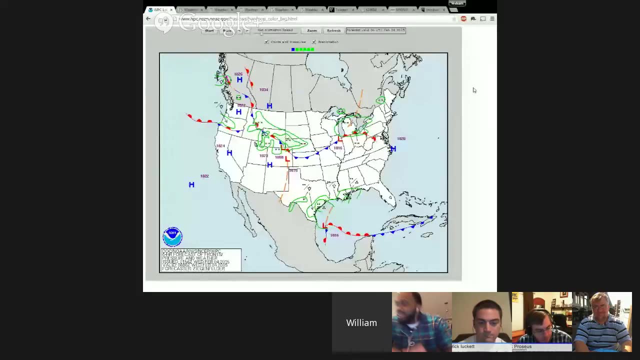 All right, Yeah, I'll cover this. So probably what everyone's hoping for in Memphis is finally some flakes, So we'll see. Hopefully we can make that happen. The first thing we'll pull up here Just to give you an idea of overview of everything this is from the Weather Prediction Center. 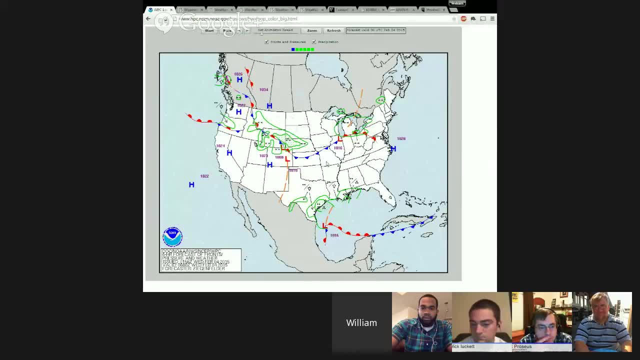 And even though it's been pretty cold here, we've still got more cold air coming. There's a system brewing to our north that's getting its act together currently. So before we get colder, we will get a little bit warmer. Tomorrow it looks like we'll get up into the 50s with a little bit of relatively warmer air coming in. 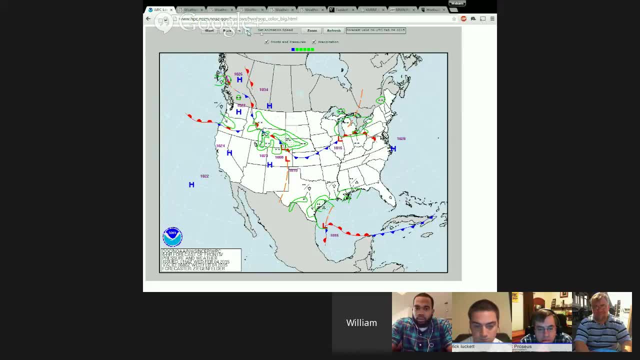 But that's going to help set the stage for snow chances, because with warmer air we're also getting more moisture coming in. So as we go through this, This loop- this is getting into Wednesday morning- That front, that cold front north of us, will just slowly start to slide south. 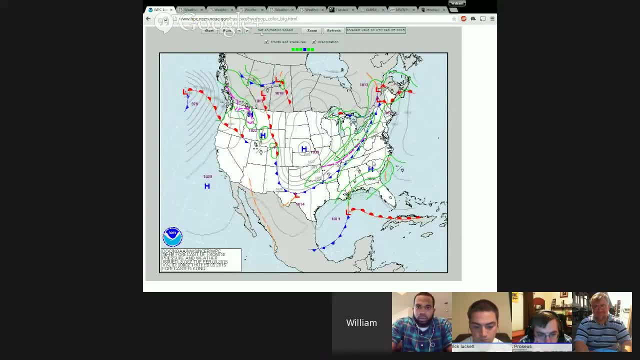 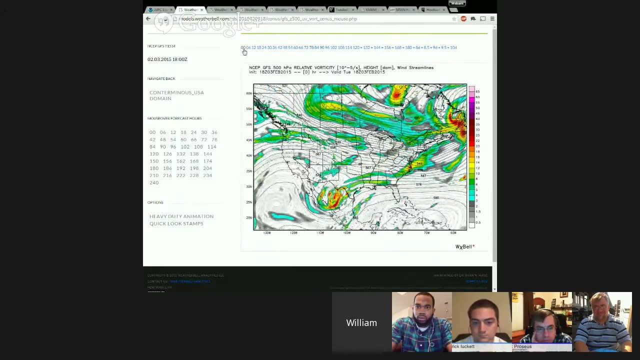 And by middle of the day Thursday it will be coming through. So but earlier than that, earlier in the morning, is when we'll have our real snow chances. So I'm not going to get too super technical or anything, But just to give you an idea. this is one of the maps we look at in the higher levels of the atmosphere, or what we like to call the mid levels, I guess, of the atmosphere. 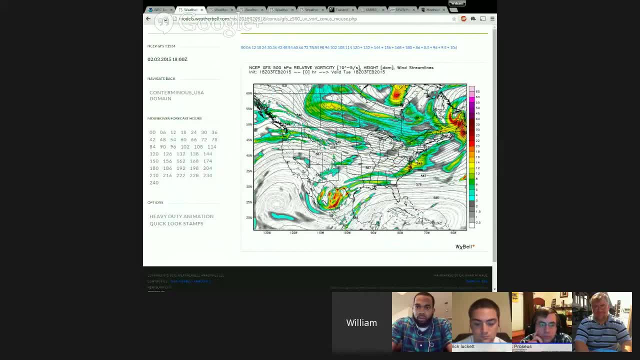 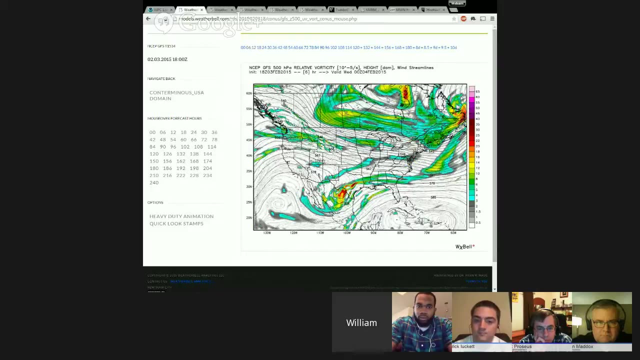 And These black lines just represent heights, or you can think of them as pressures, with lower pressures, typically the south, and higher north, while the colors you can kind of just think of as atmospheric energy which will bring potential uplift and hopefully precipitation. So as we slide through this, our trough that's going to be bringing the system through is actually all the way up in Canada right now. 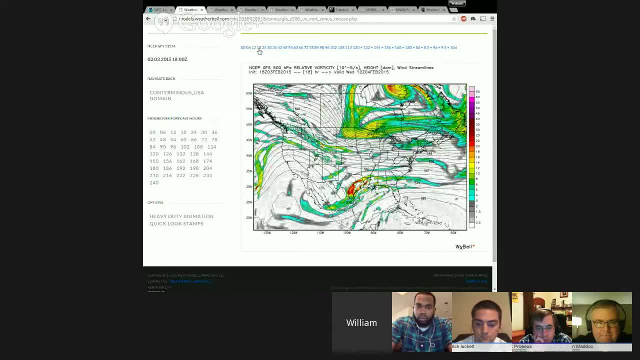 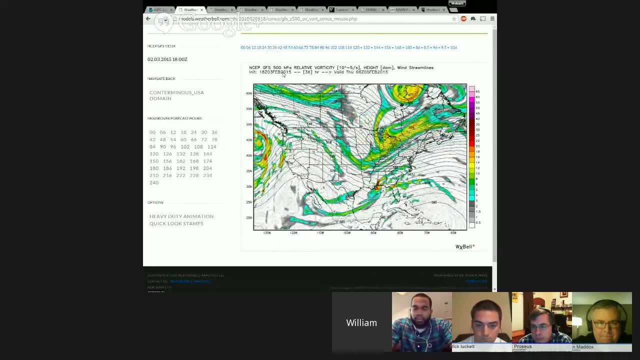 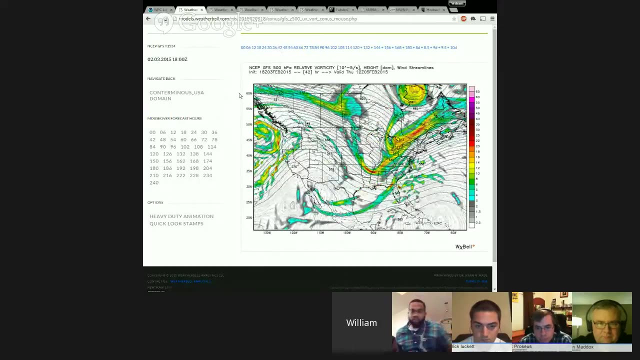 I'm not sure how well you can see my mouse, but this trough will start to slowly dig south and we'll be coming through our area by Thursday morning. So here's the. the colors represent that energy, Uh, that trough tilting down towards us and as it comes through, that's when, hopefully, we'll get a little bit of precip. 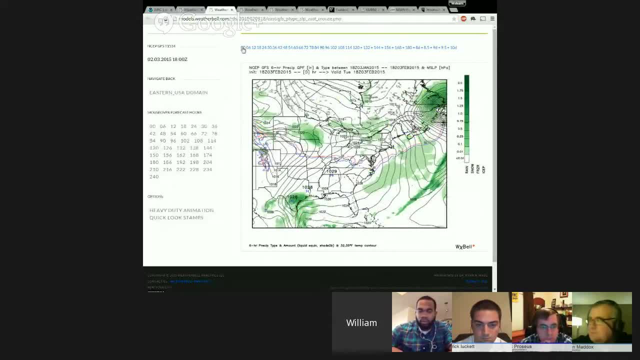 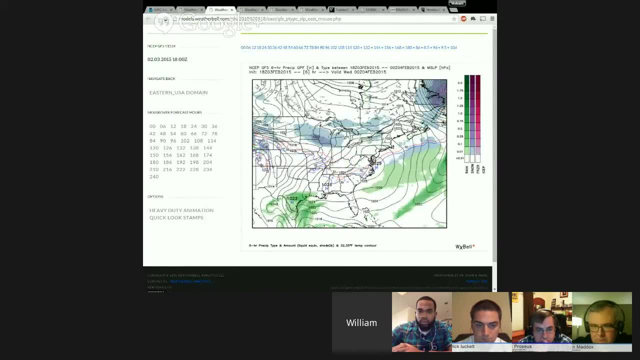 So, to kind of a easier picture to understand, we're looking at this surface here, And so currently we have a high pressure over this, with some cooler air, but slowly. that's going to bring in some warmer air up tomorrow, And this is the high pressure that's sliding in behind the trough. 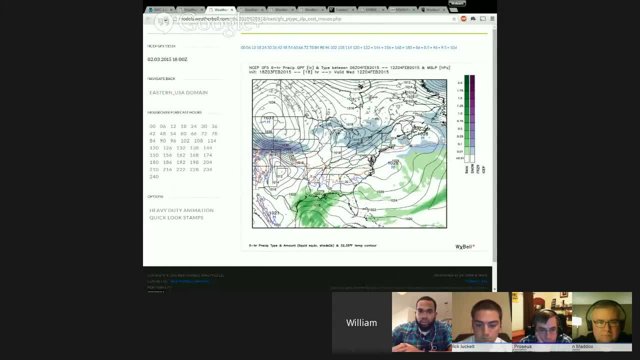 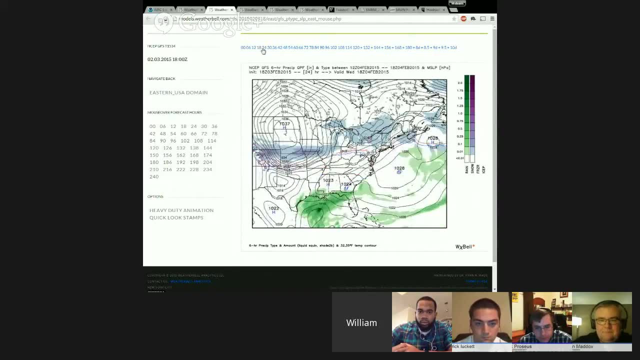 So this is the cold air, the source of the cold air, which is This is what we really need to get that potential precip to switch over to snow, hopefully, And this is one model just showing that this temperature gradient is strengthening. We call it frontogenesis. 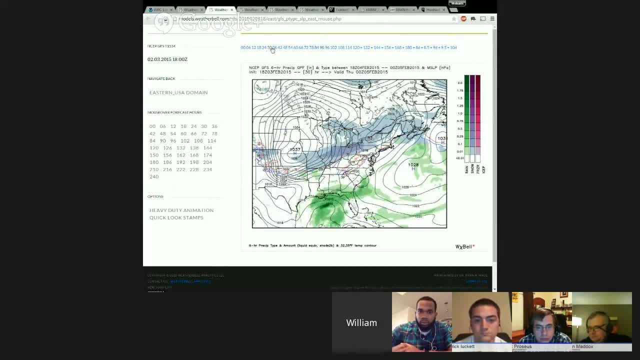 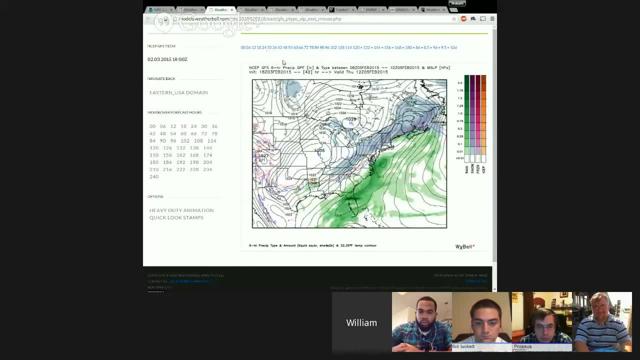 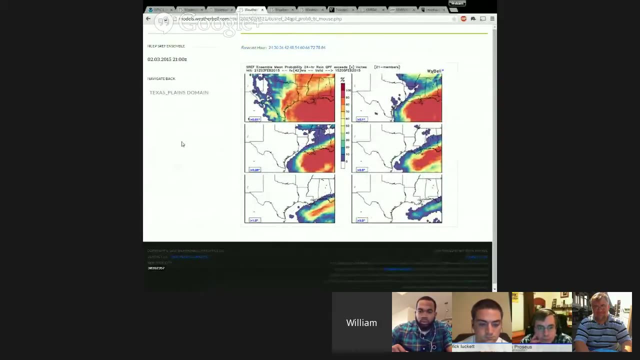 And as that gets closer, this particular model thinks we might get some snow. There's some actual blue over Memphis And as that comes through it'll dry out pretty quickly as we get into the day Thursday. So to give you an idea of one of the things we use to figure out if it's going to snow. 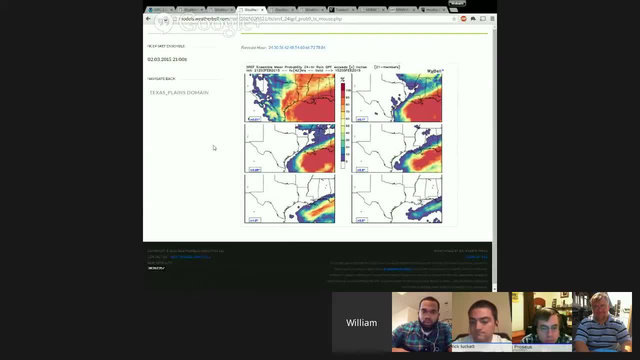 or not, this is an ensemble. This is a shorter range model than what we were just looking at, But the ensemble are basically just a model run, but slightly tweaking the initial conditions to get slightly different results. And so we run these a bunch of times and get tons and tons of results. 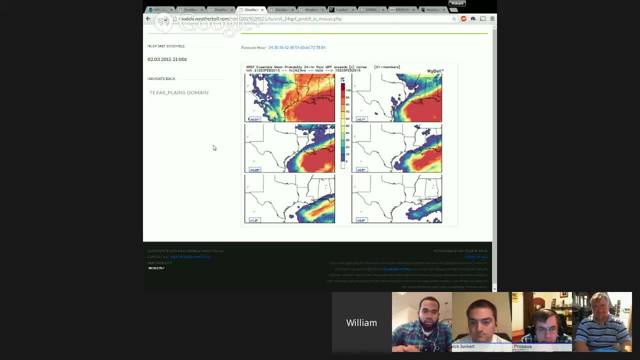 But then we can average them together to see kind of get probabilities of what's likely. So this map It's kind of hard to see. Memphis is kind of at the top here. but this is kind of the best I could do. 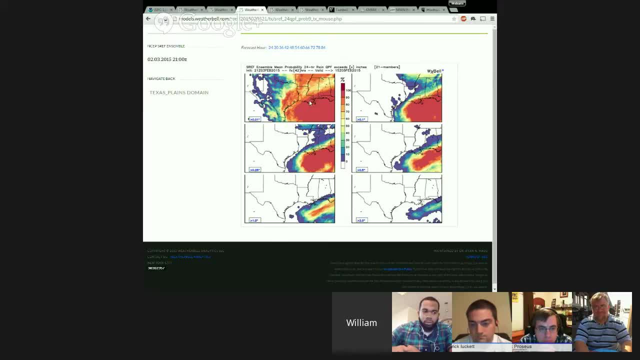 But this top left is just showing the percent chance that we get greater than a tenth of an inch, Or sorry, a hundredth of an inch, which is basically just any precip, which we're up in the 80th percentile. So basically this ensemble is saying there's an 80% chance that we get some sort of precipitation. 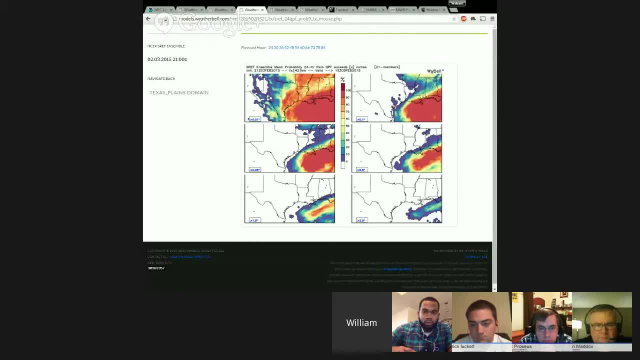 And as we move over here, we get to a tenth of an inch, which is about a 50% chance according to this ensemble. And then, as we get down to a quarter of an inch, we get a tenth of an inch, which is 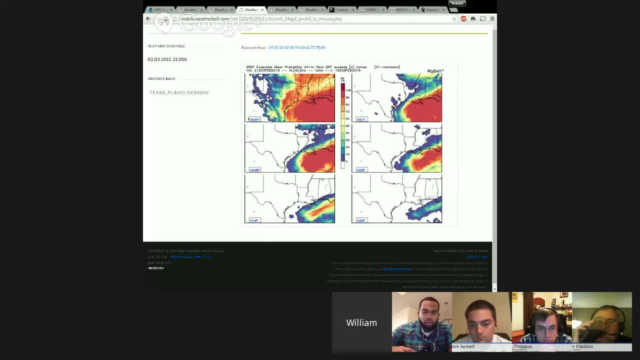 down to a quarter of an inch. We're down to about a 20% chance. So, and while those don't sound like a lot- and typically they're not a lot- when you have frozen precipitation in the form of snow, then that can really pile up. 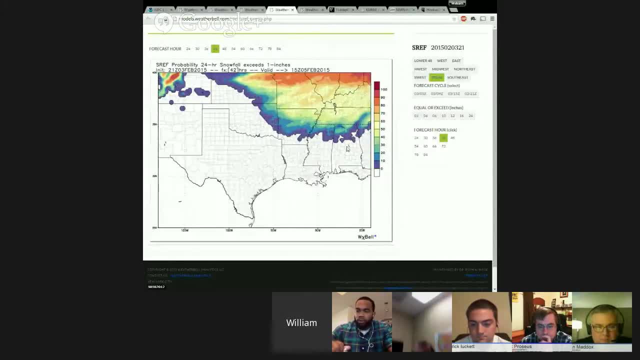 So this is specifically looking at snow instead of just rainfall. So this map is showing the potential to exceed one inch of snow and it's from that same ensemble And it has us closer to about 30% chance of exceeding an inch And I'd say that's. 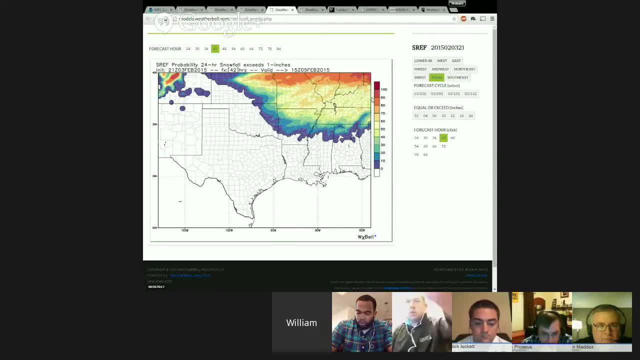 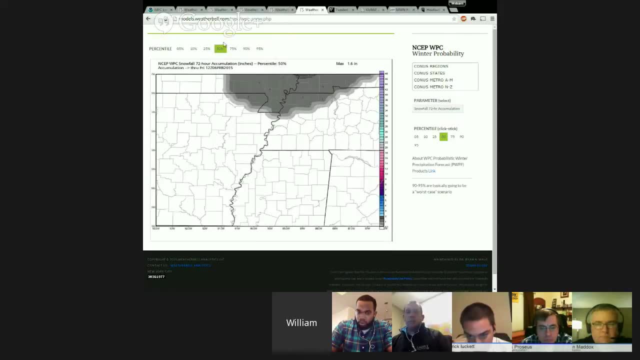 Probably fairly optimistic. even at 30% Looks like we might get a little accumulation but maybe not quite hope for an inch. And just like the maps I was showing earlier, they also have a percentile of chance of snow And they've kind of lowered their chances from earlier today. 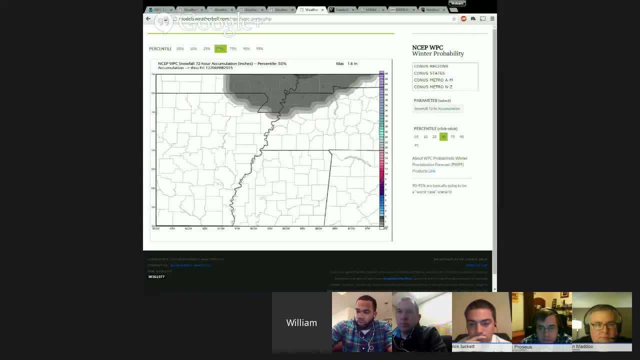 This is the 50th percentile, which basically just means this is the highest likelihood of happening according to the Weather Prediction Center, and they don't show us getting any snow. This is the 75th percentile, which would be less likely but still possible. 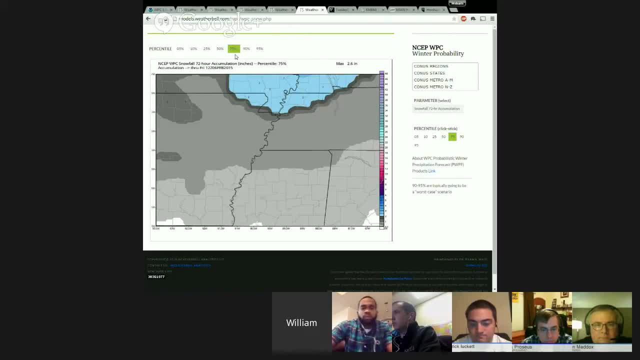 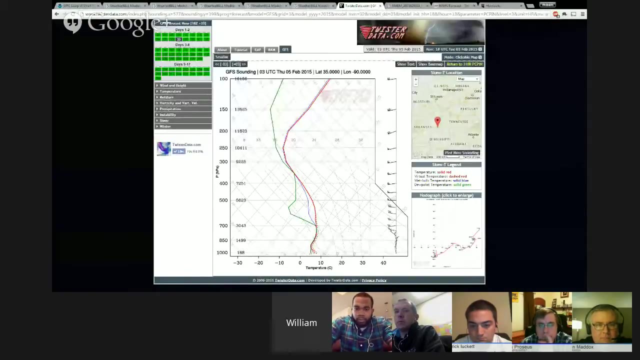 They show us getting closer to that dusting, or maybe up to even a half inch. So while possible, it's not super likely that we're gonna get accumulating snowfall. Map- Not sure how well you can see this. This shows the vertical profile of our atmosphere. 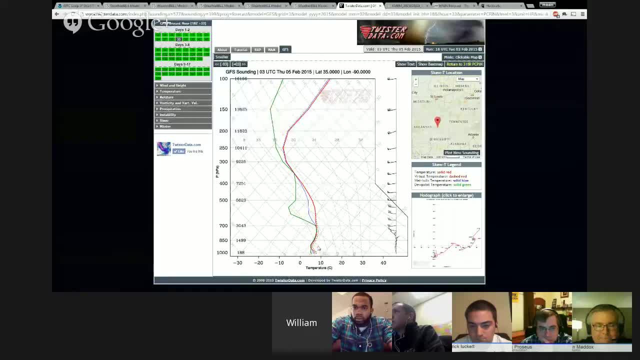 Okay, Okay, Mmm-hmm. Very interesting, Yeah, really Wonderful, Beautiful stuff. USA8 Thursday morning And this is kind of the transitionary period. so Kind of the problem we're gonna have here is, if this all was falling as snow then I'd. 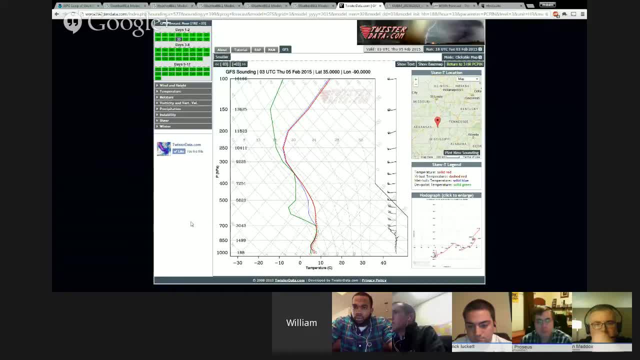 be more confident saying, yeah, we'll get a dusting, maybe even up to an inch, But the problem is it's more than likely going to start off as rain when it first gets in, so we have to wait till those cooler temperatures start effecting into lower levels of the atmosphere. 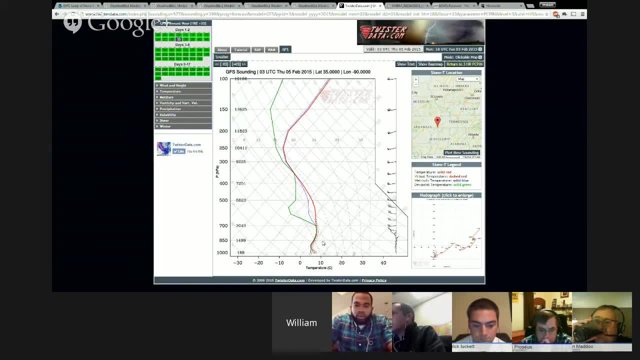 from the north, and by the time that happens, that's when our moisture's gonna start depleting. so Yeah, that's kind of how it usually happens in Memphis from that perspective. so, And just kind of on what one of the models shows, 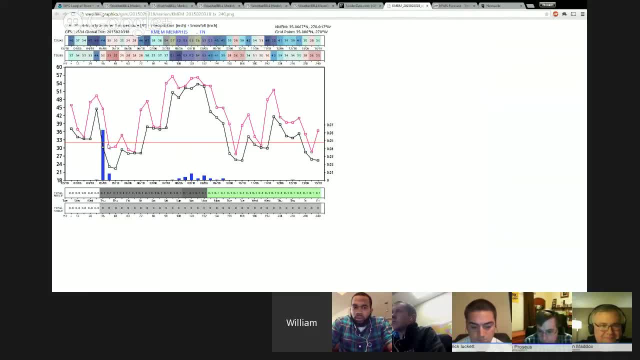 how our week looks like. So we'll be warming up tomorrow. then temps will drop pretty rapidly overnight as the rain comes in, Hopefully get a little bit of snow- That's what this is suggesting- And then by Sunday maybe up to 60 degrees. 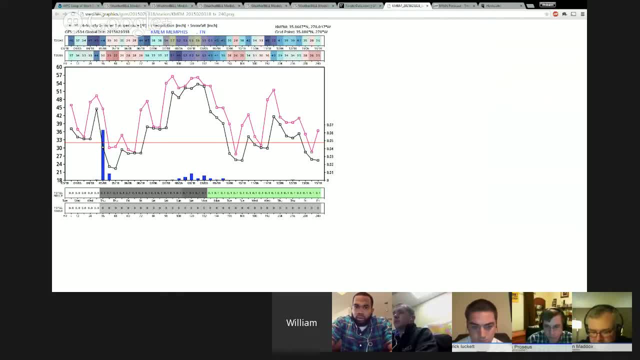 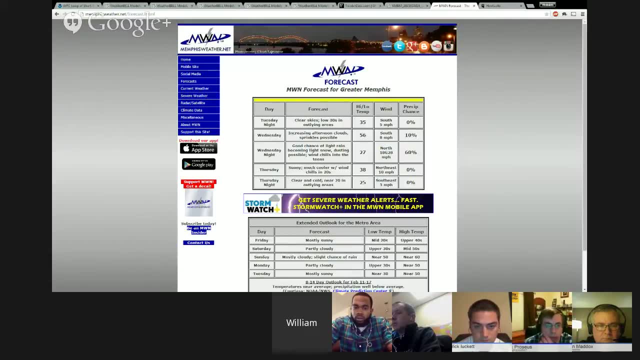 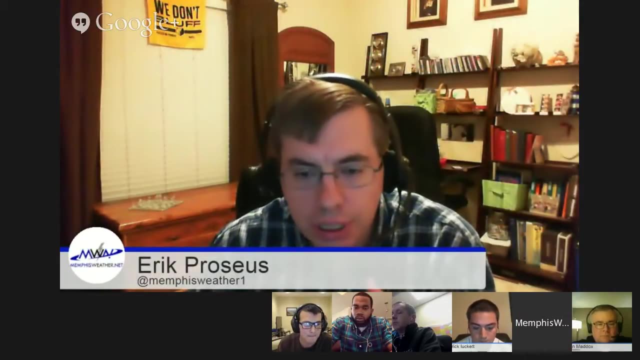 so it won't be too long before we're warming back up again. So not a crazy Arctic outbreak or anything. All right, And there's what we're looking at going forward. Let me whoops, were you still sharing that? Oh yeah. 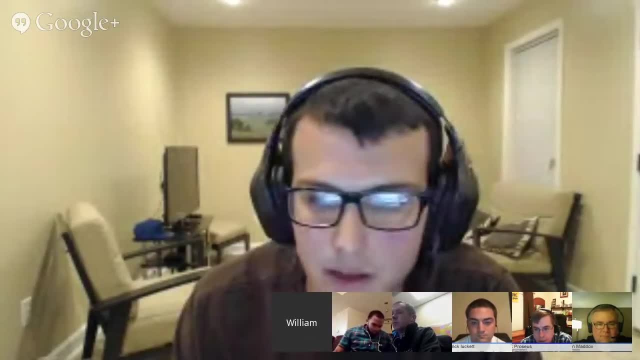 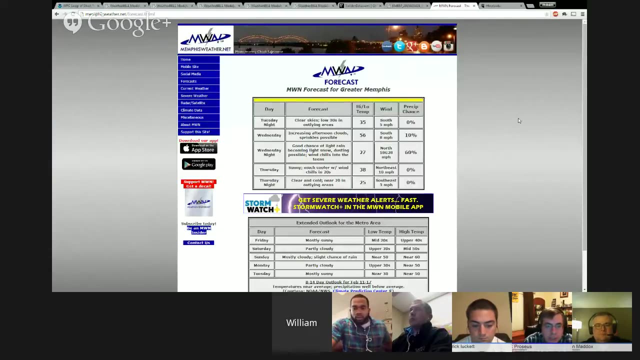 Do you want to go back to that one, Wayne? Yeah, let me see, And here's the forecast from us. Cool, so we are, and I'll share it here. So we are, on our forecast, calling for a slight chance of rain. by late tomorrow afternoon. A better chance during the evening hours. A 60% chance of precipitation tomorrow night And expecting that light rain could change over to light snow during the overnight hours. Probably around the midnight time frame is my best guess right now. 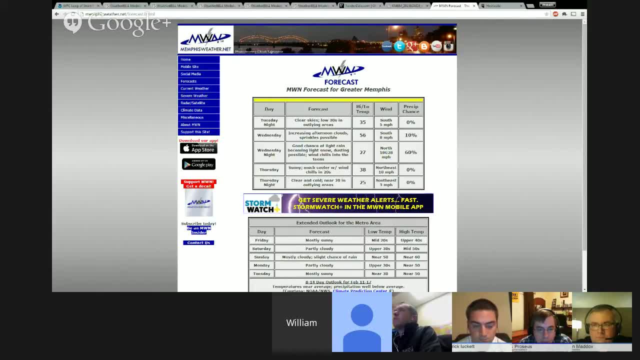 Midnight or within an hour or two of that, And then precip tailing off overnight Dusting possible. So that's, you know, up to a quarter of an inch or so, again mainly on grassy surfaces, Temperatures really bottoming out. tomorrow night, though, Down to 27, with a north wind up to 20 to 30 miles an hour. It's going to feel very, very cold at the bus stop Thursday morning. Another cold day Thursday, much like we had on Monday, And then we warm back up. 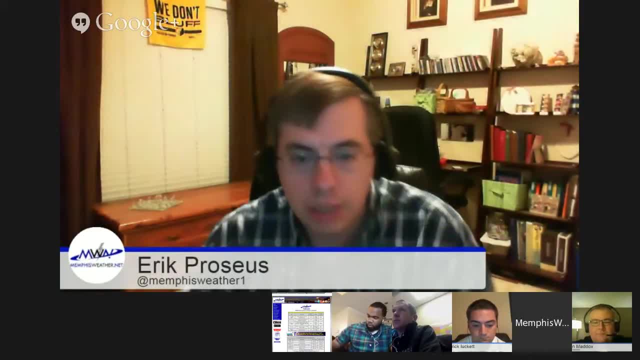 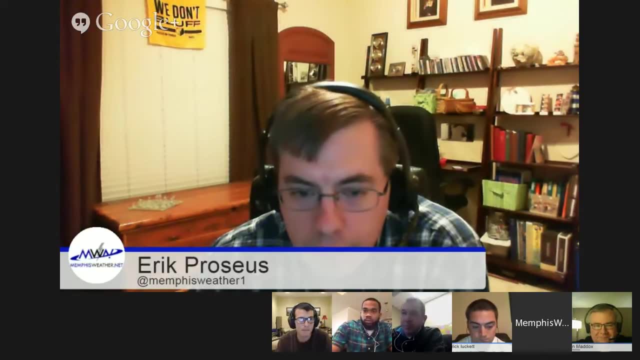 So that's a good overview. Thanks, William, for covering that, And I also want to welcome Ryan Vaughn to the broadcast tonight. And Ryan, I may have? I think I muted you manually And my mute button is grayed out. 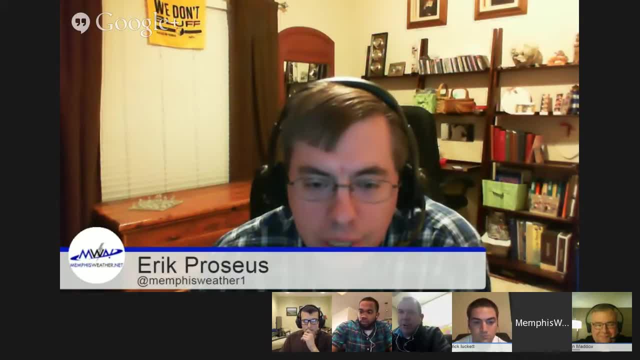 so I can't unmute you. So I don't know if you can control that from your controls or not. Can you hear me? Ah, yes, thank you. Welcome, Ryan. How's it going Very well? Thanks for joining us for a little bit tonight. 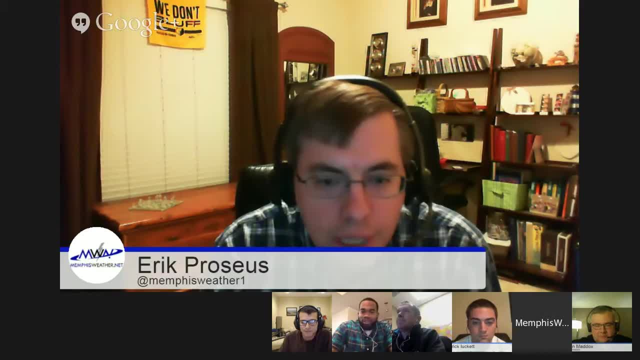 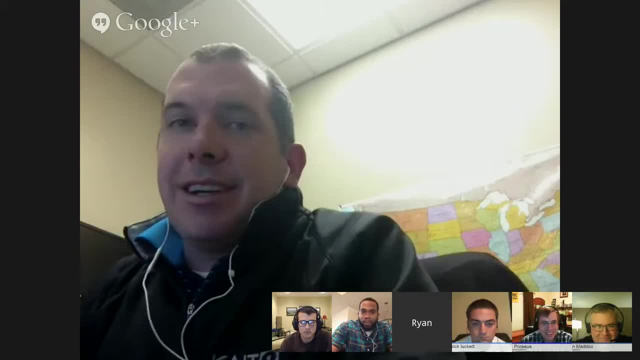 Ryan is from KAITTV And glad to have the media represented here tonight as well. Hope your basketball game went well. It was. It was actually practice. We need lots of practice. It's mold of sun. We had a slump last week. 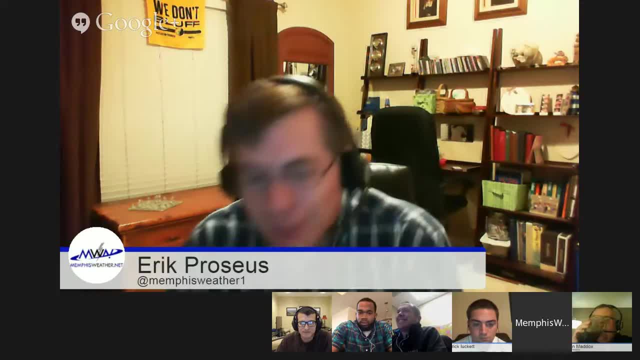 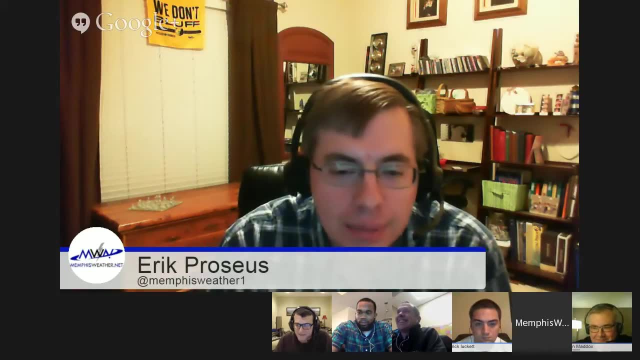 but I think they're getting back on track. Good Well, come down and practice with the Grizzlies for a while. Yeah, there you go. They'll teach them a little grit and grind Cool. So that's kind of what we're expecting. 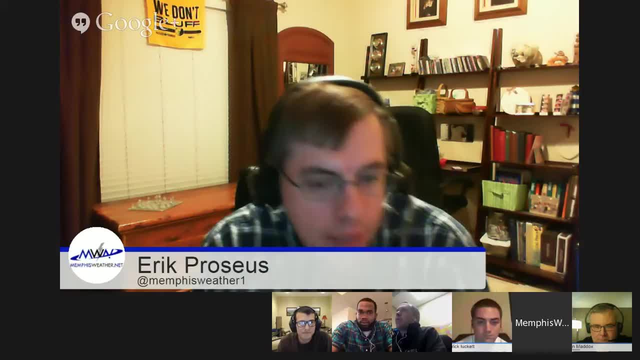 down here in this area. Ryan, do you want to go ahead and touch a little bit on what you're thinking up there in the Jonesboro area? Yeah, I'm going to go ahead and touch a little bit on what you're thinking up there in the Jonesboro area. 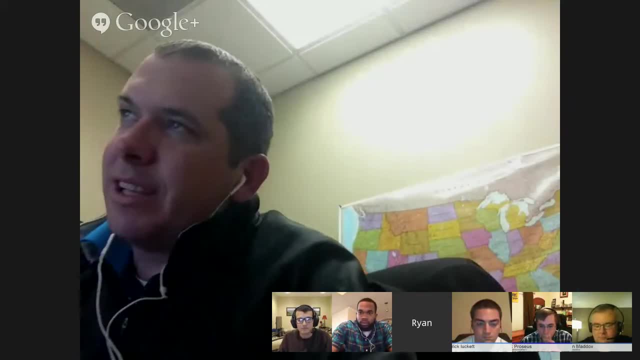 I'm going to go ahead and touch a little bit on what you're thinking up there in the Jonesboro area. Well, you know, I'm sitting here looking at Zero Z NAMM coming in right now, so I'm kind of multitasking. 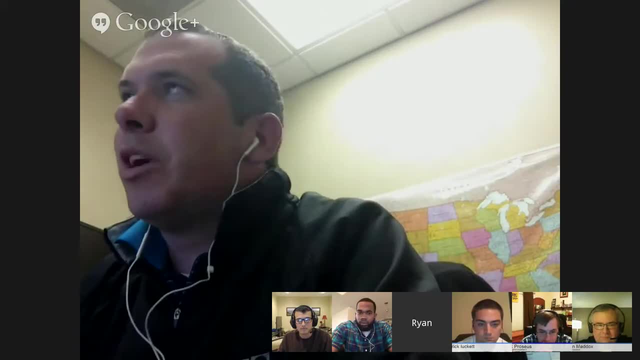 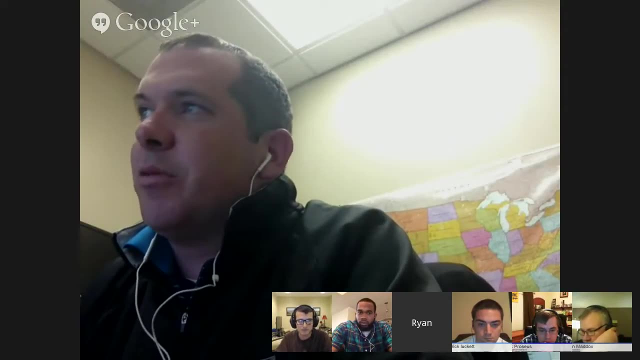 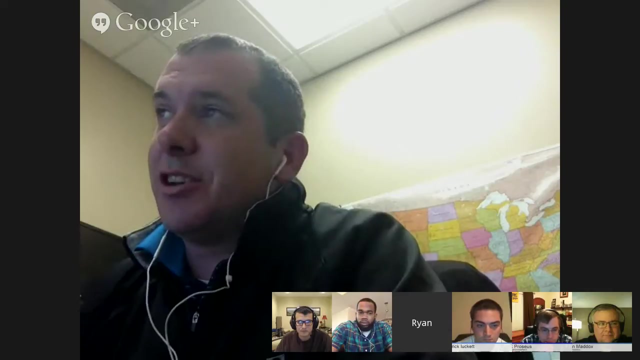 but boy, this is one of those moisture-starved systems and I'm just not overly impressed with it. I think we're going to stick with going with a dusting and possibly not everyone even getting that. I'm making sure the kids know. 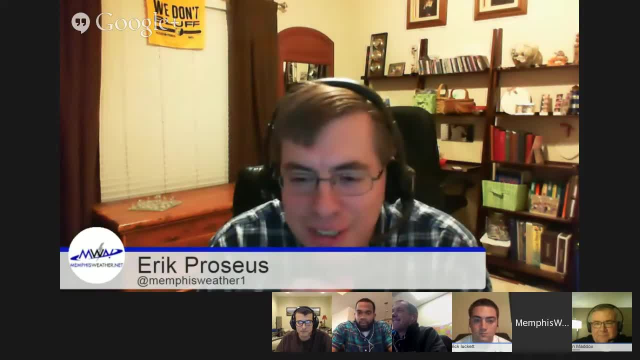 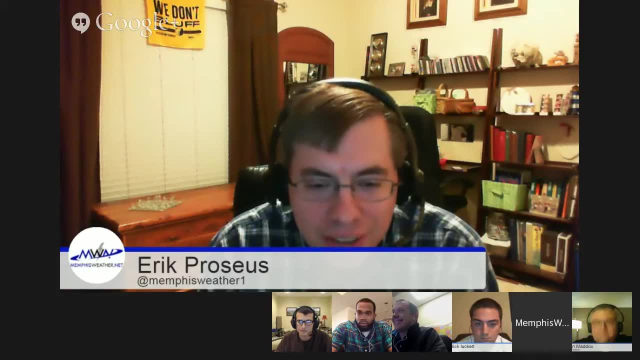 they're probably going to school on Thursday. Yeah, that's a good idea And unfortunately, that's what everybody wants to know is: do I need to do my homework on Wednesday night? And yes, down here in Memphis, kids do your homework. 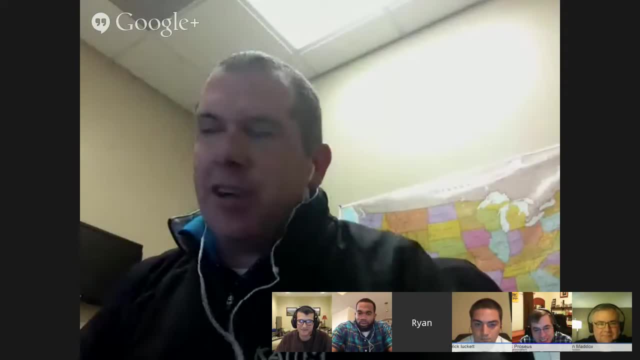 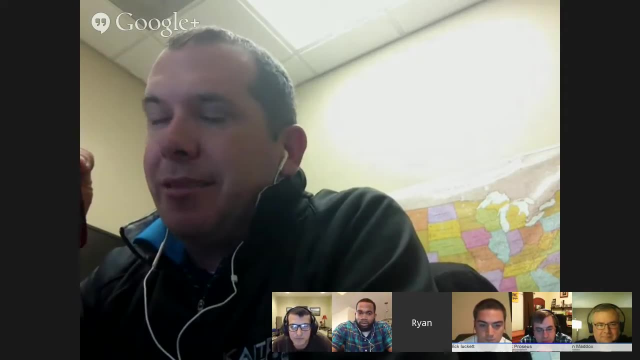 Do your homework. You know here. you know we were talking earlier about. you know, not only do we have to forecast, but we also have to impact forecast, meaning you know, will it stick to the roads? You know, I'm not a concrete engineer. 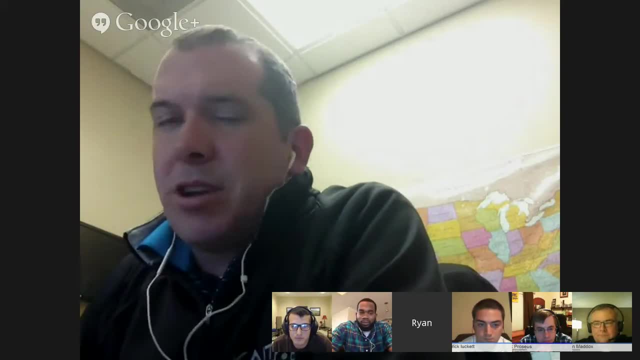 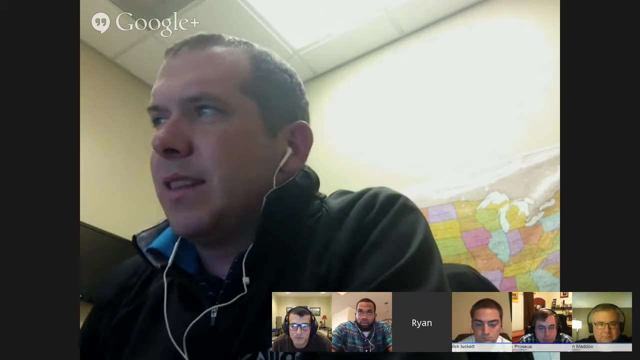 I'm not an asphalt engineer And so we were talking in the storm center this afternoon. you know we get up to 51 degrees tomorrow. Surface temperature, I think here at the station was about 42 degrees today. You know, will it stick tomorrow night to the roads? 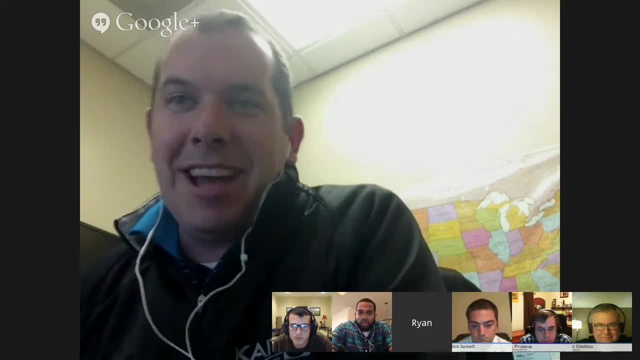 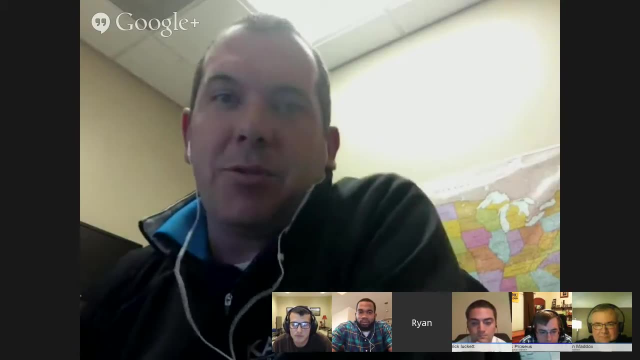 You know, that's always a toss-up As soon as you think, you know, no, there's no way. after hitting 51 degrees it'll just be on the grass, You know. then you get a street covered up and the superintendent's going, you know. 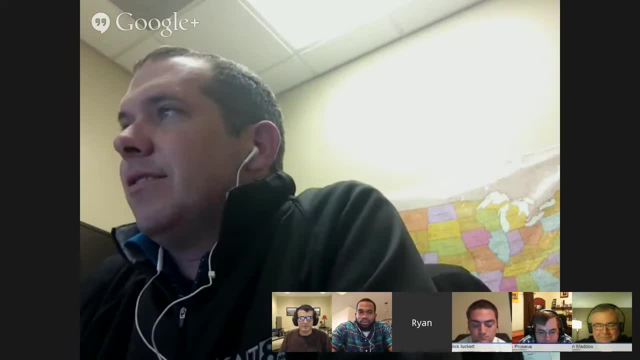 it's worse than what you said, even though it's a dusting. So you know we're going to have, we're going to try to prepare everybody for a dusting, but at the same time, a dusting can also. as you know, in this area cause some somewhat of an impact. Yeah, and I think down here as well. I mean, we've got a lot more elevated surfaces than you do as far as bridges and overpasses and that kind of thing. So even if we get mid-50s tomorrow, I mean those temperatures are going to drop like a rock tomorrow night, Yeah, very fast. So you know, I don't know if it's something that that, if we've got a little. especially even just a little water, water on the streets. if we drop to 27 by 6 am Thursday morning, do we end up with some icy spots on some of those bridges, And I guess I can't rule that out. 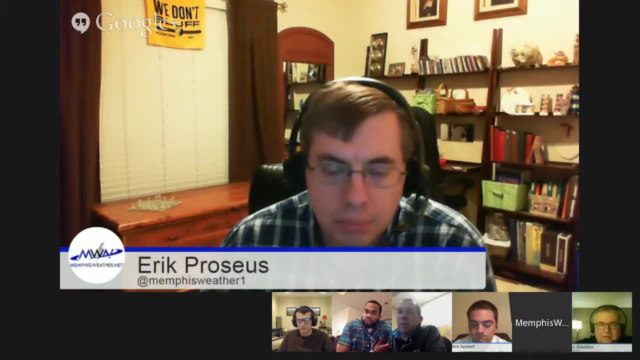 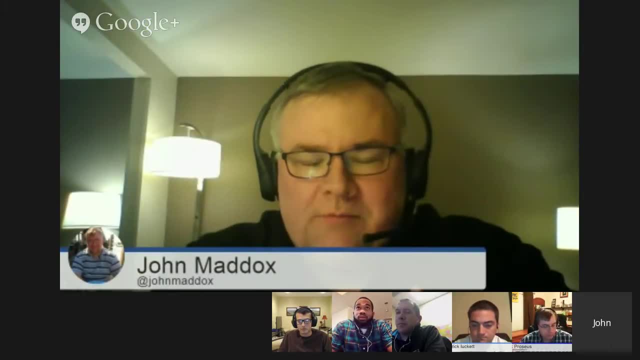 What do you guys- other guys- think? John, you've been around here a long time, both Johns. What do you guys think? Well, I think it's going to be tough to have road problems because of a couple things. Number one, as Ryan said, you know, 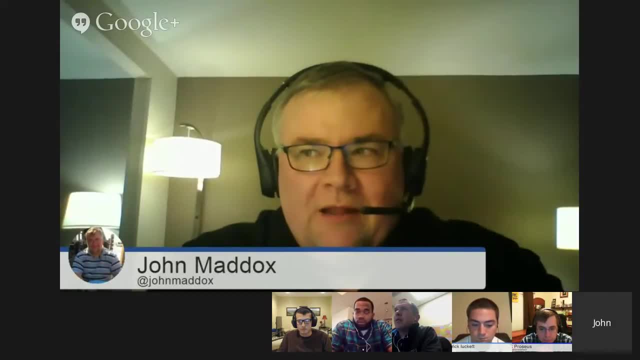 today on Twitter I made mention soil temperatures here and have been in the mid and upper 40s for the better part of the week, And that makes it difficult to stick. Number two: another blessing is we're going to have 20, 30 mile an hour winds coming in behind. So unless you get snowfall at a pretty good rate, it's not going to have time once it hits. even if it hits and doesn't doesn't melt, when it hits it's going to blow off the roads pretty quickly. So you know, but here we've got you know. 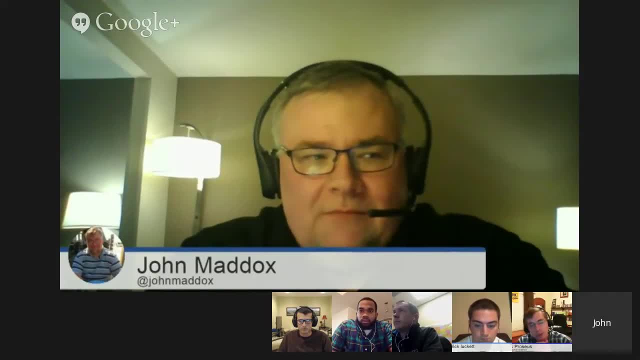 non-385, the ice rink that that is, and you know bridges and overpasses And it's like you said earlier. I slipped and slid a couple of times on my way to work This morning in Fayette County from the heavy frost. 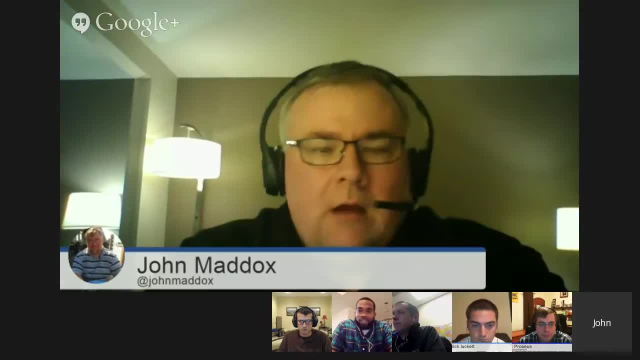 that was on some of the bridges. So you know, it's one of those things that it just doesn't take very much and it only takes one bridge to cause headaches. So you know, just give yourself wake up 15 minutes early Thursday morning. 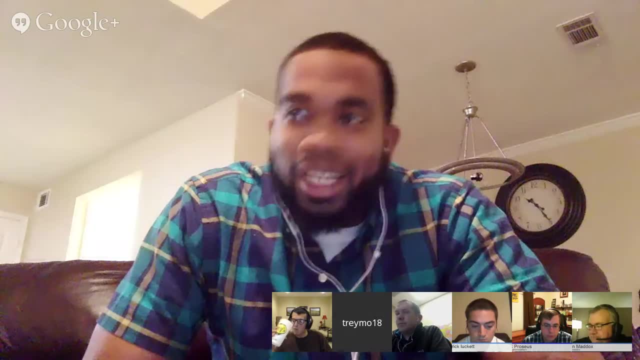 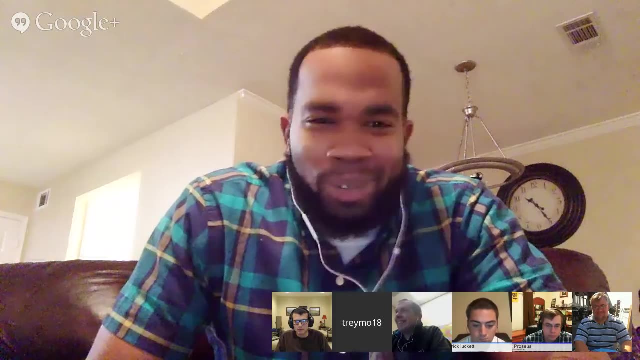 and be prepared to slow down when you cross a bridge. Yeah, exactly, And that's what we're trying to convey to the public, because even if you go back to November, when we had that light icing event and we had 50 accidents in Memphis- 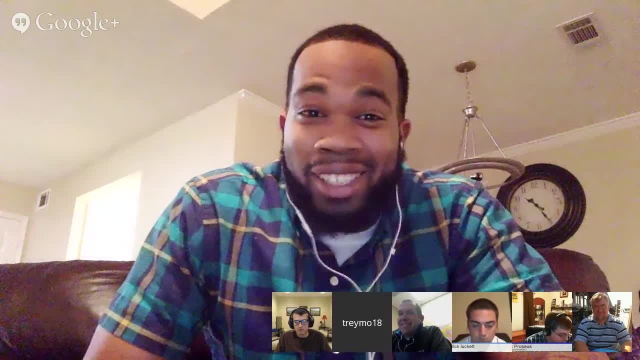 and we didn't have it in November the forecast. so we want to make sure we get that out this time, that hey, give yourself some time. yeah, that's one thing we did kind of hit on. we have this thing that we joke around with called the. 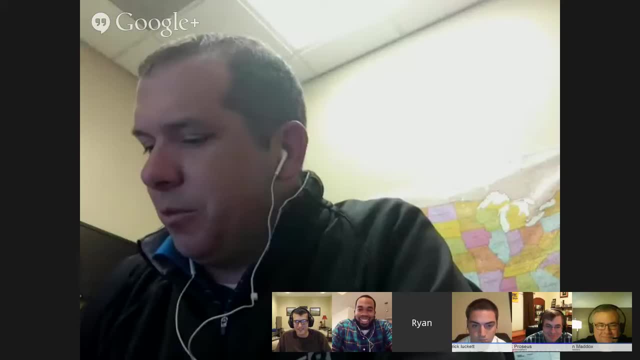 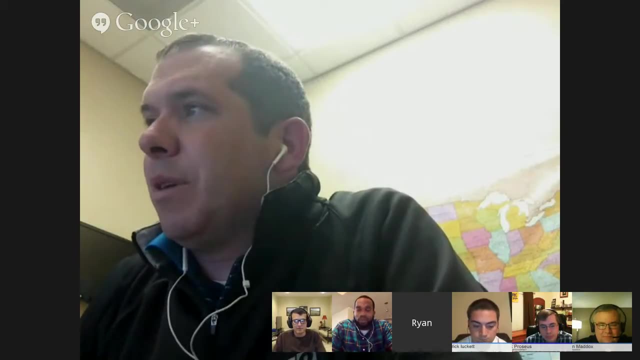 panicometer and uh, you know we have fun with it and you know it more or less gives people an idea of: okay, is this something I need to worry about or not worry about? we've just kind of been pushing a little bit that you know get up, you know five or ten minutes early. 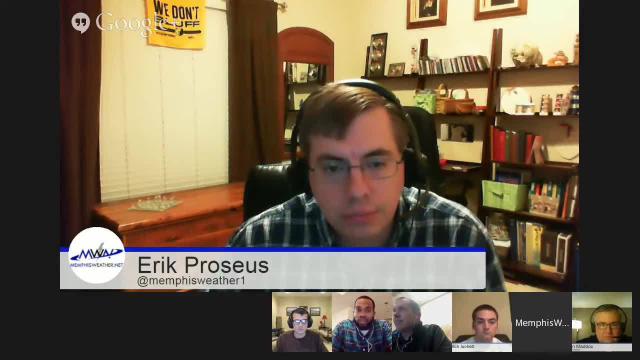 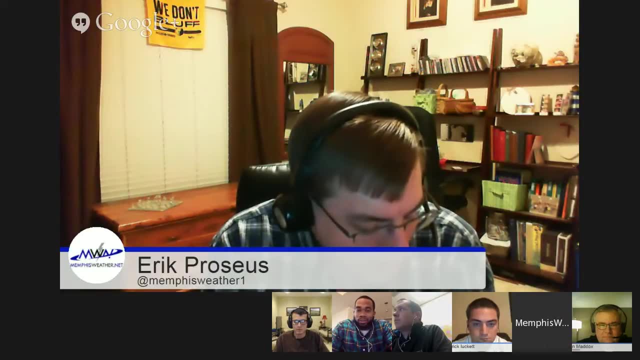 Thursday morning and make sure you don't need to leave five or ten minutes early- you know the weather wherever- makes me check the weather before you leave. yeah, yeah, that's. uh, that's something I think we'll get into a little bit later on, but there's, there's a there's an inclination. 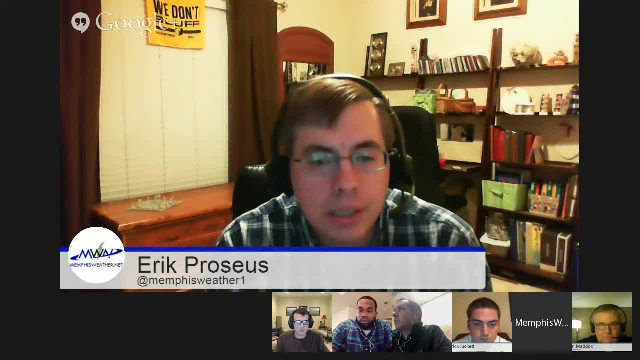 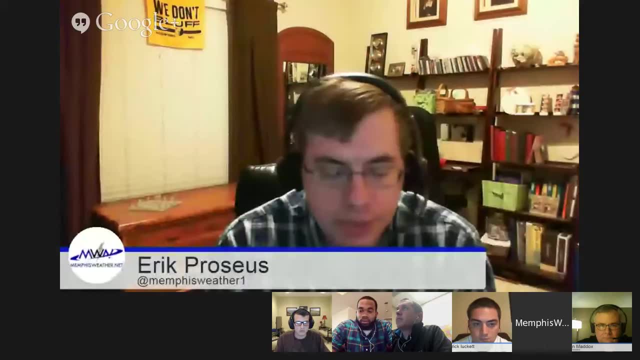 for people to- especially those that aren't as weather savvy as somebody maybe like John Maddox, is here with us or whatever to check the forecast. you know, say I looked at it yesterday and they're calling for snow tomorrow night, and kind of keep that in the back of. 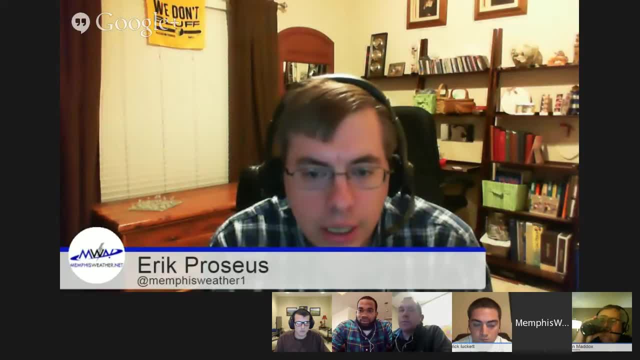 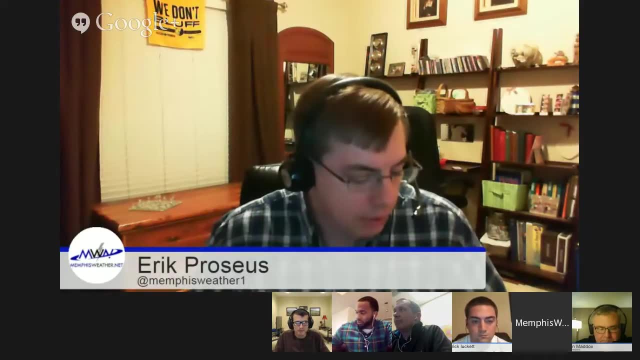 your mind and then and then not look again. and- and I think that's part of the consumer of weather's responsibility is to is to keep up with changes, and that's part of the forecasting, the uncertainty we we have a a job to communicate the best that we can in ways that the public 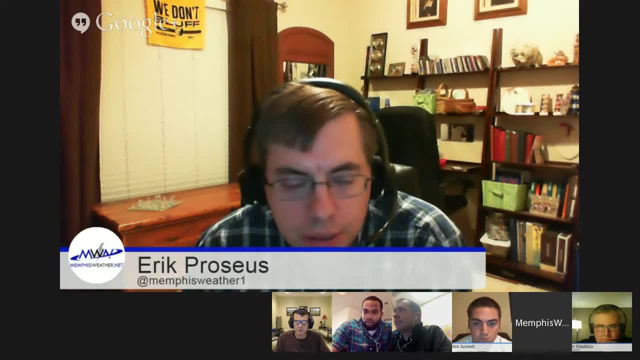 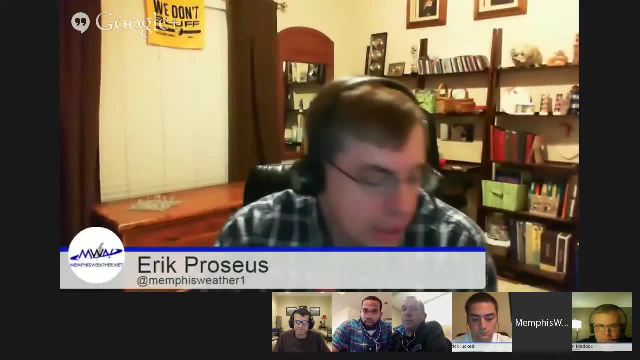 can understand. it's also incumbent on them to take that information and use it in in the ways that we're hopefully getting across. you know so well. we'll see. we'll see how things work out Thursday morning and you know I wouldn't be surprised to see a little bit of a. 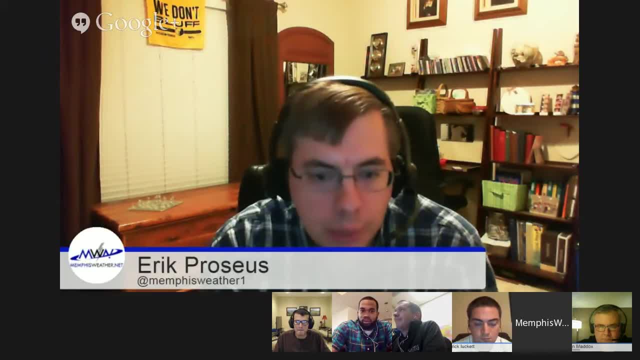 dusting on you know the little the mulch out in the front beds or whatever. it's probably going to settle between the grass and you won't see it. on the other hand, I wouldn't be shocked to see nothing when I wake up on Thursday morning. so give yourself a little extra. 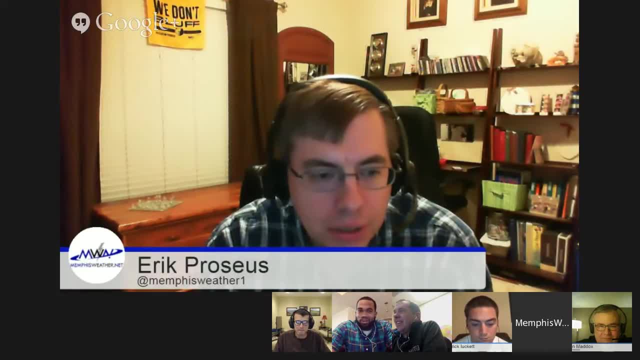 time we'll. we'll certainly keep you abreast, as we usually do here on MWN the weather service. follow them as well at NWS Memphis Facebook and Twitter, and up there Northeast Arkansas, Jonesboro, Ryan does a great job of that as well, so keep updated with the latest information. so I 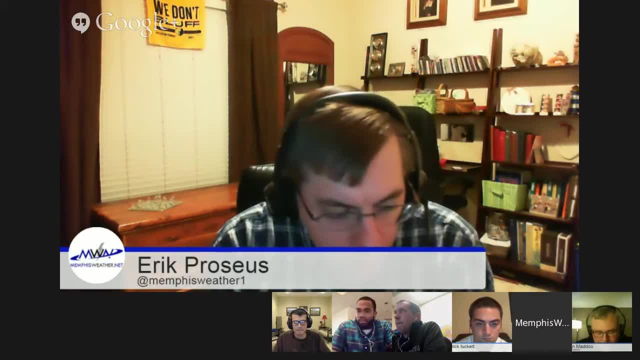 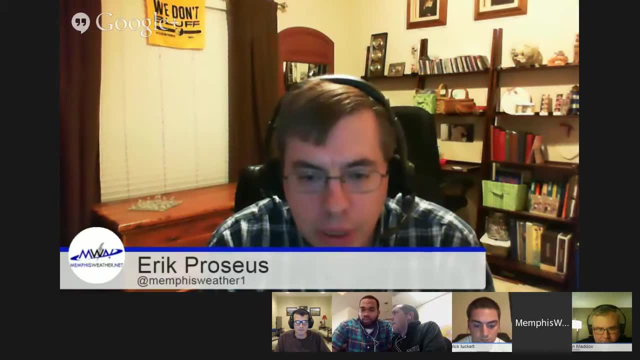 want to switch gears just a little bit. I wrote a blog last week and want to use that kind of as a basis for some discussion going forward with these guys, and I'm really glad that we've got kind of the- the public-private media all represented here, because this is this. 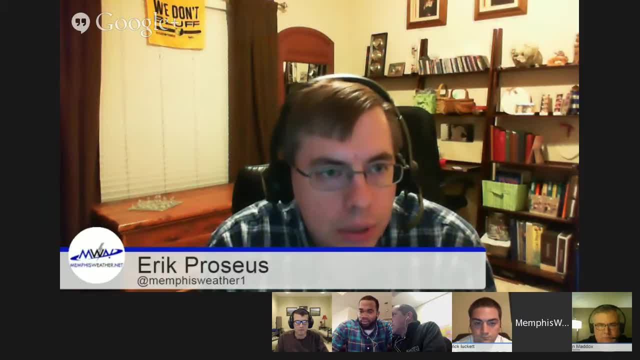 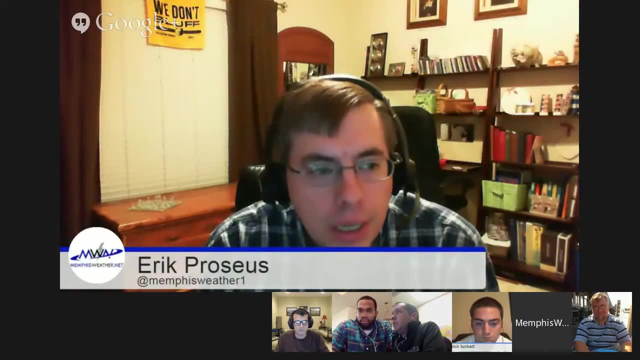 was kind of about what was. it was instigated by the blizzard, the first of a series of blizzards going through the northeastern US during this couple week period. but there was a call for a pretty big snowfall amounts in New York City back last Monday for the, I think was. 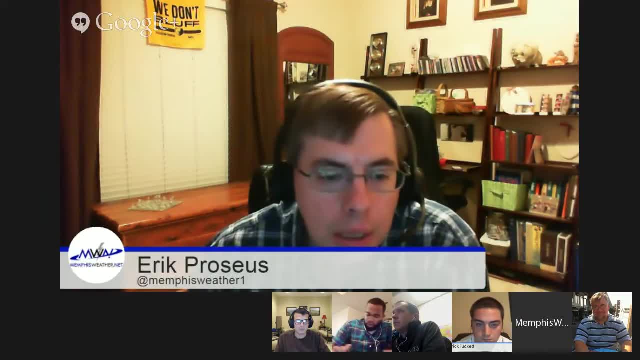 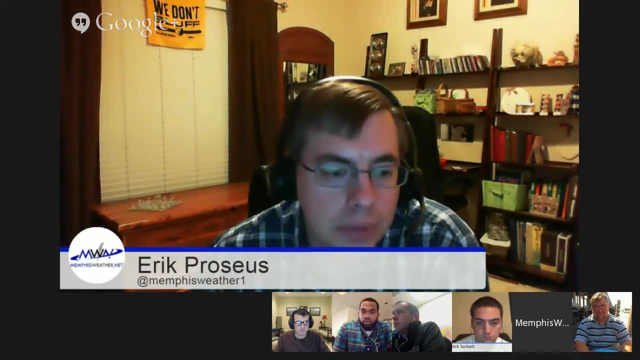 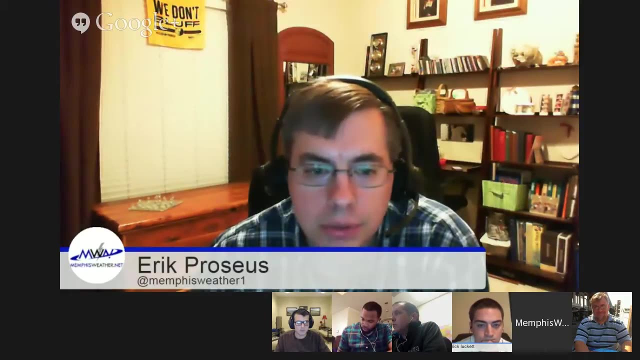 Monday night through Tuesday time frame and I want to, I want to see if I can share here some of the information that that we were looking at now. this doesn't pertain specifically to Memphis, obviously, but definitely was looking at it and in my, in my regular job, this was a. 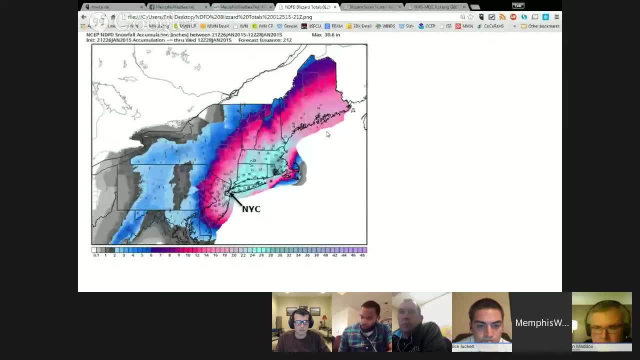 forecast we're putting together. so this was what the National Weather Service forecast for the Northeast Monday, Monday through early Wednesday, with New York City labeled there in the middle. so this is. this is the weather services to. NDFD is what it's called, but it's weather service data and basically, 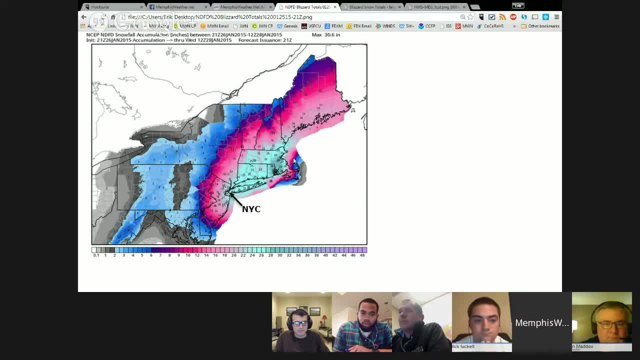 the Blues that are in here are up around two feet of snow and all the way back through New Jersey and up through the Hudson Valley and so forth, and in southeastern New York, amounts of about a foot and a half of snow. and this was, this was the forecast from Monday. 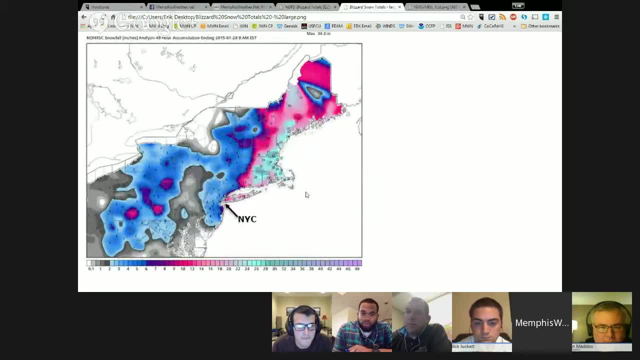 afternoon for that period. this is what they actually ended up getting, and so you see the the forecast and hit very, very well in the areas where it was more confident. over here from southern New England, Rhode Island, Connecticut, up through Boston- we saw a lot of pictures and video from Boston up into Maine Long. 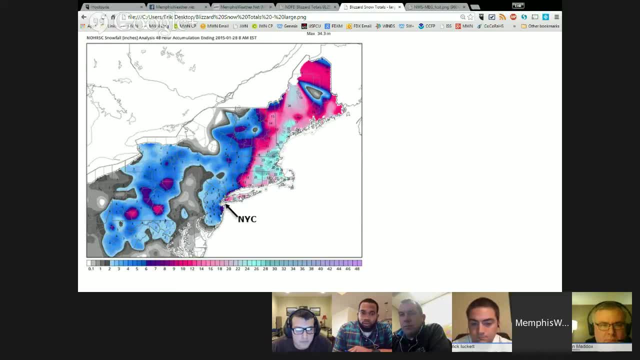 Island got hit really well. well or hard or whatever you want to call it, but they got anywhere from a foot to two feet of snow as well, depending on where you are, but the back edge of that very heavy snow was in the worst possible place as far as visibility is concerned. it's high. 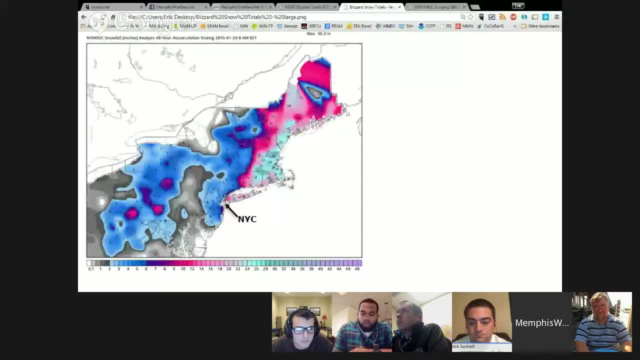 impact, high visibility, the media capital of the world, right over Manhattan and most of the totals in the New York City Metro were in these, somewhere from six to eight inch range, a little bit higher out to the east but you notice, you didn't have to go very. 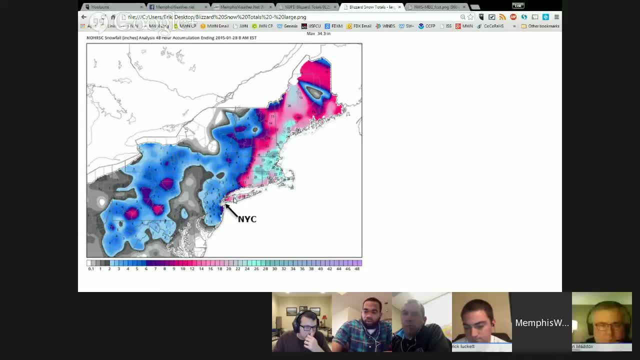 far out Long Island, you know 50, 60 miles or so, and there's a 22 inch reading just out down the street there. so you know, of course, with with this kind of event being forecast and and all of the all of the response that was initiated. 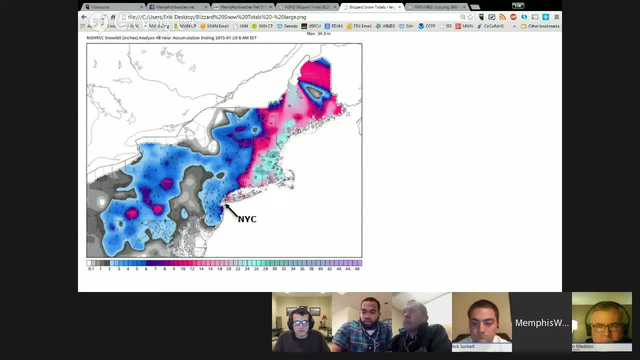 by the, you know, the local and state governments up there. they'd already been through a huge debacle with the Buffalo area lake effect snow earlier this year, where they weren't prepared for that and so they were no taking no chances. they shut down the subways, they got everybody. 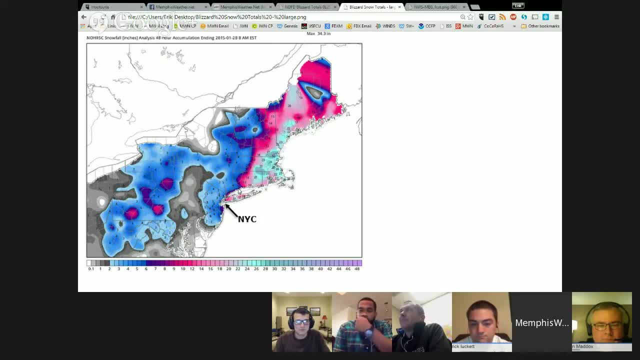 off the streets. they basically shut down the city and the next morning or Tuesday afternoon everybody's looking around going. we've got five inches of snow. we can handle this without any problem. so there was a lot of lot of discussion in the meteorological community on this. 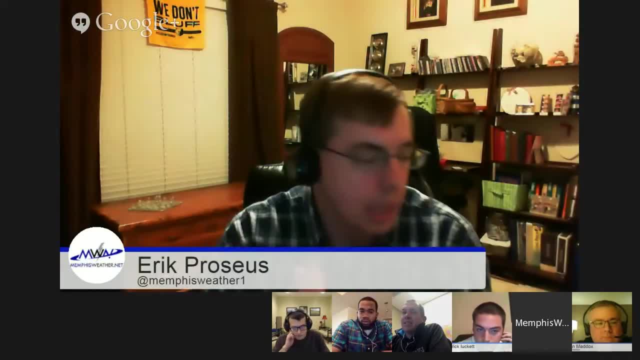 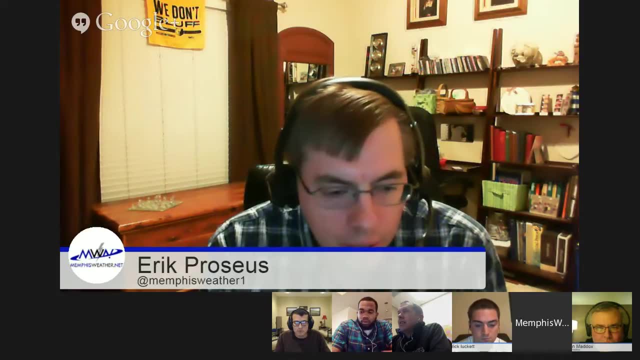 um, and a lot of different things that I read and decided to kind of put it into my own words in that blog, and the main thing that I think comes out of this is that, well, the forecast: yes, it was too high for the New York City area. 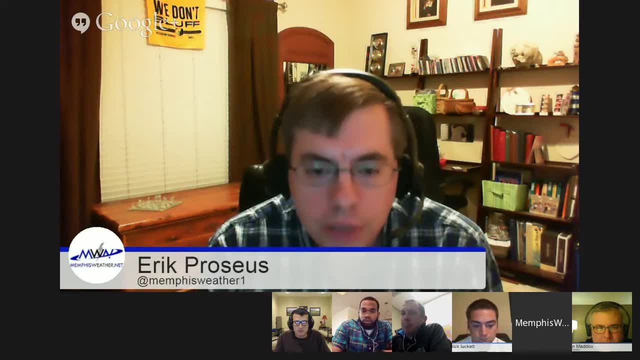 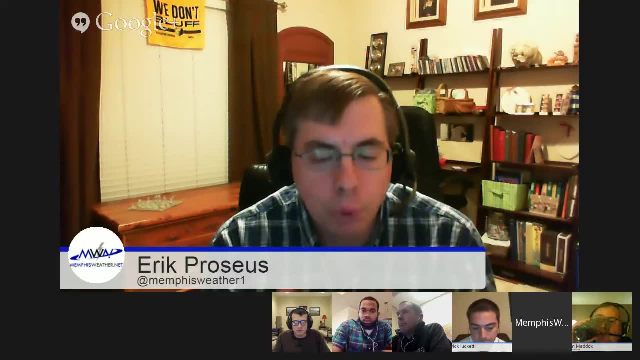 generally for the region. it was a really, really good forecast for a very high impact event. I mean, this is one of those world records are being broken. it's not very often that you're going to find people forecasting records to be broken, because it's just an outlier and I think 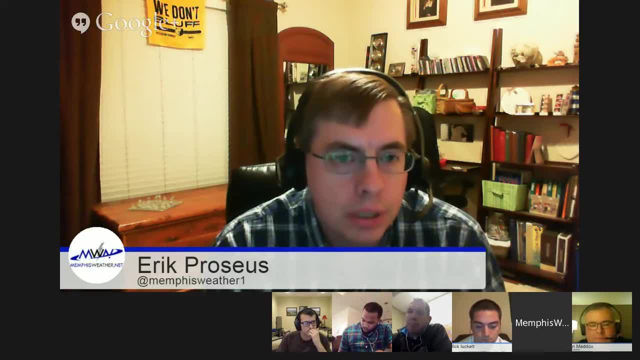 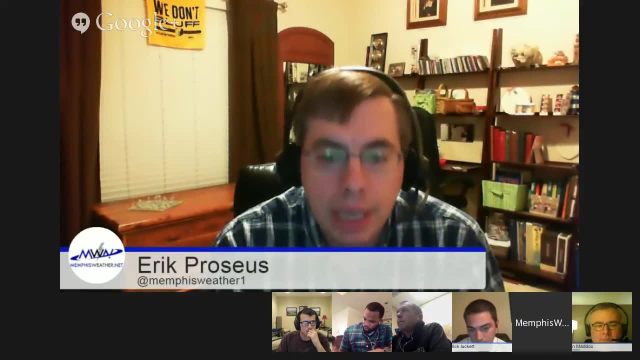 where the main issue came in, and this came up over and over again with others that are much more knowledgeable than me and bigger audiences, but it was all about forecasting the uncertainty and communicating that uncertainty, and so there's a lot of different ways we can do that, but I think that part of that is 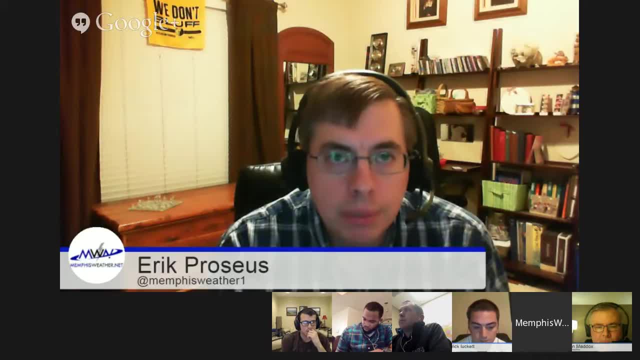 that you know, I think, what they got, what, what the Weather Service up there did, and then what the others that latched onto the Weather Service did was was kind of take that higher end probability event and run with it when actually there was a much higher probability of that being a bust in New. 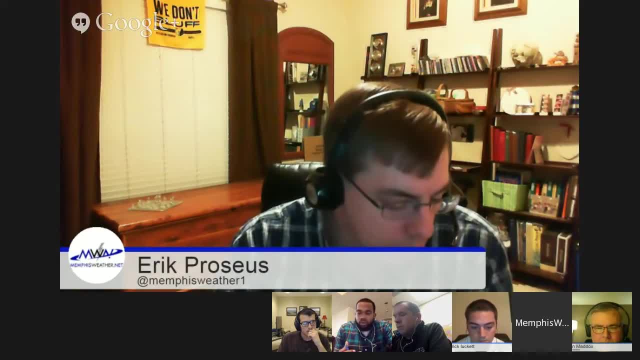 York City than there was in Boston, and I don't I'm not sure that that word was communicated well, now I'm not up there, but I followed it very closely, so like to touch a little bit then on. you know basically what? what is the? what is the? 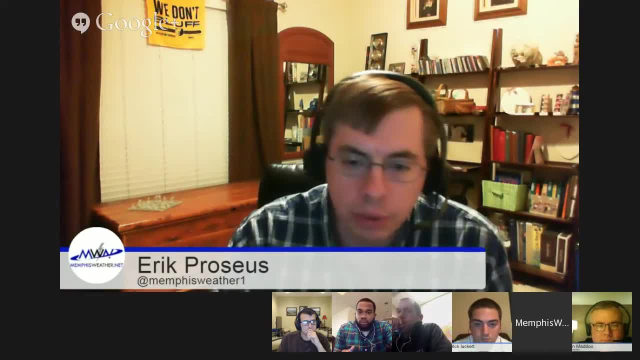 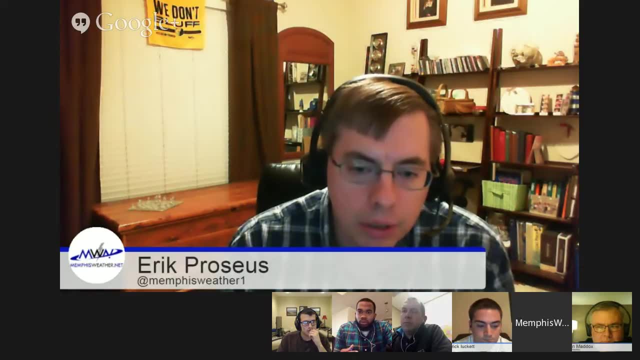 role of the weather person, whether it's on TV, whether it's the National Weather Service, whether it's a private entity like ourselves. what is our role in this and how do we communicate better with people in situations just like this? so I'll open the floor up and let you guys 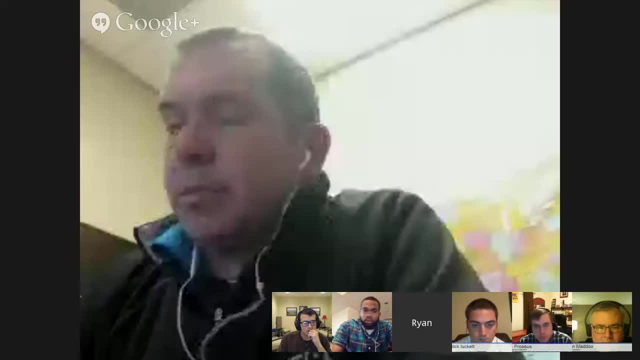 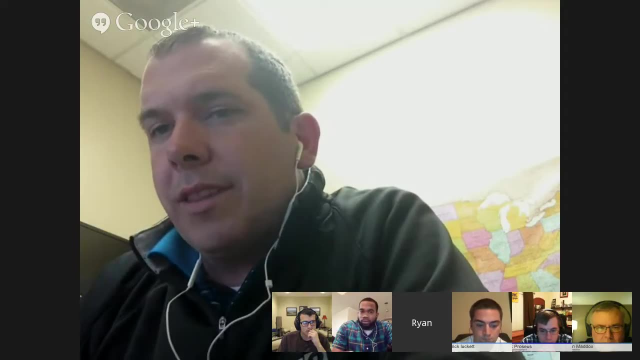 kind of comment. we'll just. we'll just talk about it. well, I've got about six minutes before I have to get a get to do in some some recording, but I'll throw this in. I think it's good to talk about what the uncertainties are, you know in. 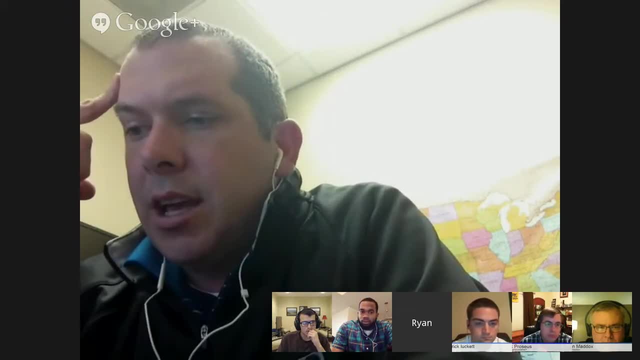 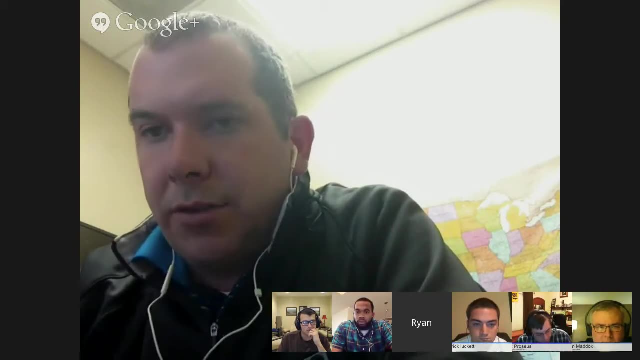 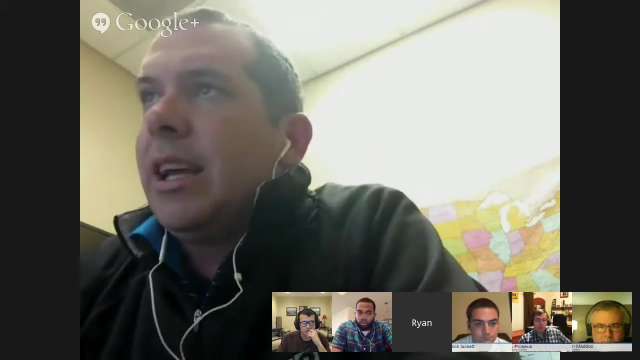 the in the situation last week in in the Northeast. we all knew that there was a very sharp cutoff and to put to convey that to the consumer, that there was a cut-off and that you know it easily could be east of New York City and I didn't watch any of them up. 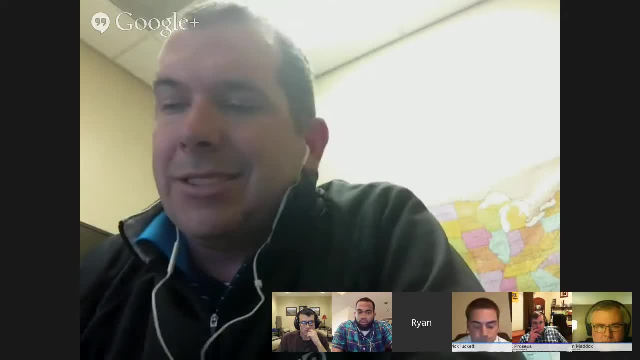 there, but I think that's important, kind of like this whole system tomorrow. of course you know apples and oranges, but I mean, when we're talking about the believes lack of moisture, you know what are the uncertainties of what the weather service but out of pretty cool graphic talking about. you know this is. 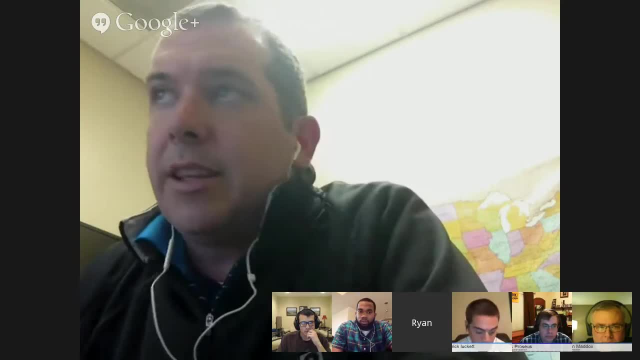 what. this is what we're thinking. if it's a little stronger, it's going to look like this, little weaker it's going to look like this. you know, I don't think there's any shame in saying the. there's some uncertainty, you know. i know some people think that that's being wishy-washy or. 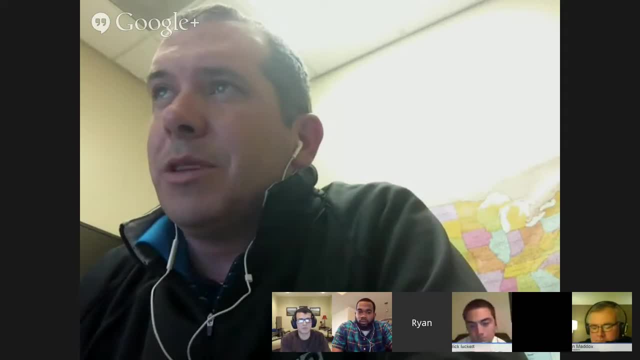 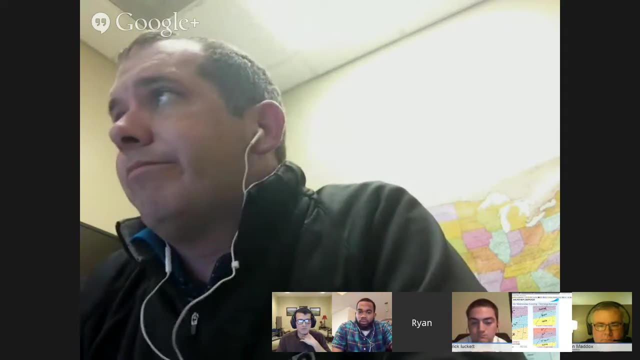 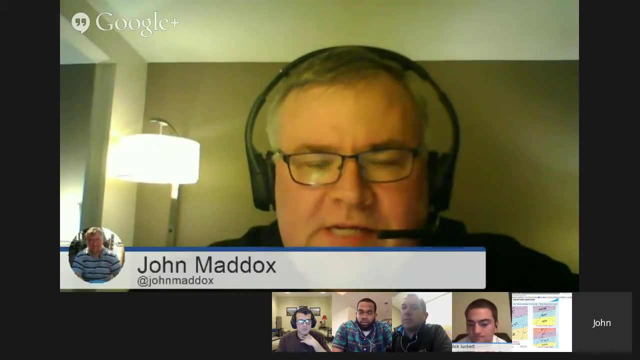 whatever, but, um, you know, also telling people and being honest with them and just saying, hey, um, it's not as cut and dry as what we, what we would hope it to be. um, that that's my two cents. i i think one thing, too, that that has to play into this is: and- and ryan, you can probably speak- 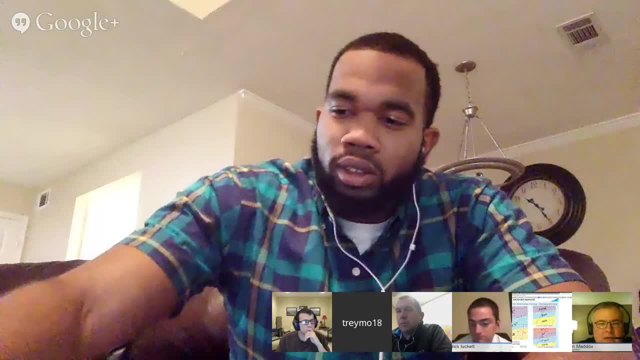 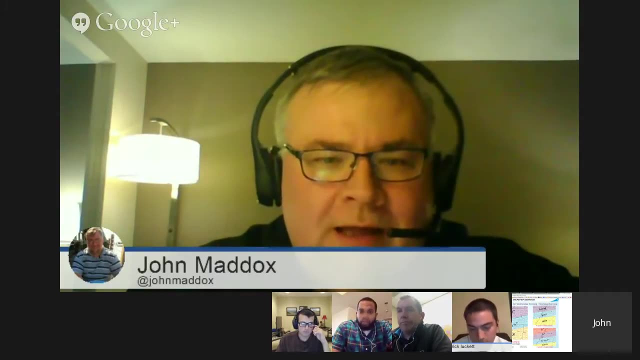 to this and, john, more you too, you guys, more so even, maybe even than eric. you have many different types of consumers to think about. ryan, you have a lot of agricultural interest. you know, john, you guys cover. you know you can't, you know it's real hard for somebody and say, well, how much is it? 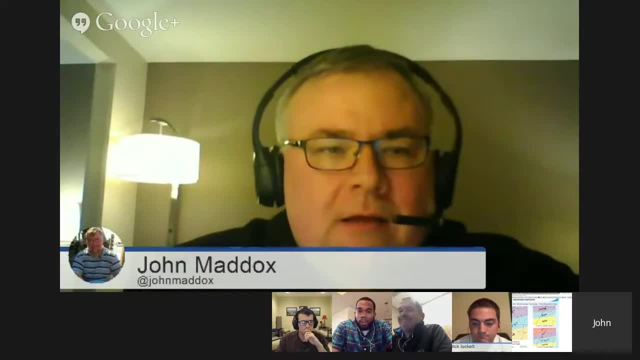 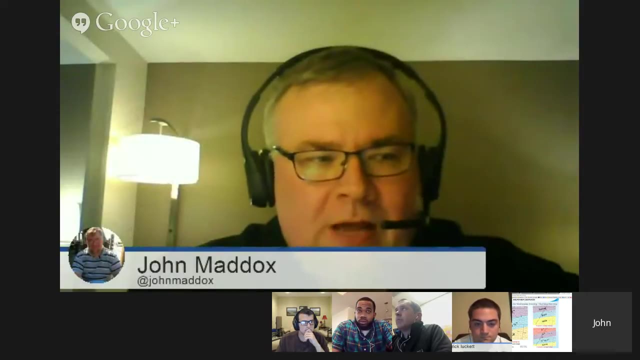 going to snow at my house for you guys, because you know you cover such a wide area and different consumer types take the information in differently, and i think that's one of the challenges in the weather community is how do i make it where you know eric and ryan and patrick and william and john? 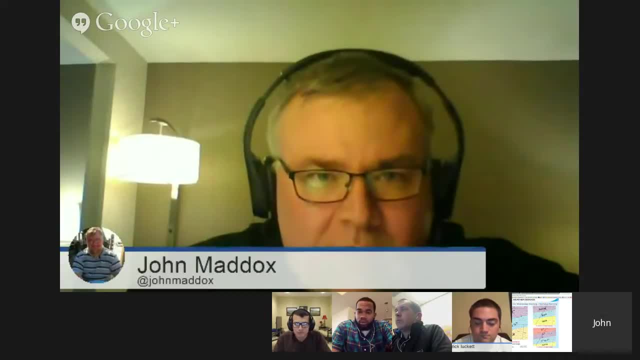 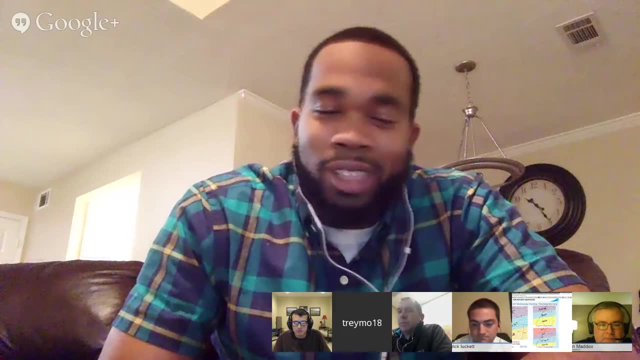 maddox can understand it and how my mother-in-law can understand it. i think that's one of the other challenges too. yes, that's, that's exactly right. john got a very interesting perspective on this because, when all this was going on, uh me and our new wcm, uh gary, uh woodall, we're actually 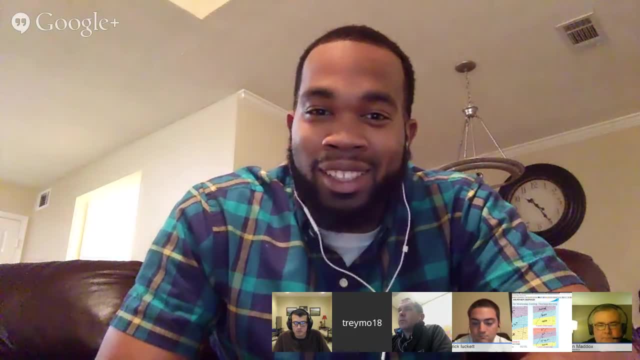 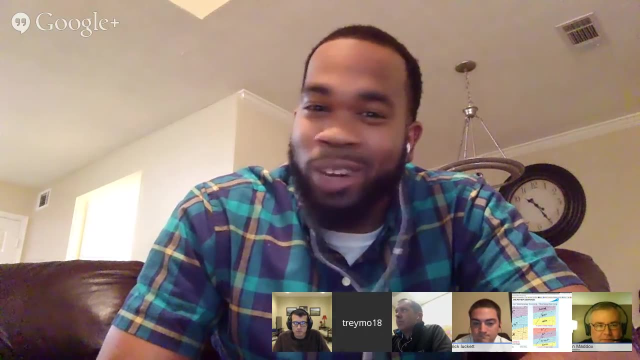 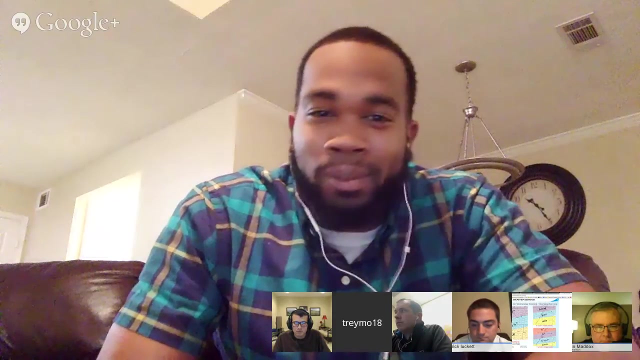 having a meeting uh at the mima headquarters down in jackson. so, yeah, we're watching uh cnn weather channel and they were telling us: hey, every time we want worst case scenario, we don't want any uncertainty, we don't want what it may be, we want the worst case. so as far as that partner goes, we have to kind of keep. 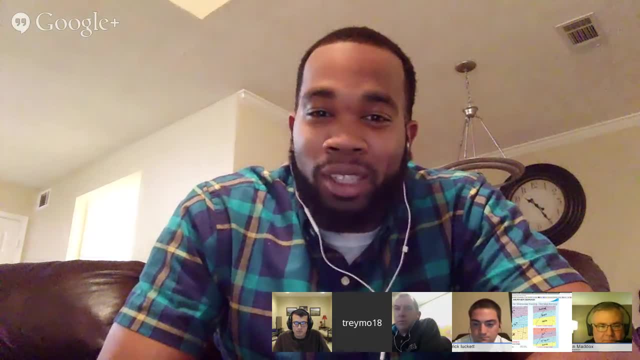 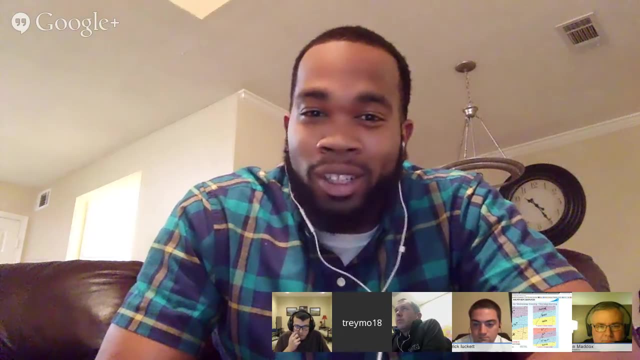 in mind that, hey, we gotta, they have to be prepared for it. so we always got to give them worst case scenario, that's mima. but hey, uh, the local, uh, the local guys, the shelby county, they want, they want confidence, tough factors and everything we do. they want to know how confident we are. most of the 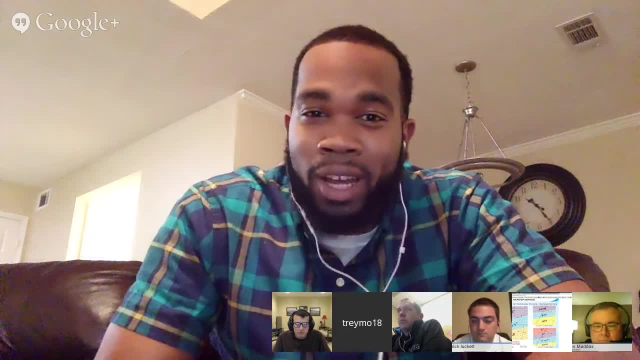 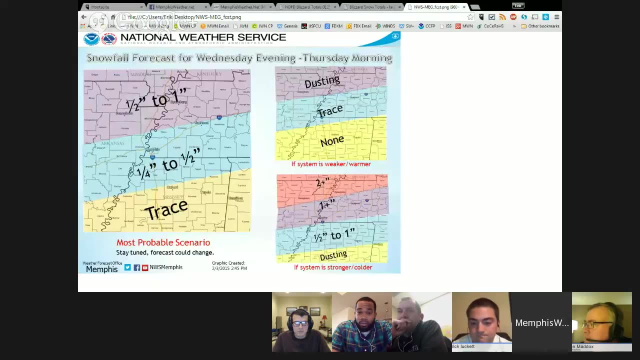 local school boards want to know how confident we are, so that's something we definitely have to keep in mind. john, i'm going to go ahead and share screen share this graphic here and i hopefully everybody is seeing that, but that's the one that uh ryan was talking about. it. do you want to uh speak to that? 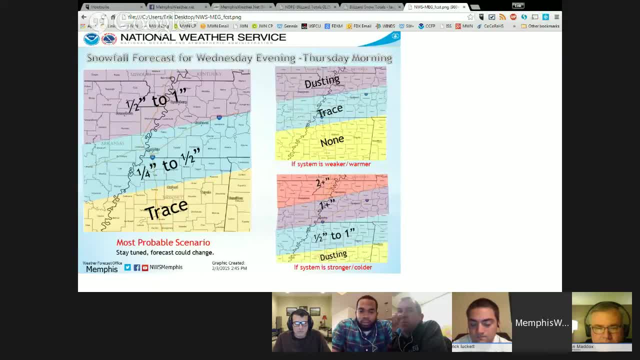 i know, ryan, you've got to leave here anytime, so i really appreciate you jumping in tonight whenever you got to go. just feel free, okay, thanks, yeah, good to be here. sorry i couldn't stick around longer. i will invite you. i'll stick around a couple more minutes. so okay, john, you want to? 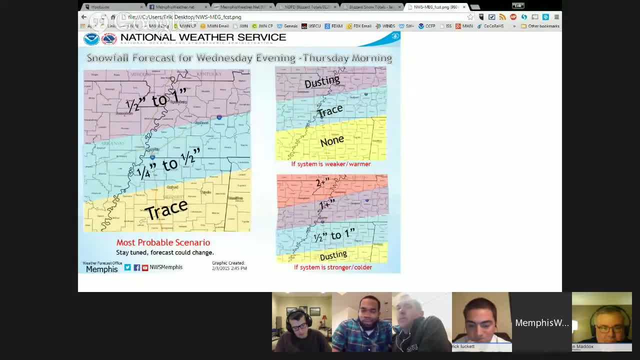 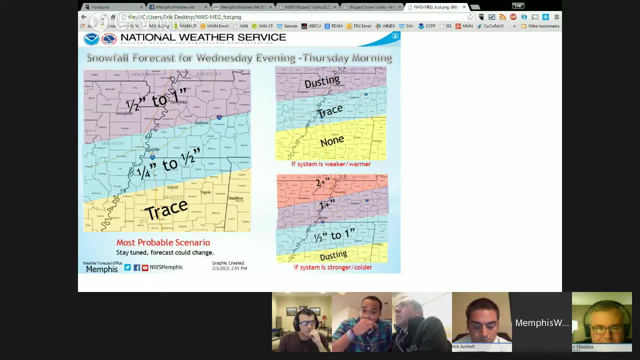 through all our social media products and any products that we put out. so, uh, this is a sample of what you're gonna see uh to come. this is a very small uh event, but we thought that we uh work on it beginning with this event. so they want us three scenarios each time to display our confidence. 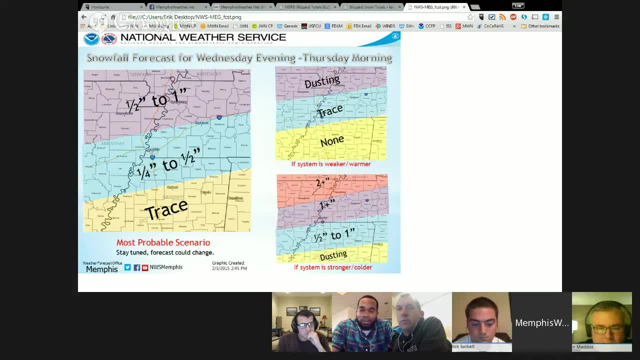 most probable scenario, uh, of most likely, like i said, most probable uh- an upper scale scenario and lower scale scenario. so we got to make sure we display each uh confidence level and try to explain why. as you can see, we couldn't explain really, because there's so much you can fit on a on a graphic like that. but yeah, sure that's. 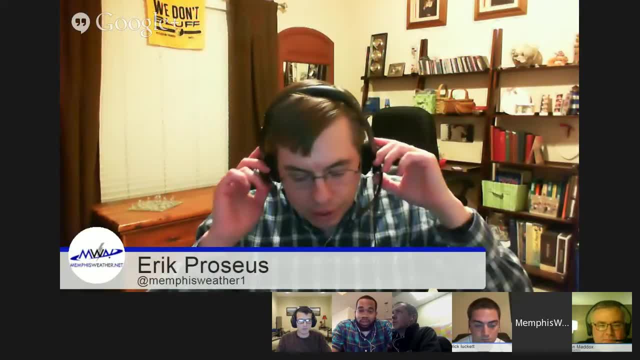 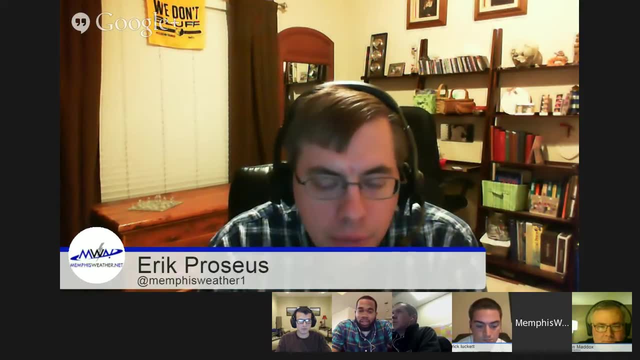 what they want. so that's. that's one of those that um. you know that that product is actually in experimental- i'll call it official experimental status um- at several weather service offices in northeast and they have a lot of information about what's going on and what's going on in the 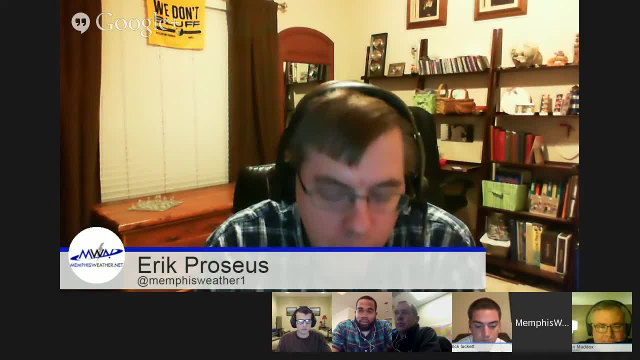 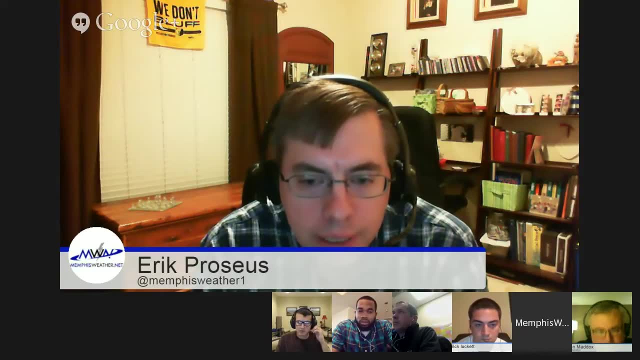 industrial area. so when you had that graphic available for that week, for that storm last week, i never saw it come across social media. it's buried in the website. you gotta kind of know where to go to find it. um, but that is. i mean, that's, that's really going towards i. you know i hesitate to say, well, that's perfect, but that is really going towards um, you know the direction that i think people need to know. if, if you are one of those like at um, at the emergency management agency, for instance, and you need to know, you know what is the upper end, what is what is the greatest threat you're going to face, is your brand that you're not able to handle, because when you're losing an order, you're losing kind of a lot of money. so you're gonna have an order delivery in order to actually get it done, and that can be a very difficult thing if you're going to be a leader of an organization or a company or a company itself. but that's the only thing that's really important to see and that's what's going to happen, and you know it's really important to see. 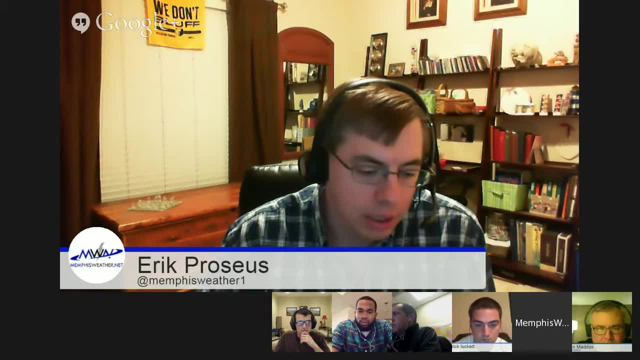 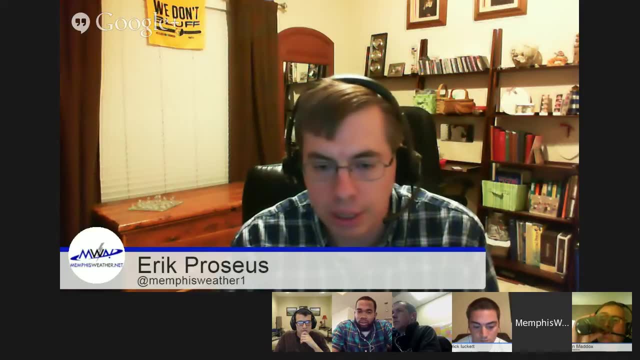 we could face here. that gives that picture. if you are, um, you know, a school superintendent, you want to see. well, what's our range of possibilities here? you know, this is what we expect, but it could be this. it could be this at least they know when they wake up that morning to take their first. 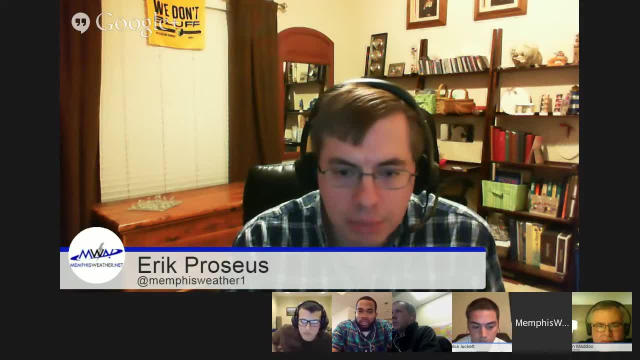 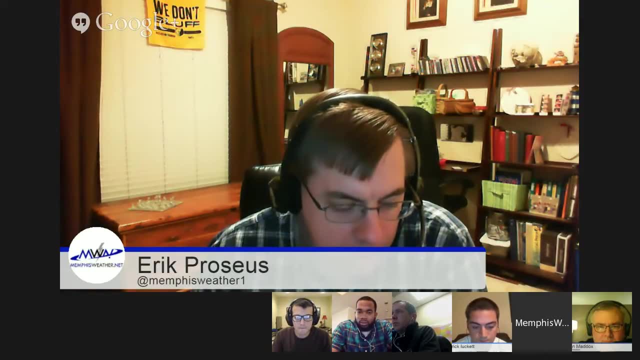 glimpse out the window and see what the roads look like. they know generally what they might be looking for exactly. so, uh, really really nicely done on that and and i i took that to heart uh, last week when i saw the, the discussions, that, and started looking at those weather service. 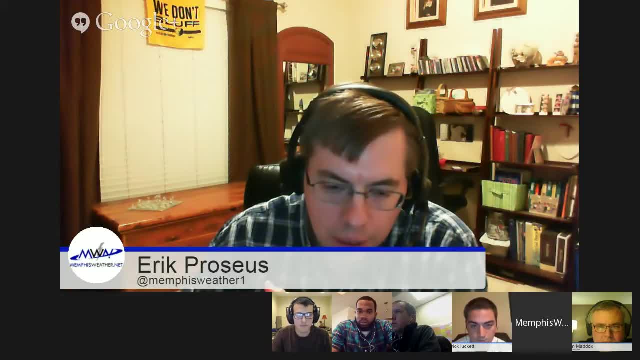 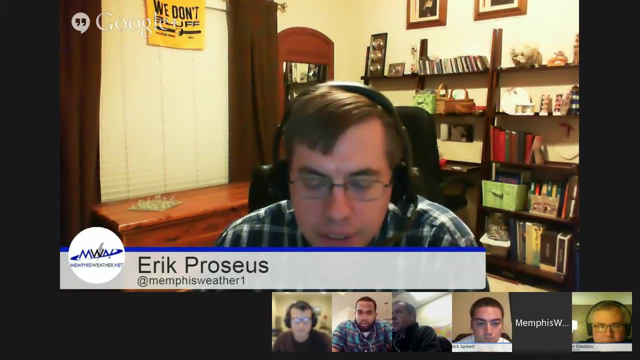 graphics, um, and you know, included that in our blog for for tomorrow night as well, that we, uh that i wrote yesterday is, you know, basically, what is the boom and what is the bust. uh, if, if this the total system totally busts, are we still going to get an inch of snow, or is it nothing? and in this, 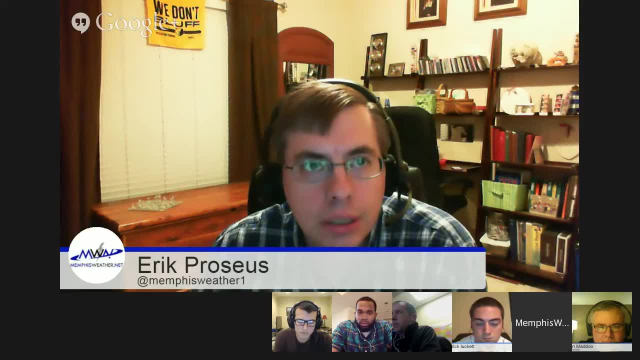 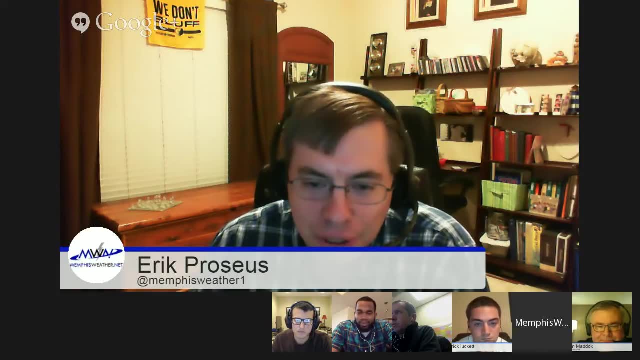 case it'd be nothing. but you know, depending on when you only get uh, you know a borderline one inch event every four years. i think my snow counter is at 1154 days since the last one inch snow here. we're due um, but but you don't have as much uh opportunity to kind of use that. 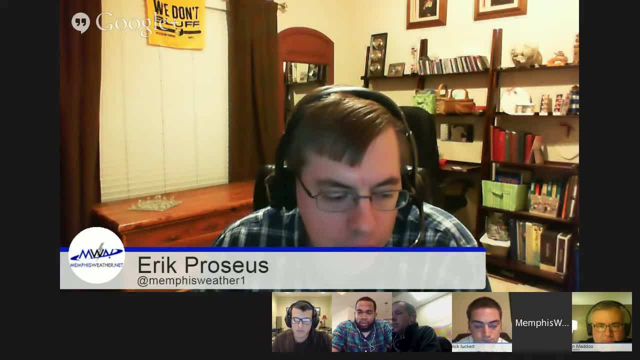 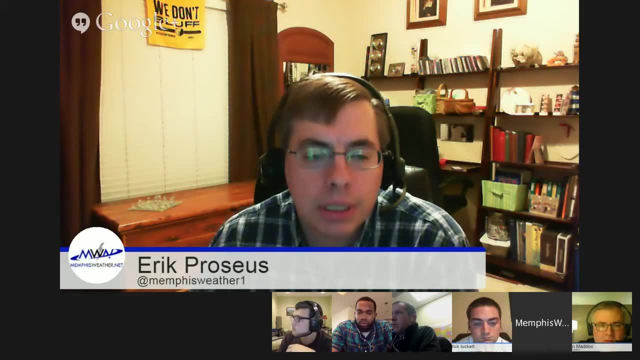 as much, but, um, it is a good habit to be in, i think, and it's a good way for hopefully the that the viewers are the users of the product, to get some- uh, you know, get some information out of that. that's useful, you know, eric, and i think the great thing about that graphic, too, is it's something that you. 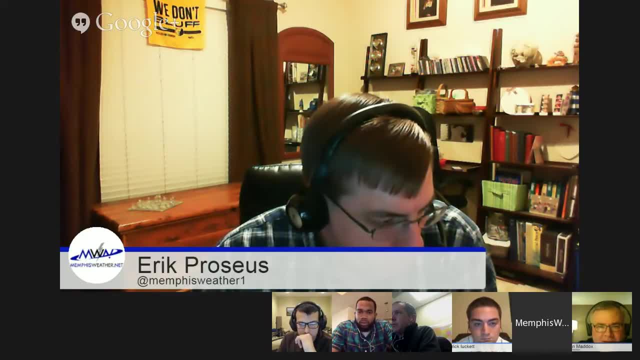 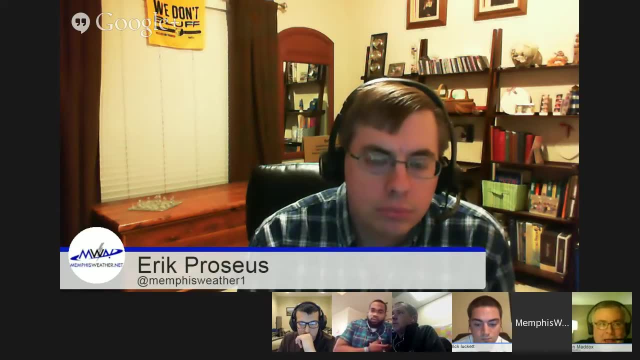 mentioned the ems and all that. everyone that looks at that graphic can understand it. i mean, you know that's. that's the beauty of it is, everybody can look at that graphic and go: okay, here are the three chances. i know how a quarter inch of snow impacts me at my house. i know where. 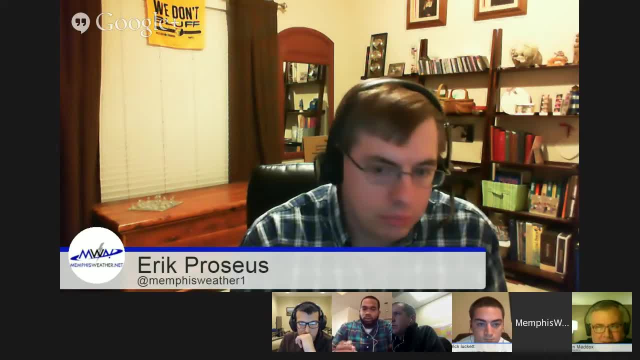 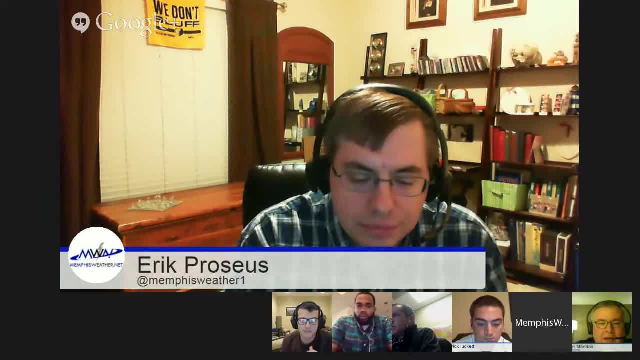 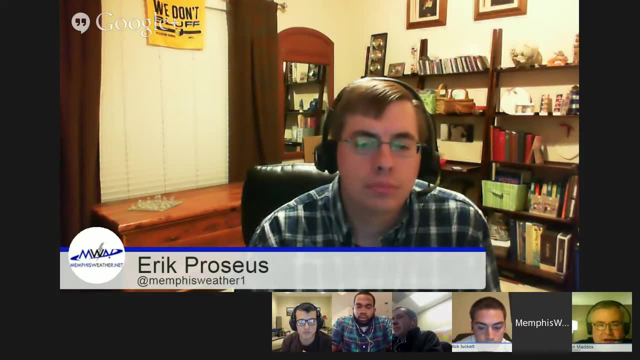 county you live in and and so on and so forth. but you know, everybody can look at that map and i want to commend the weather service because that's just, it's so easy to understand and everybody, every consumer, can understand that map. a lot of social science when they're in that map. in a short 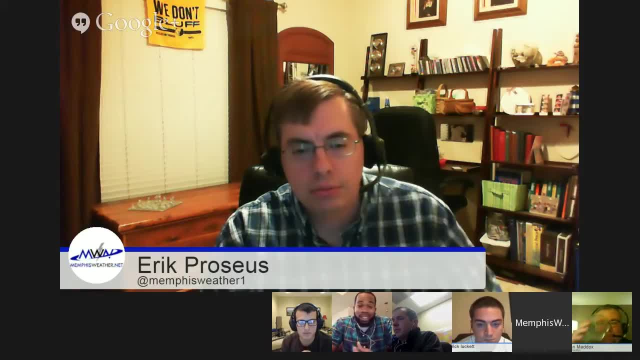 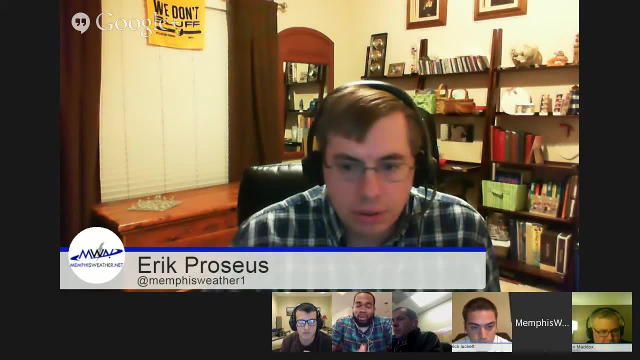 period of time actually, because the collaboration only started, uh, probably a week or so ago, uh through email, and they're not going to be able to understand that map. so i think it's a good way to and everything. so we did a lot of work with a local tv, mets and everything that see how we could. 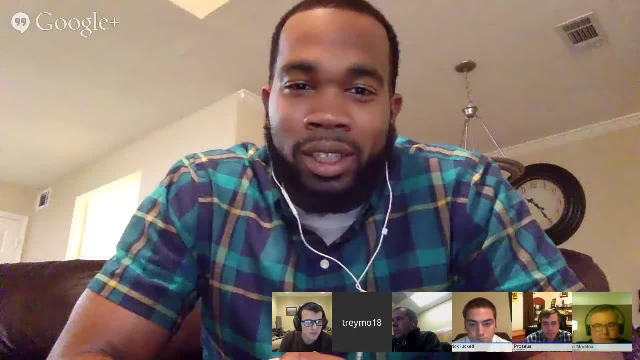 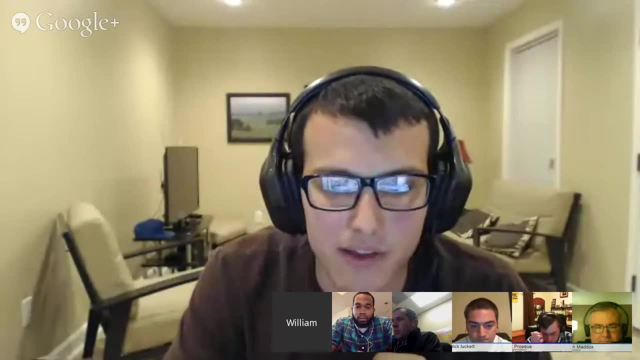 best convey those graphics to the public, and color schemes and everything. yeah, really nice. i just wanted to say real quick too that, um, i'm definitely for that and i think that's really awesome. you guys are starting that, because when you just pull up a weather service forecast grid, it's just like 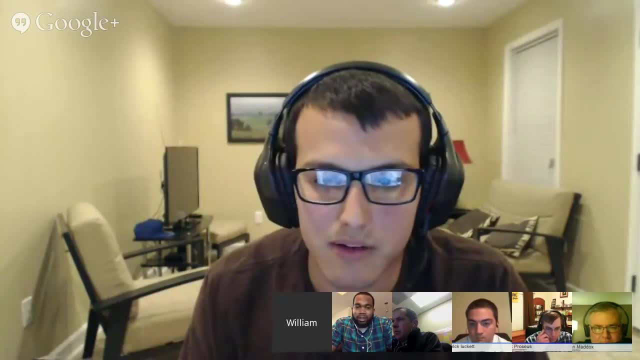 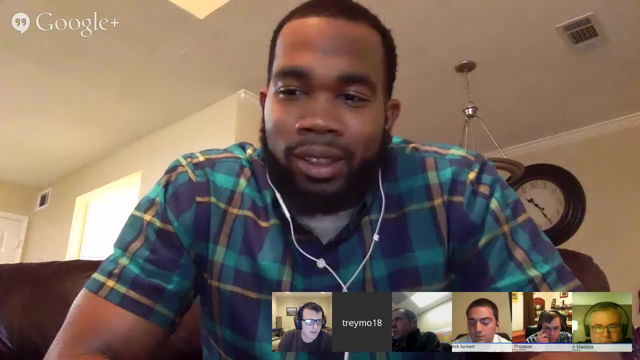 this is what's going to happen. it's just kind of like a you know, if you read that and you're like: okay, this is going to happen, this, so this better communicates what's actually possible. yeah and uh, i just want to throw out there, too, that it's always so much more important and not just 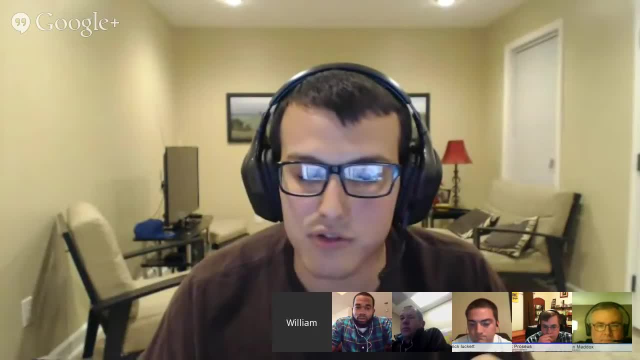 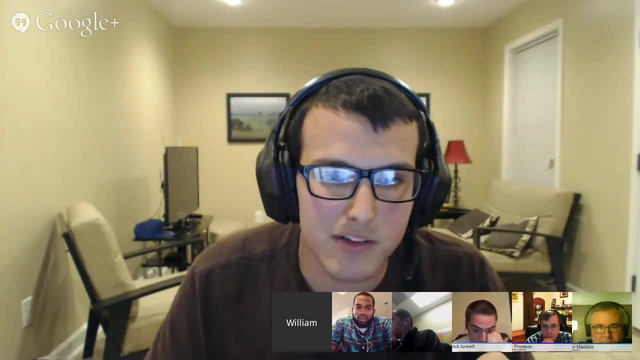 here, obviously because in new york city this happened. but the snow and ice impacts are just so much higher. so it's not like when we just have like a normal stratiform rain event. no one really cares if it busts a tenth of an inch or even an inch, it's just rain. so but when it's snow or ice, 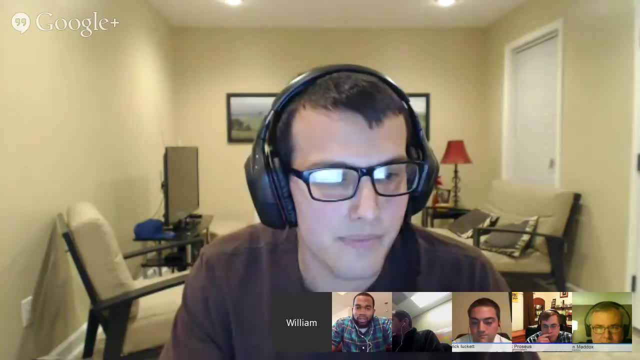 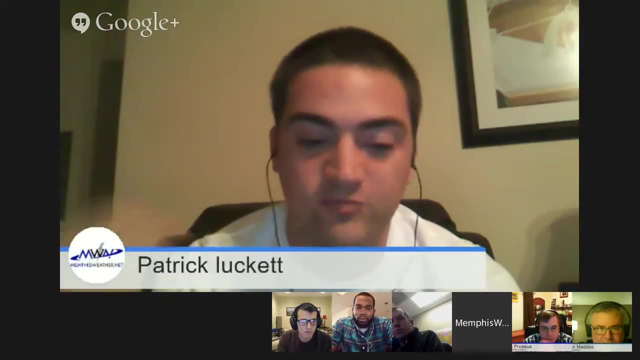 it's, the stakes are much higher and and so just kind of throw that out there, that that that exists too. so, jock, really agree, i saw that this morning and i just this is a really good idea. i think it's. this is brilliant. this is what they all should be doing, because it conveys the forecast as long 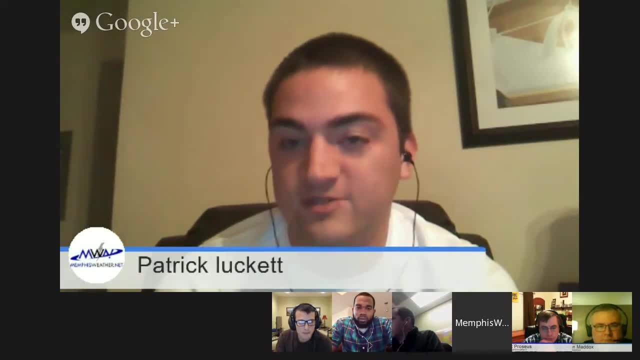 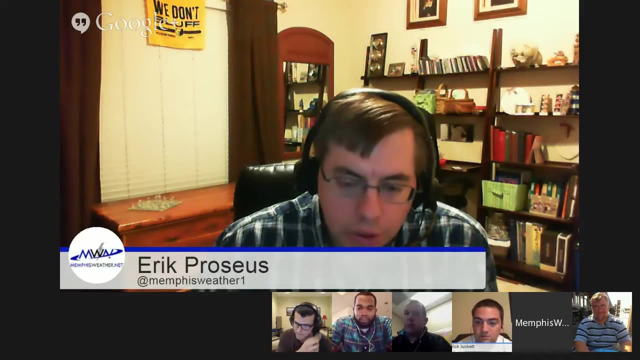 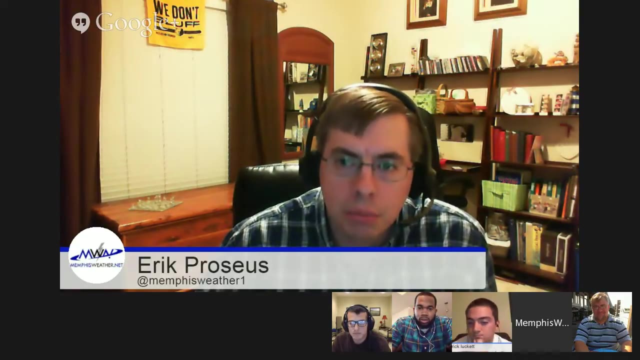 along with what the low end and high end possibilities are, and that's easy for anyone to understand, like john was saying yeah. so uh, john moore, do you think this is um, that this type of concept, using these um kind of range of options, is something that, um, i mean, i think it does have? 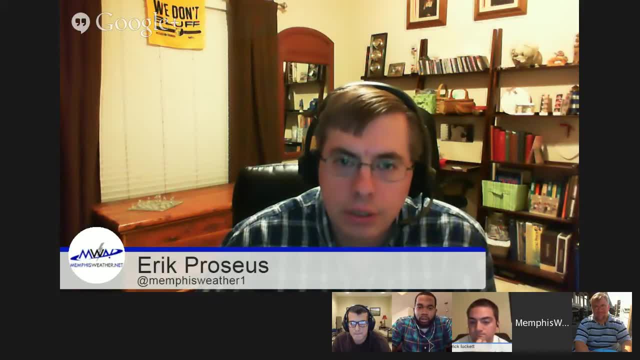 some application to say, severe weather type scenarios? do you have you guys even considered- uh, i know this is brand new, but it used to be a lot of time ago and i think it's going to be a lot of time to see that being used farther down the road for that exactly. we actually had this conversation in 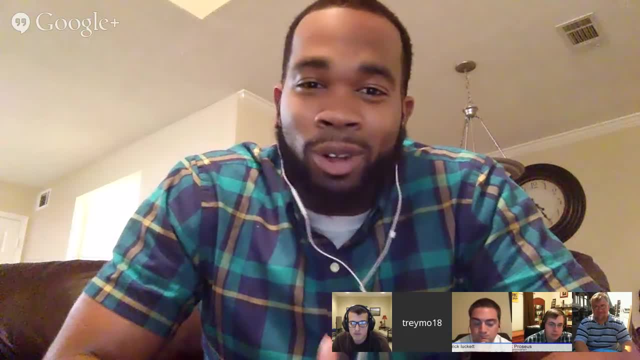 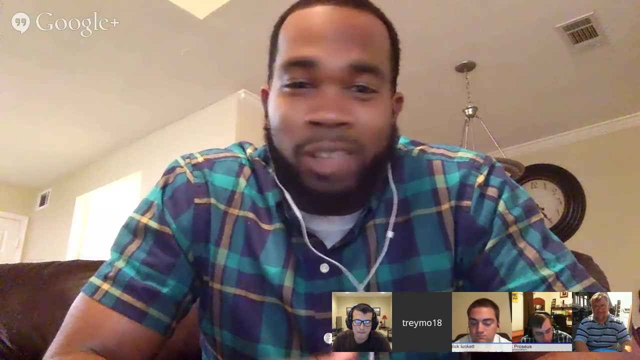 the office today of me and gary would all had it, and how best we could, uh, turn these type of situations, that type of graphic, into a severe weather graphic. so, uh, it's going to be some more coordination with the spc and maybe they can up their game a little bit on that end would. 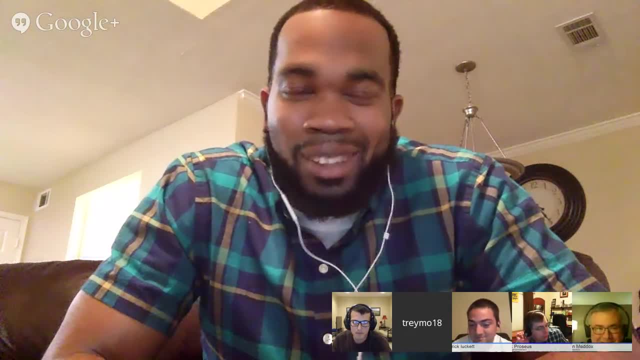 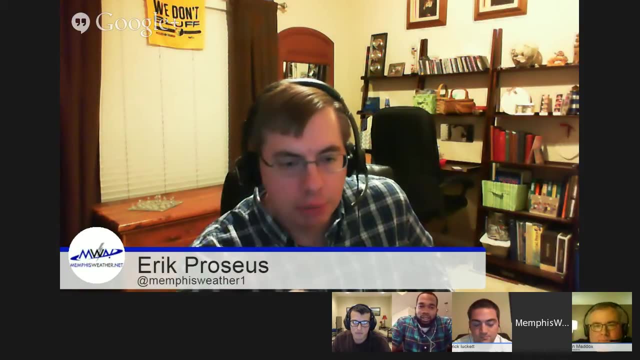 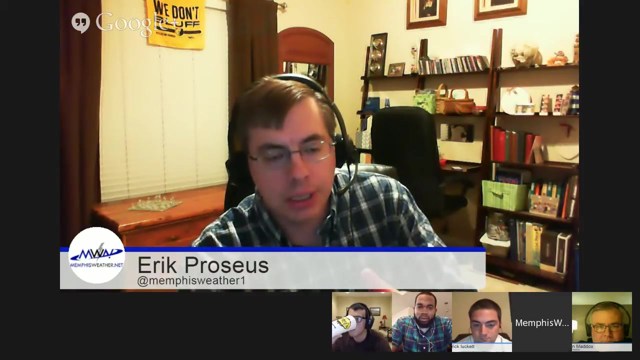 coordinate uncertainty with their graphics. yeah, they're, you know they, they, they provide a lot of that information um in in probability scenarios so you'll see, you know, probability of hail and severe wind and and tornadoes and so forth, um which then goes into those probabilities then are basically the direct input to what risk zone we're going to be in. 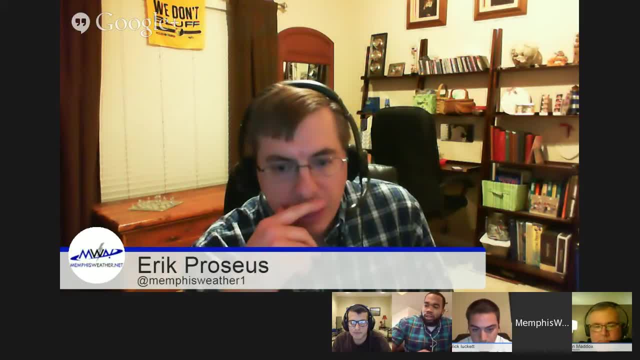 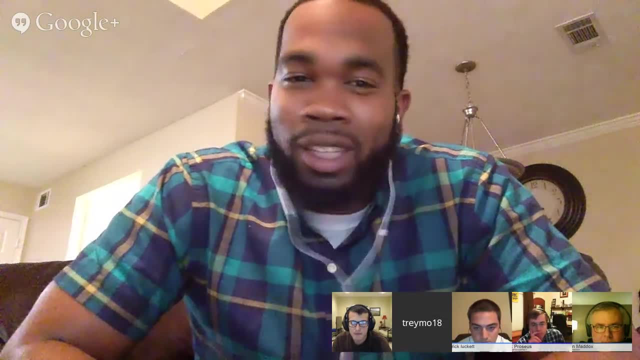 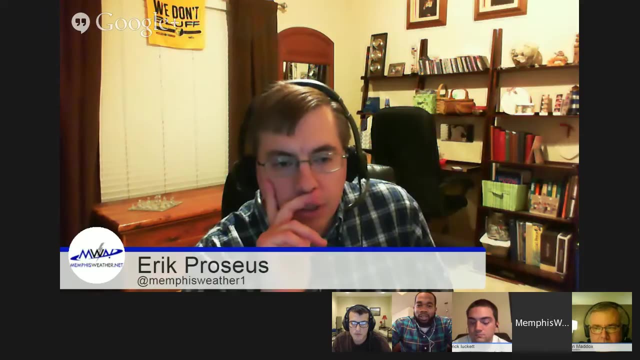 whether it's a, you know, an elevated, moderate, slight, whatever, even with timing, even timing graphics. if we're uncertain with timing of the following storms or greatest potential timing, uh, we can convey that in three different maps or three different, three different confidence types, sure, sure, a lot of, a lot of different applications to that. 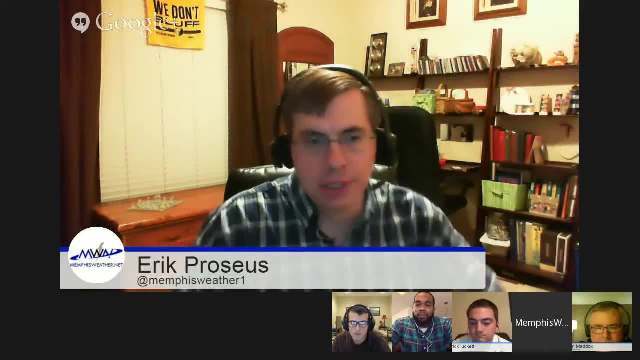 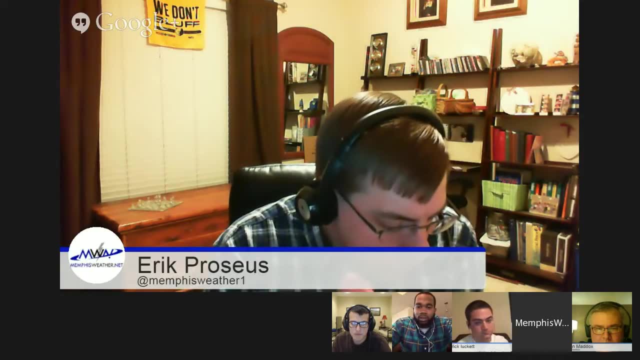 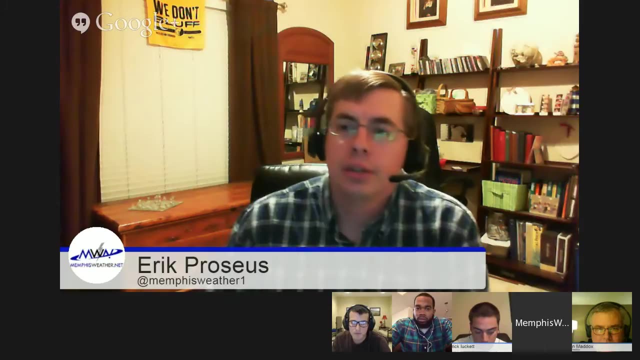 um, yeah, i look forward to seeing some more of that and seeing how that, uh, how that works out. so, um, that's good, um, so here's a question that, uh, that i want to pose to you all as well and kind of get everybody's opinion on. so, after this event last week, um, everybody of course knows that new 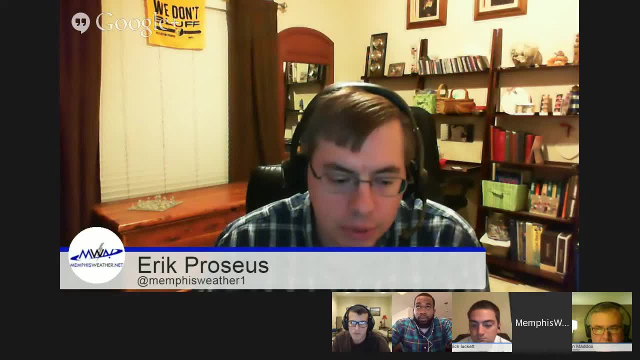 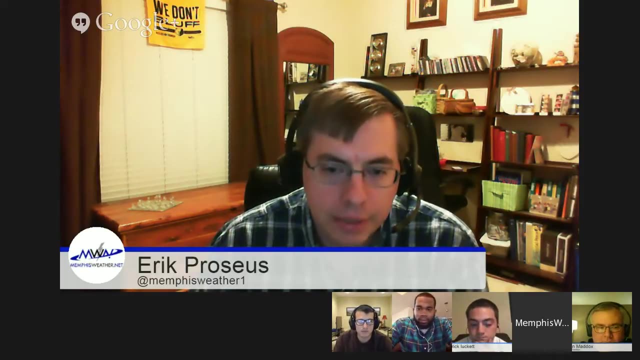 york city quote: busted the forecast you know it was. it was six to eight inches instead of 22 or whatever. so one of the first things that happens is you get public officials from local and the head of the national weather service out basically apologizing for a blown forecast. um, and now the director of the weather service, uh lewis usalini, also used the. 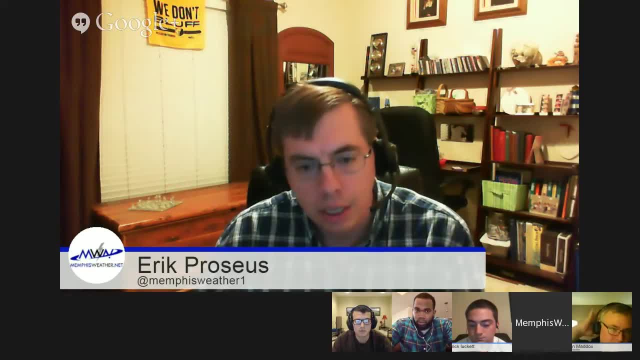 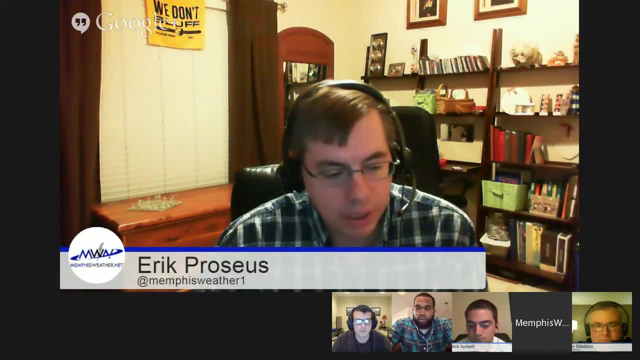 opportunity to kind of educate and say: well, you know, this was kind of what we're looking at and and this was the scenario that was playing out- um, but uh, you know the same guy at uh, at the philadelphia weather service office that's in charge there, that um basically put out the plea. 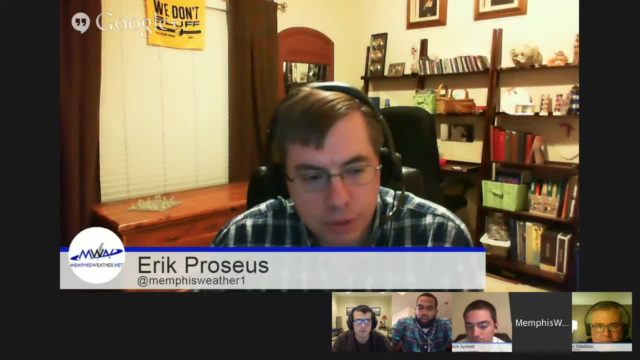 before sandy came in. um was the one that was the one of the first ones that was in charge of the storm warning. they said: you know, does this mean that i'm not going to be perfect every time? um, i think it's the most driving factor. i think that's what i think right now. i think it's the most. 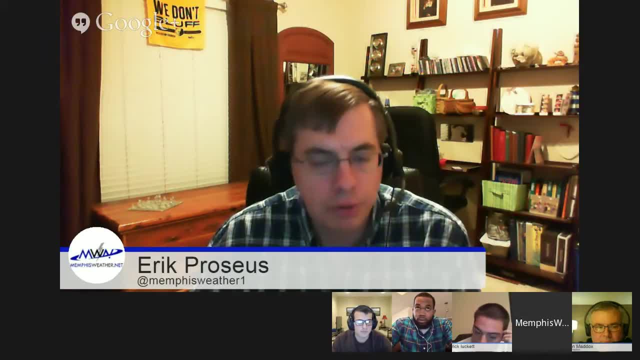 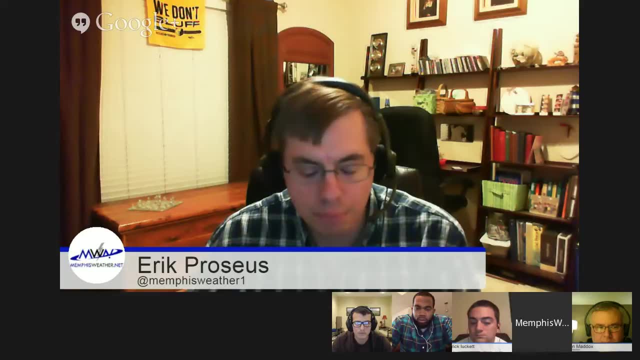 driving factor that's going to happen in the future. yeah, i think that's exactly right. what i think about it is: it's a, it's a joke. it's a joke, at least for me. it's a joke for me. but when it comes out and and uh, almost i almost want to say remorseful for, for the blown forecast, so what? 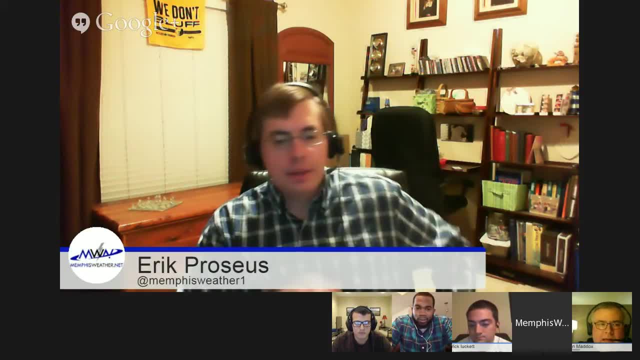 do you guys think when you're in a position where you're putting out that information, it has uncertainty? that's that's built into it. everybody knows that you're not going to be perfect every to end up and, rightly or wrongly, the public views that as a little self-serving. 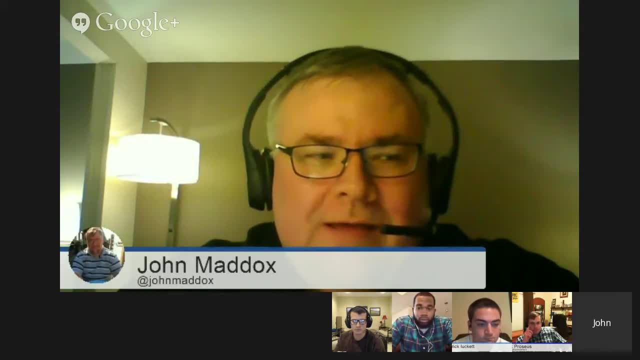 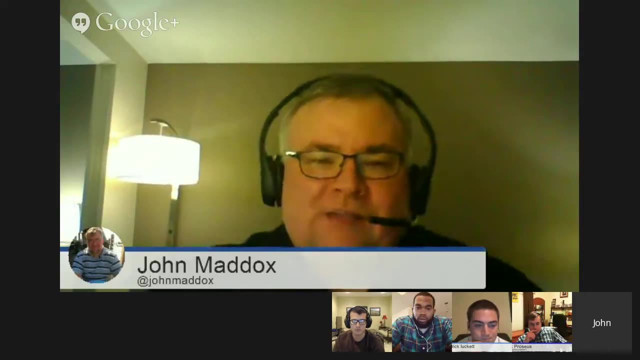 and a little you know, oh yeah, you screwed up. It's kind of like a referee in football or basketball or whatever sport. I think we all deep down would accept a little bit more. these things happen. but that's why I think, if you forecast, 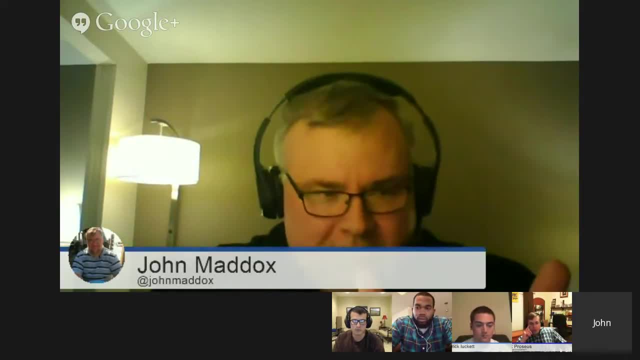 the way you guys are talking about, where you say: look, here's what we think will happen, here's the other two. then apologies aren't really necessary. I think that you know what happens is what happened in Buffalo, as you said. I think it was. 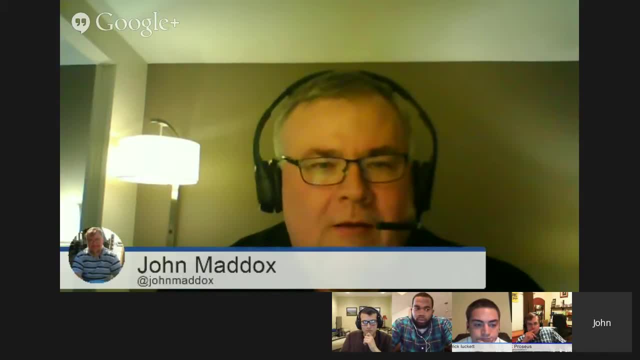 the governor of New York said: you know, there was no warning, we weren't prepared. Well, you know. and then everybody scrambles and goes. well, if you go back and look at the forecast discussion from four days ago we were talking about 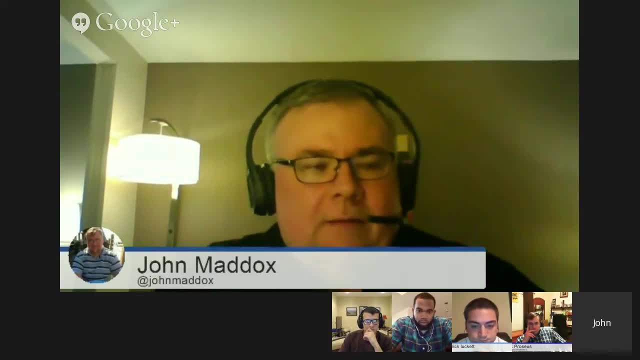 this. Well, the general public doesn't look at the forecast discussion, So I think that's where the line is kind of balanced and I don't know. you know I don't apologize to the public when I make a mistake. 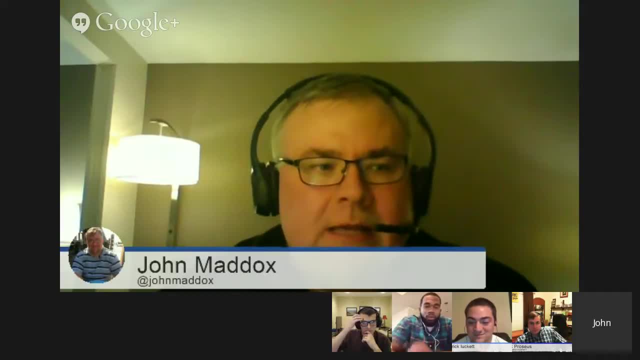 You know at my job. I mean, granted, my job's not you know in that sector, but I just think you run the risk of when you start apologizing all the time. you know when a storm takes a, what was it like? 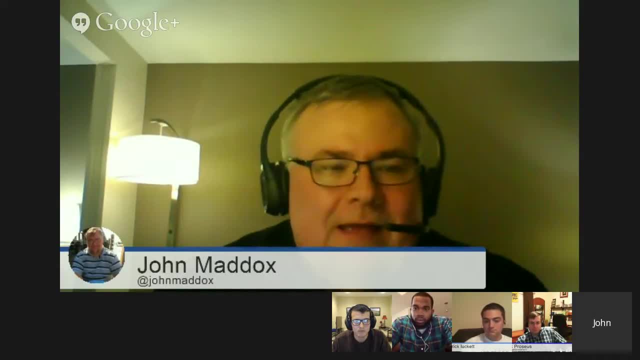 a 40-mile deviation to the east. I just think you're going to spend half your time apologizing when people are going to have the same reaction. People are going to be angry, people are going to be upset. So if you come out and apologize, 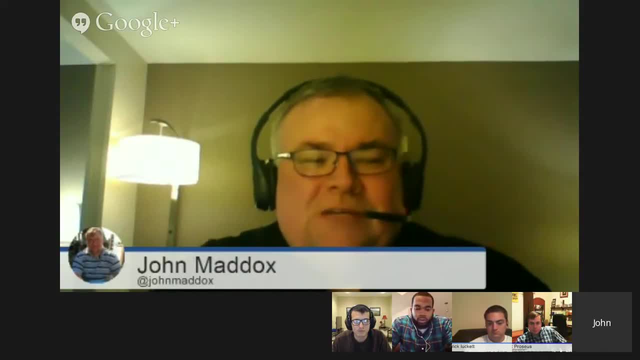 does that and, John, you're maybe more in tune with this, but does that sometimes make the situation worse than if you just, guys, just kept? you, just keep on, keeping on, because people are going to be angry and upset anyway, so why put? 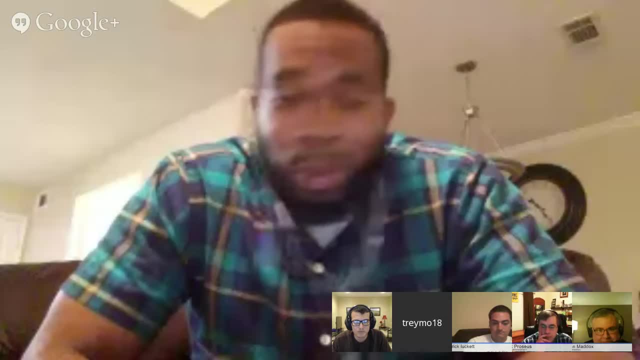 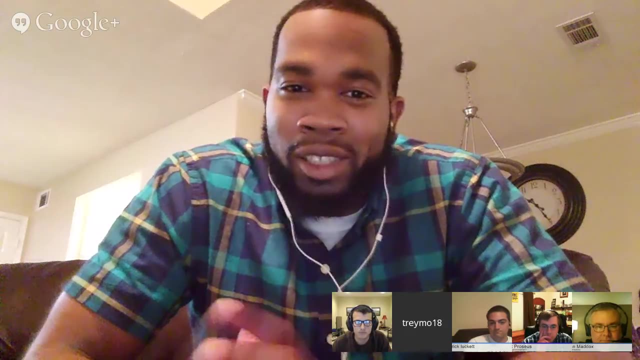 yourself through that? I don't know, Just my thought, My personal opinion. I would never apologize for a forecast that I use Every tool that was at my disposal to use and all the outlets to get it out. I'd never apologize for a bad forecast. 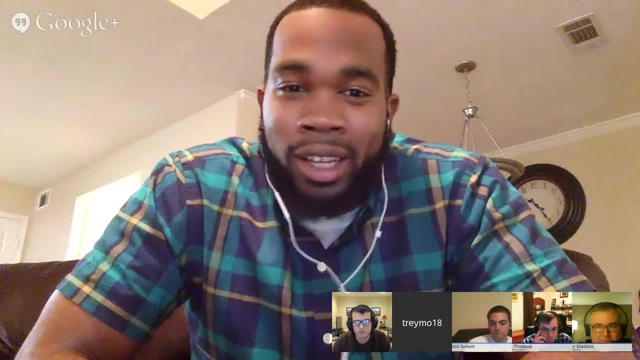 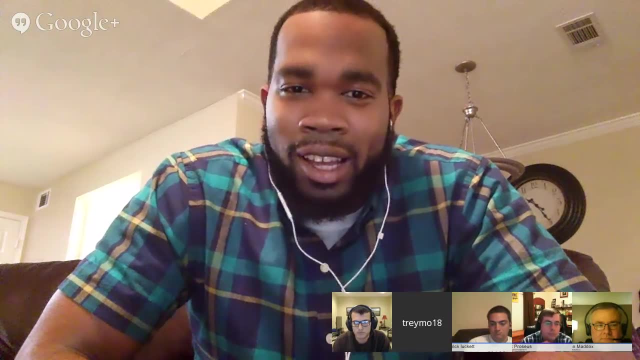 Who's to say it was a bad forecast? It wasn't a bad forecast, but what's going to come of it if we keep apologizing? It makes the public lose confidence in us. And as far as apologizing, what happens if I issue a tornado warning? 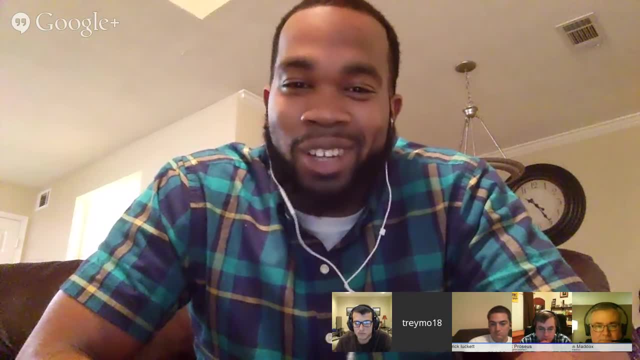 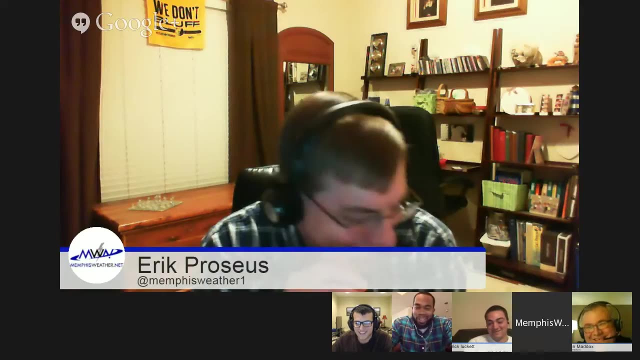 We don't have a tornado, I have to apologize, because a tornado warning is no tornado, So if a thunderstorm warning is not verified, I had to issue a lot of those last year. My FAR is pretty good but it's still pretty low, so I'm not apologizing. 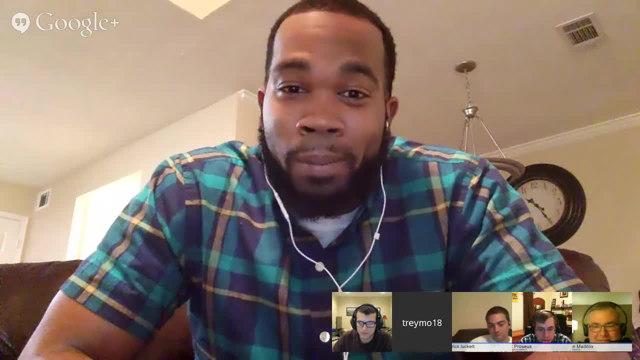 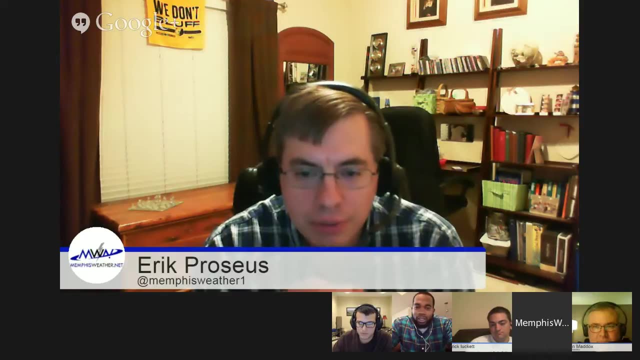 for that I'm going to apologize, for trying to save lives. Well, and in effect, are you really just apologizing for the data and so forth that you're looking at? I mean, if you're using all those tools that you have available to you? I'm not. 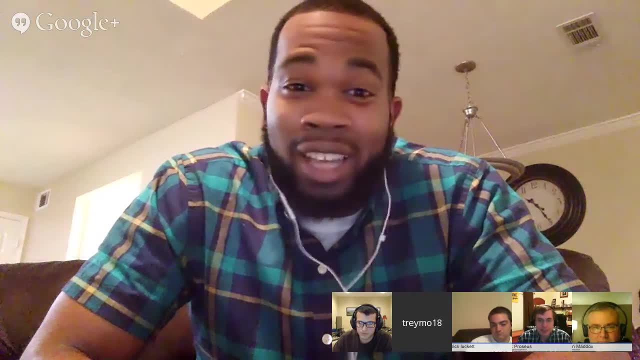 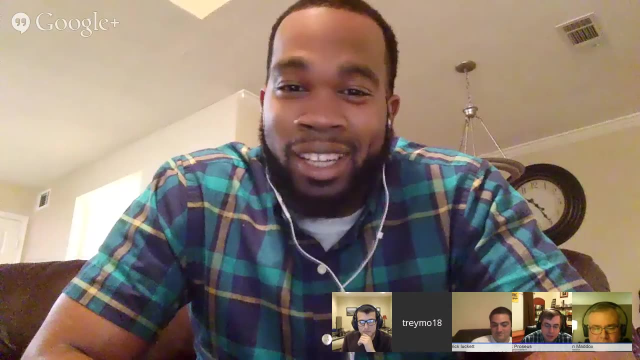 apologizing for the GFS being bad. Someone higher up than me has to apologize. This person making the calls has to apologize. This is my personal opinion. I'm not about the service, but I cannot apologize for something that I try my hardest on. 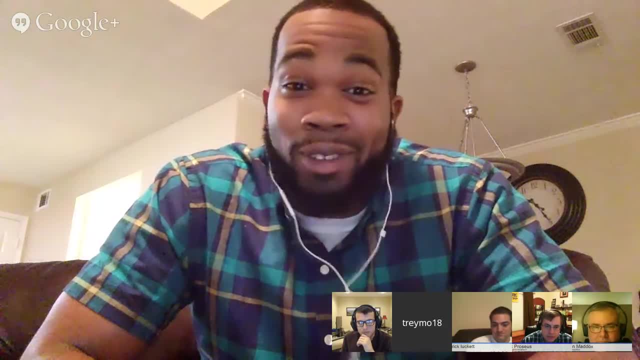 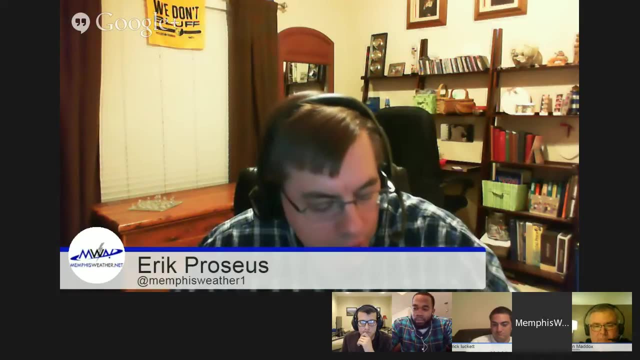 I guess that comes from my athletic background. I was always taught that if you try your hardest, there's no need to apologize. Yeah, How about? how about you guys, Patrick or William? you're kind of on the young end of the. 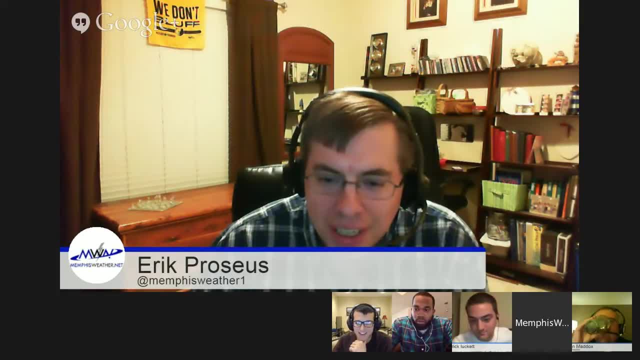 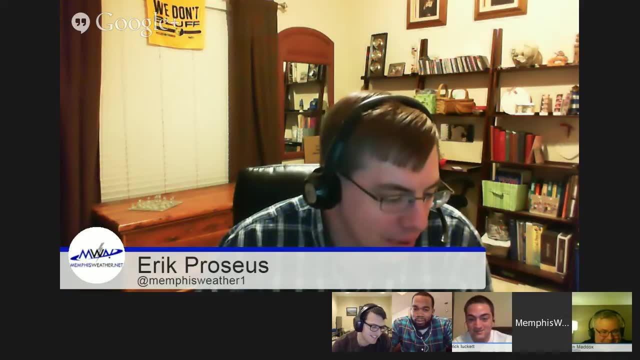 I haven't had any forecast to apologize for yet. but what do you guys? because you guys are still perfect, You're zero for zero, right, But no, what do you guys think about this whole thing? I mean, you get a job at the weather. 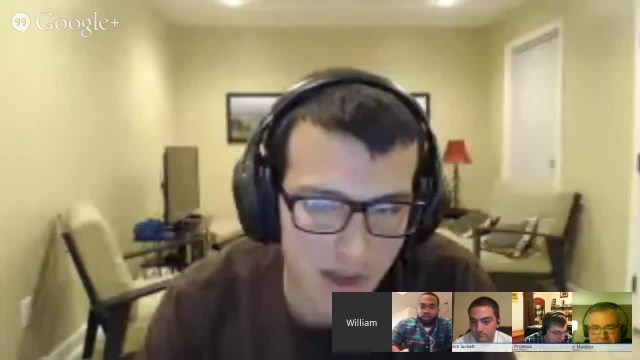 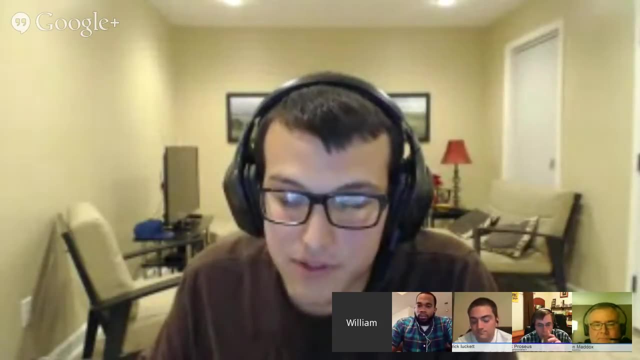 service or whatever. where would you go with that? Well, I personally think that this was more of a unique situation for those specific offices, because they kind of realized they really screwed up Because if you look at that map they definitely busted in those specific 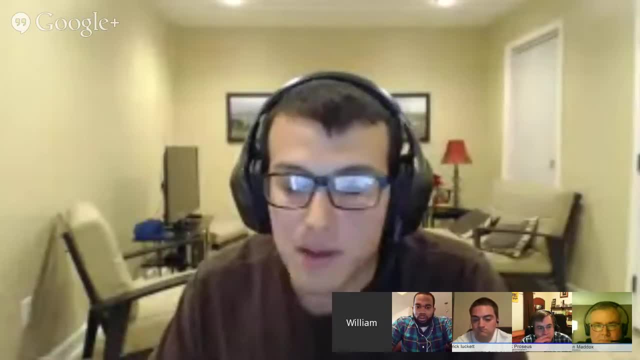 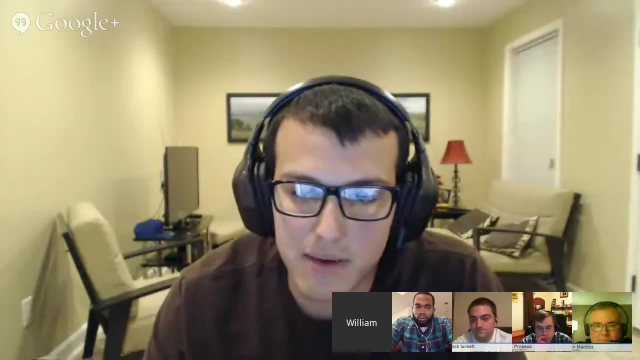 weather forecast areas. But generally speaking it was a good forecast, but maybe they feel like they didn't convey that uncertainty well enough. So I think in their case: hey, you were advertising potentially a record-breaking storm and you had a huge bus, So 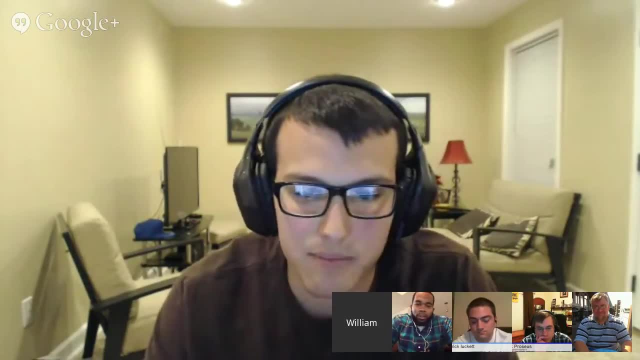 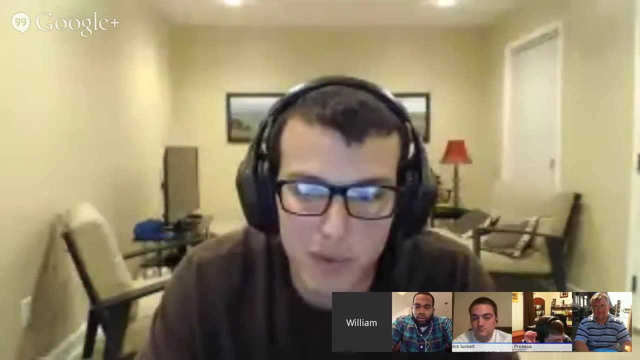 maybe an apology is kind of warranted in that case. But generally speaking I'm with both Johns here. I don't really think they should be going out on a limb and apologizing, especially for just normal bus. I mean, as long as you're kind of conveying what. 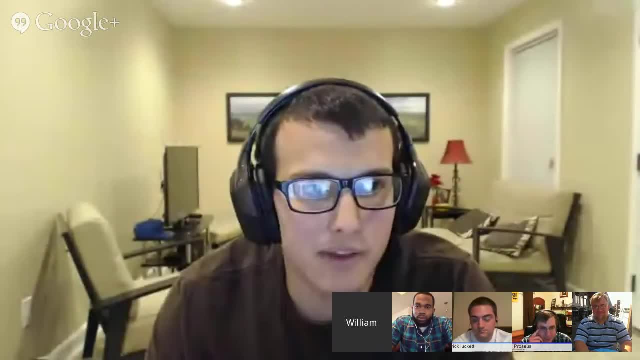 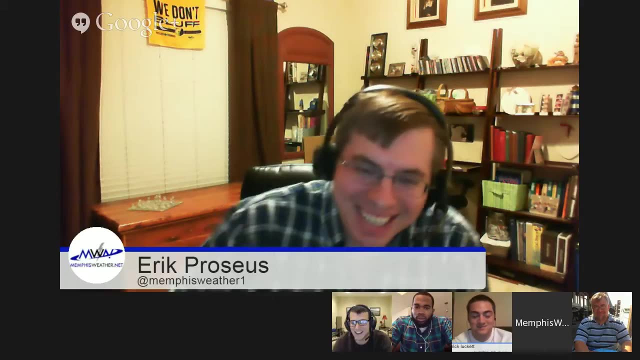 you think's going to happen. I mean, generally speaking, I don't think it's necessary. As long as you put a 14-inch deviation for your forecast in the normal bus category, I guess you're right. No, I'm joking. 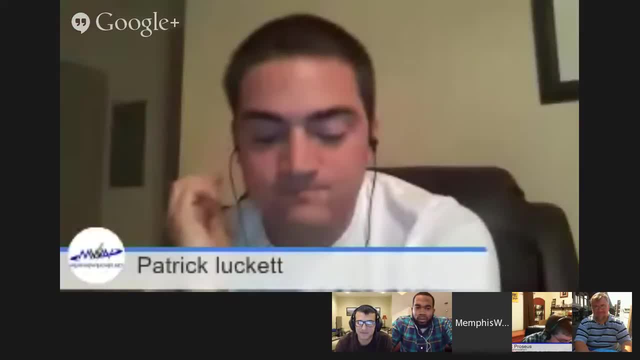 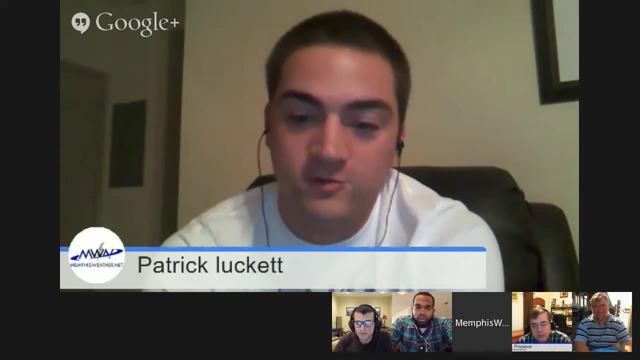 Any other thoughts, I would say that you don't really need to apologize for it, but rather than that, say what you're going to do better in the future, like with the forecast graphics that y'all are making now. If you just come out and say: 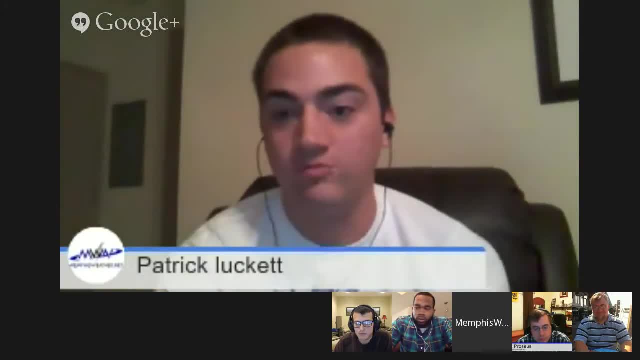 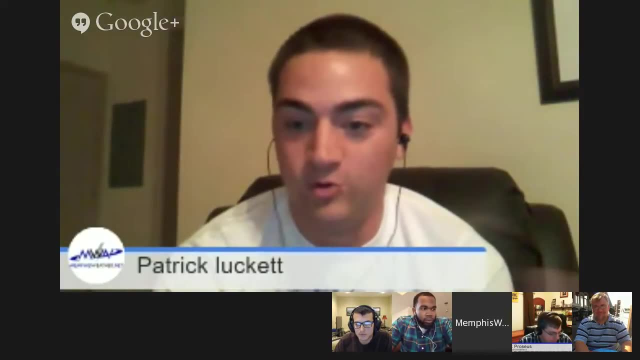 in the future, we're going to be using these to tell y'all the deviations that are possible in the forecast, rather than just having a set number that it's going to be 40 inches of snow in New York City. I really like what the head of the weather service did. 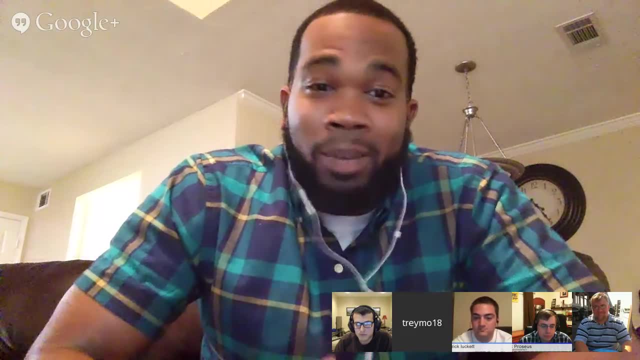 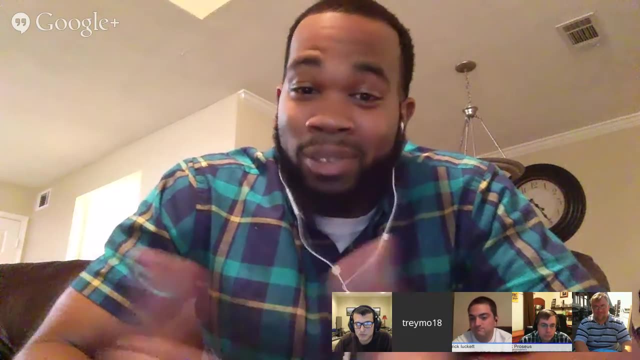 he came out and he displayed to the public. we were wrong and this is why we were wrong. He didn't apologize, but as long as you let the public know that this is not a perfect science and we're trying to get better, and this: 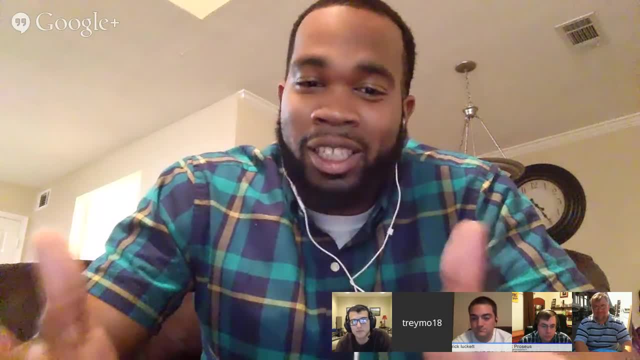 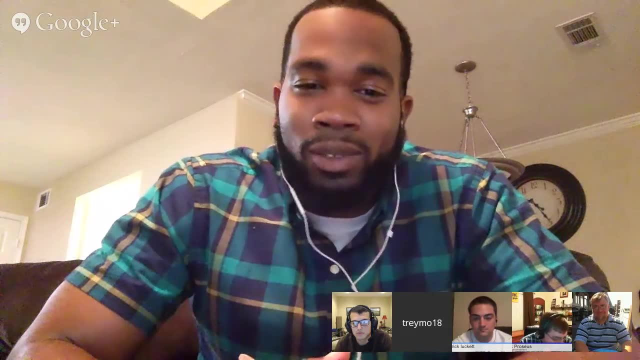 is what we have at our disposal and we're going to continue to serve it as best as we can, so it's no need to apologize for that. Just make sure they understand that we're trying our hardest with what we're giving. Yeah, ideally, I think that. 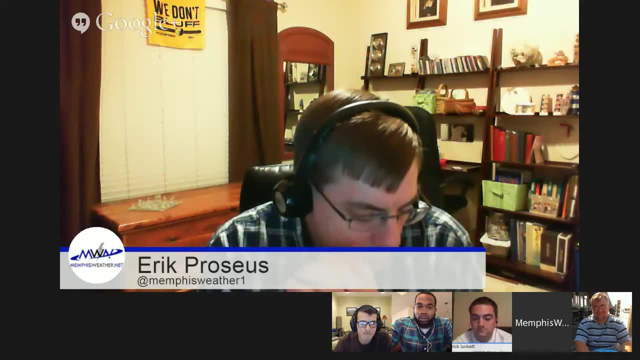 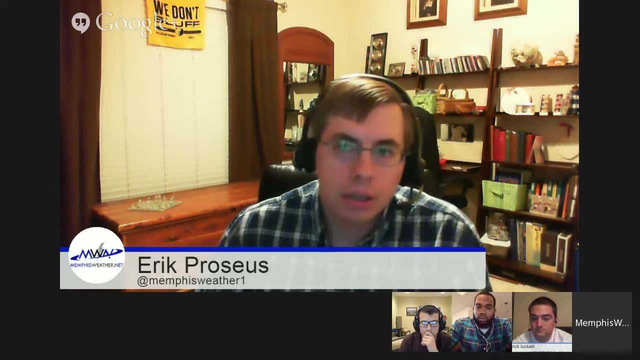 is better. That kind of segues pretty well into one of the other thoughts that I've got, and that is that all of us that are in this job, in our jobs, a lot of jobs. you're in the job because that's just. 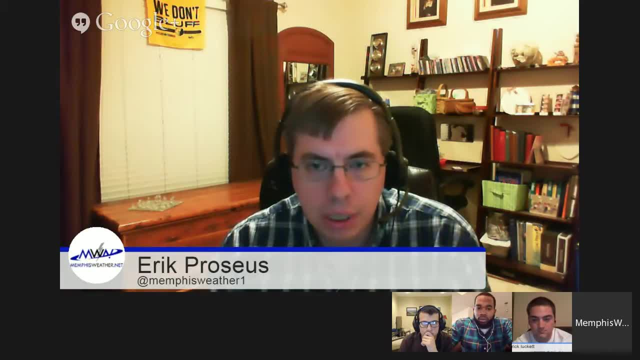 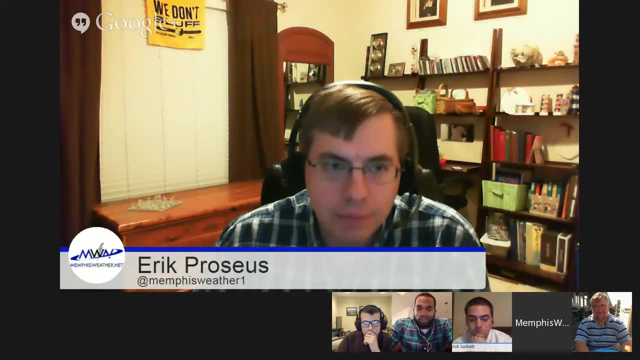 where you ended up. You're not there because you necessarily had a passion for that career and you always wanted to do that, since you were five or whatever. I've met very few meteorologists who aren't very passionate about what they do, and weather is their thing. 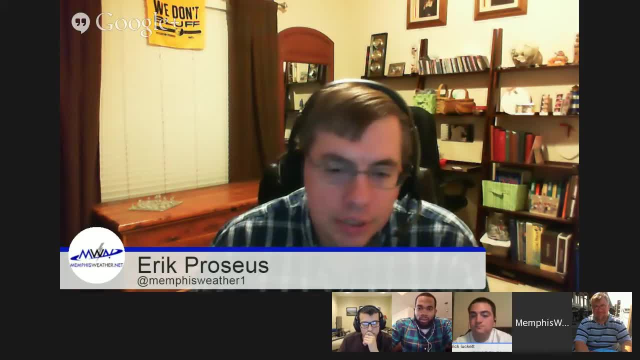 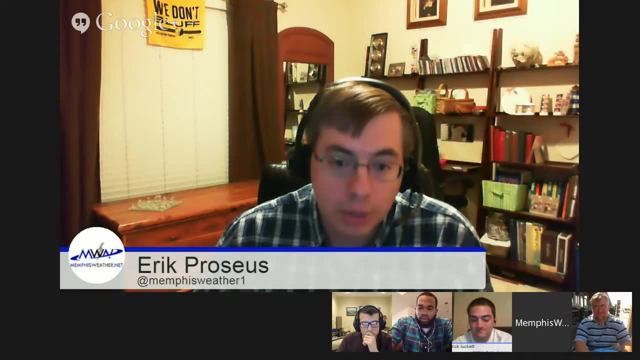 If they weren't getting paid for it, they would probably still be doing it anyway. We pride ourselves not only on our accuracy: we know when we screwed up. We're going back and looking the next day and going: man, I was off by 200 feet on the. 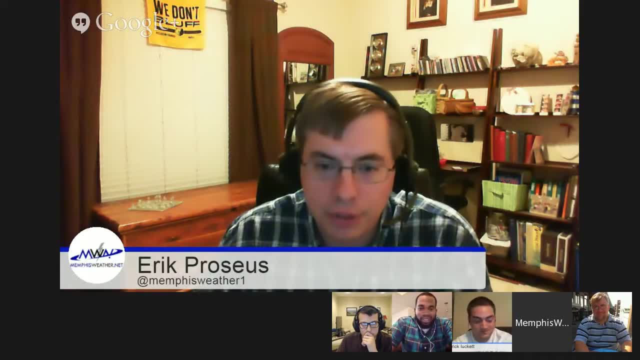 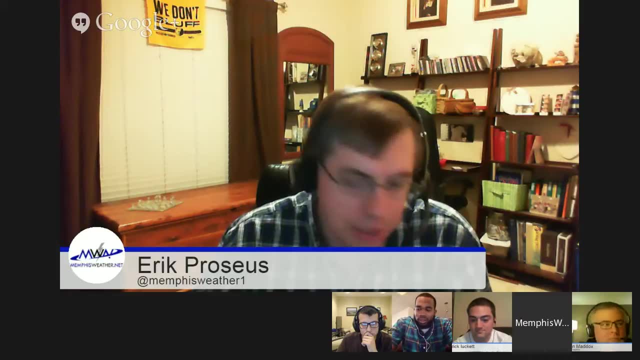 ceiling in that aviation forecast, or I've called 55, and only got to 53. How did it only get to 53? Was it that high cirrus deck that kept it down two degrees, or whatever? We tend to be pretty hard on ourselves as a group. 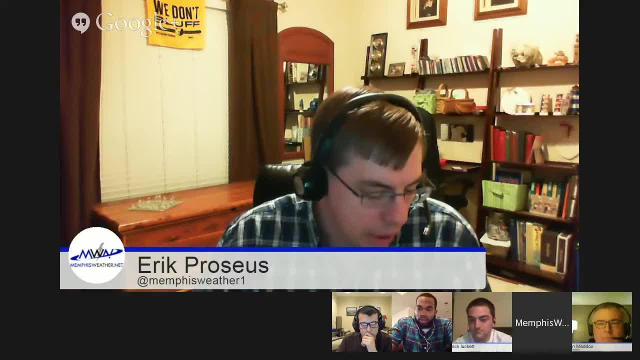 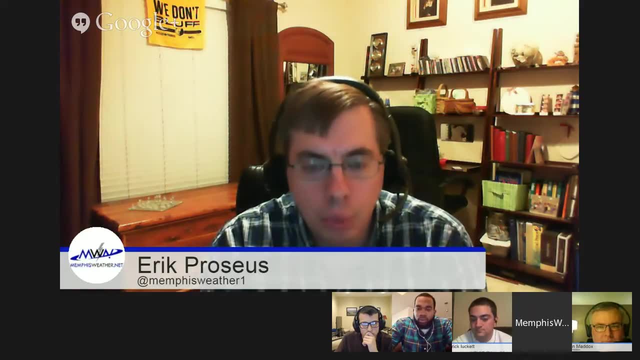 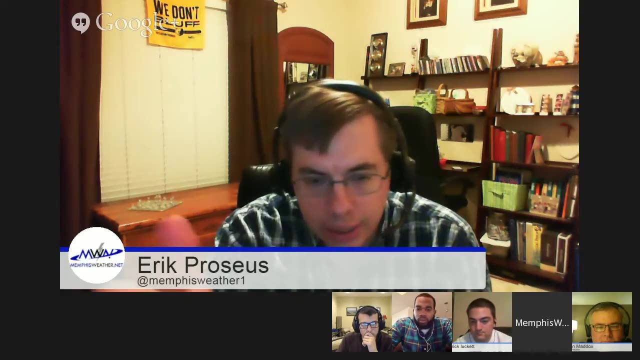 I think. I think that because of that, we're always looking for ways to continue to better what we do, how we present it. All of this, I think, is a learning opportunity for all of us, Just like the Weather Service here in Memphis is. 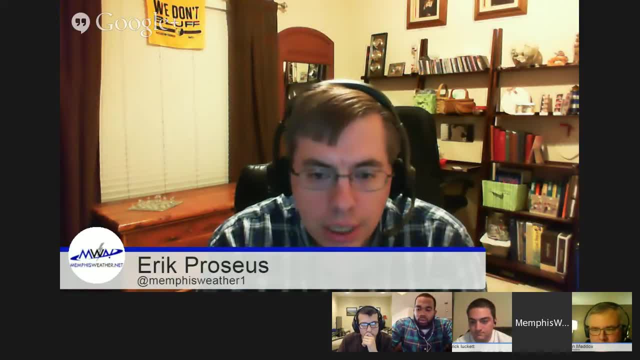 in a week, rolled out a new graphic set that they're going to be using. It's all about lessons learned. If we didn't take pride in what we were doing, we wouldn't care that we were off by whatever, and we'd just go on about our business and keep doing. 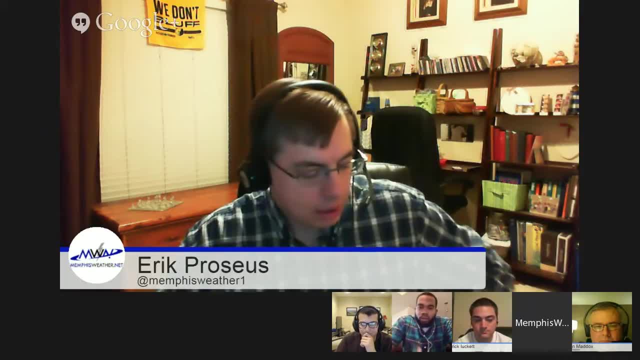 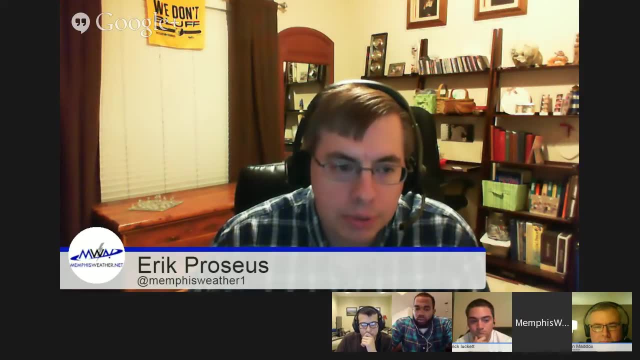 the same old thing, I think, that's. we're continuously learning, We're continuously taking feedback. We know when we screwed up, so we don't have to have all y'all tweet at us to tell us that we were off by two degrees. 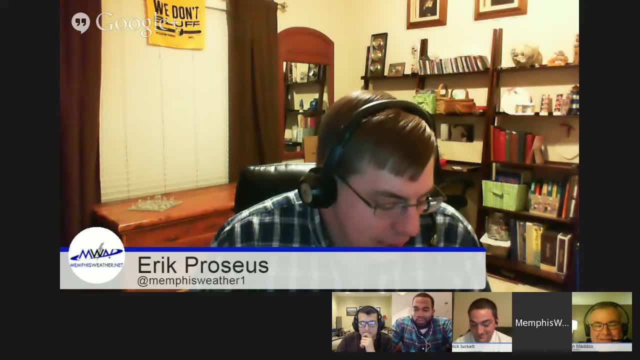 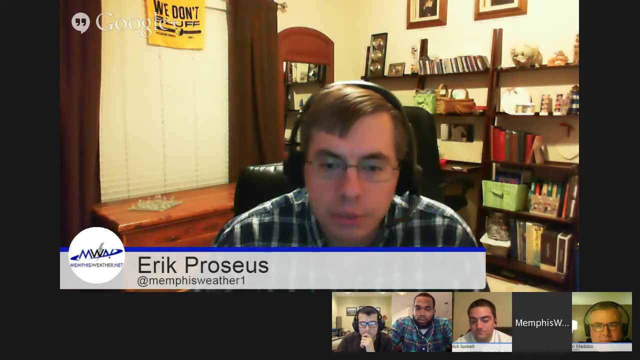 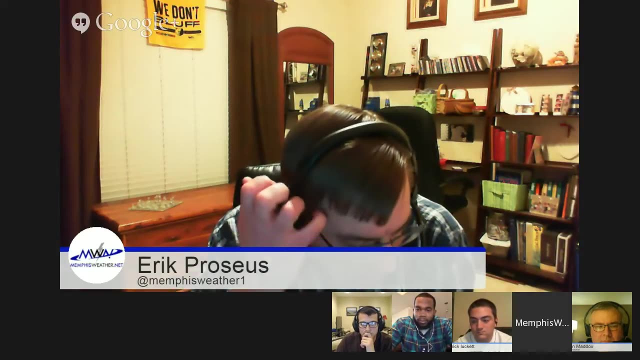 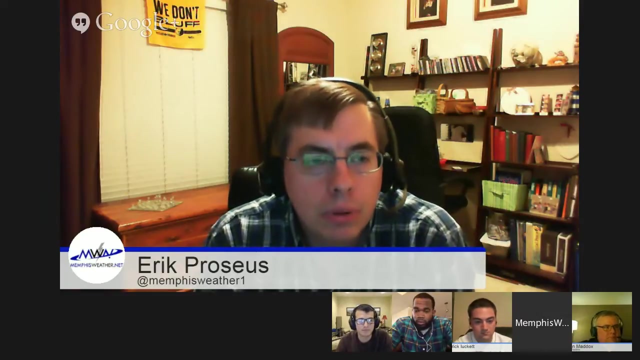 We know that, But it's something that we continuously strive for and try to create things that will meet the needs of the consumer. With that, I think that from the consumer side then- and we touched on this a little bit ago- that there is a responsibility also. 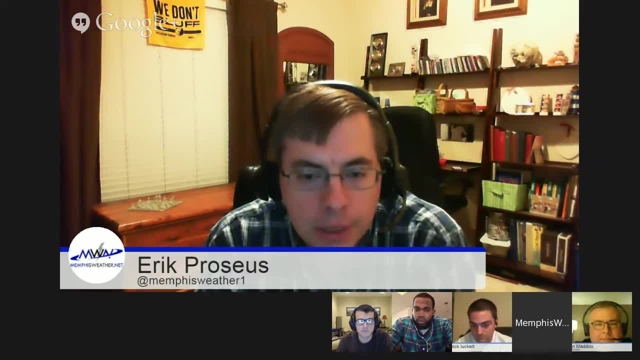 on the people who are getting these forecasts, That you have to not only stay in tune with what is being communicated to you, but understand what those impacts are as well. How is that going to affect you If you don't know? my gosh, there is two-way. 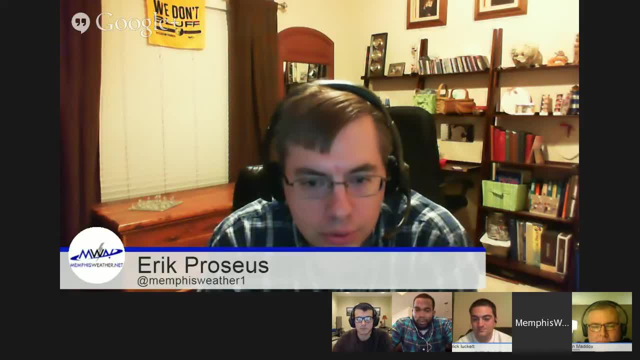 communication all over the place. now It's pretty easy to get a hold of somebody, and if you aren't getting response from someone, then there's probably someone else who will be able to help you out. I think it's incumbent on the consumer. 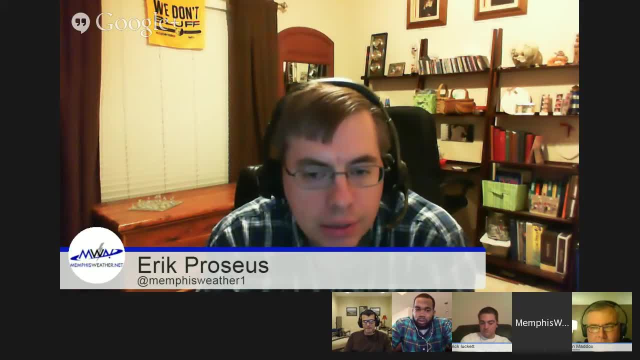 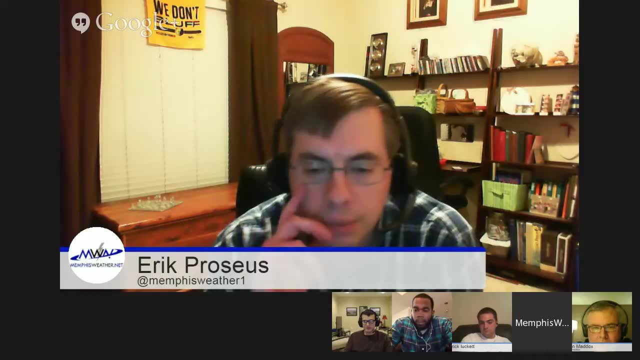 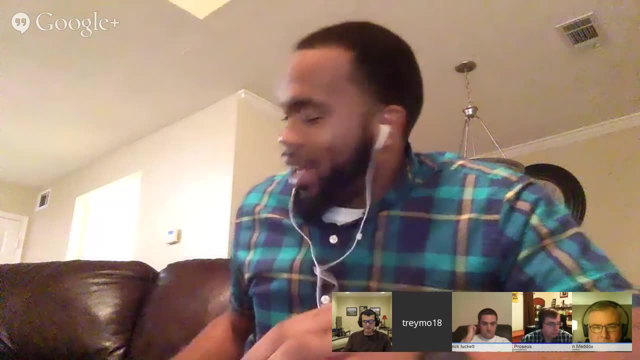 also to use the information and to help us figure out what's the best way to communicate that. I know the Weather Service is doing a great job on that two-way communication. It really stepped up the game in social media across the nation. Yeah, we really have. 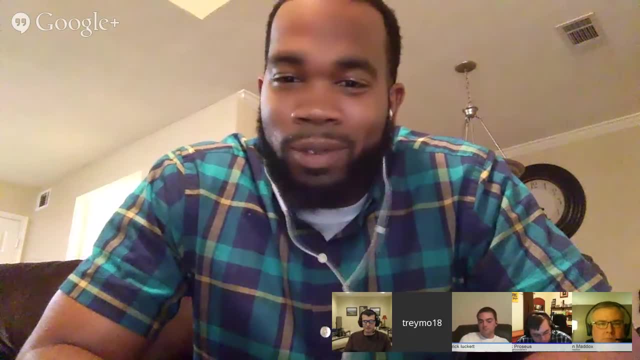 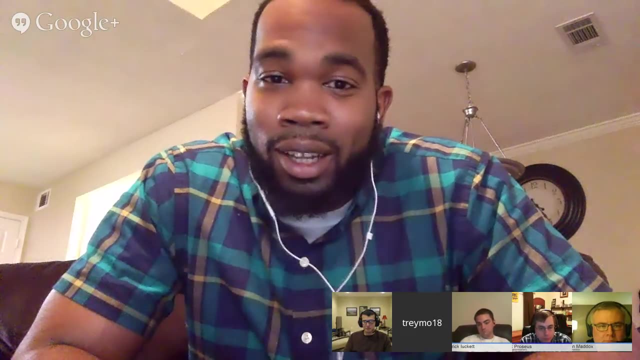 The last few years we've seen our followers on Twitter, Facebook, almost quadruple in some offices. We're still far behind the other offices in Memphis, but we're making big strides. Making big strides? Yeah, definitely are, Definitely are. 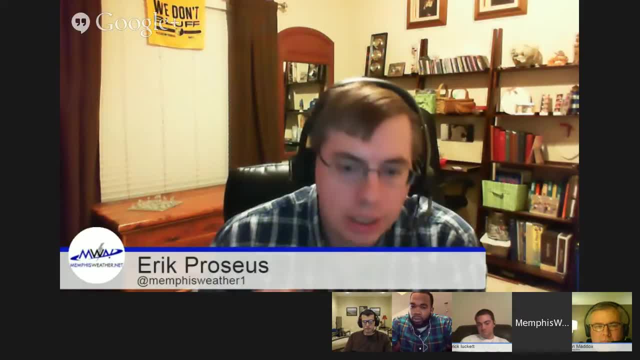 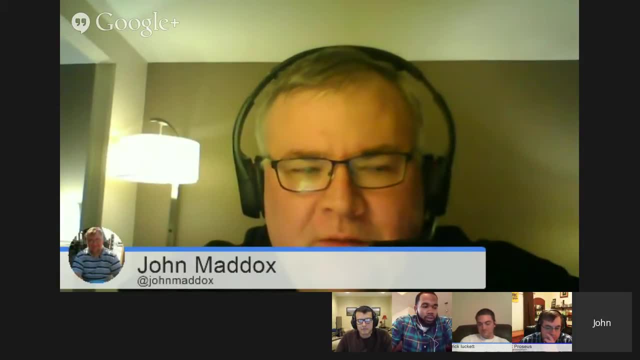 Any other guys have any comments on any of that? I just you know. going back to consumer responsibility, I agree with you that if somebody at the Weather Service isn't responding to you, obviously you guys are very active on Twitter, but we do. 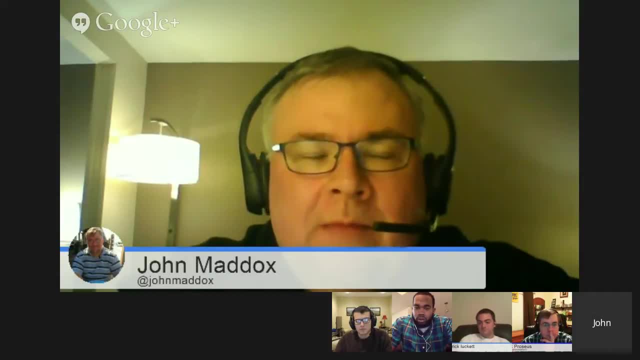 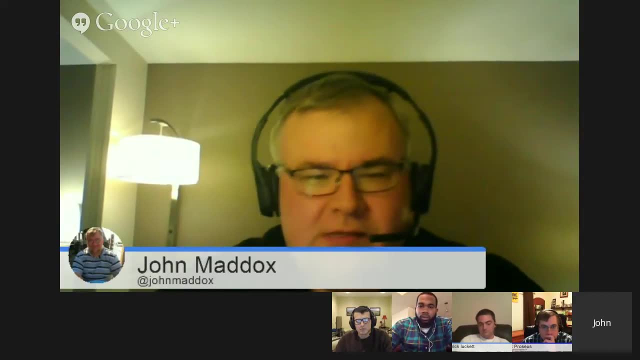 have a responsibility as a weather consumer- which is more what I am than anything else is- to you know, be aware, Just you know. for us, if you guys busted a forecast between 6 inches of snow and 22 inches of snow, it's not going to matter. 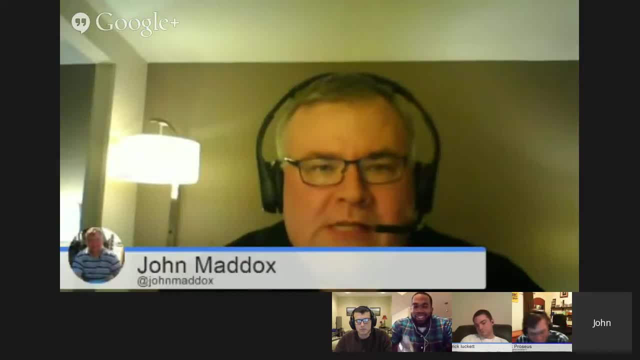 for Memphis 6 inches of snow is. you know that's a paralyzing snowstorm. So you know, if you say, hey, we're going to get 6 inches and we end up with 15, then everybody loves you guys. 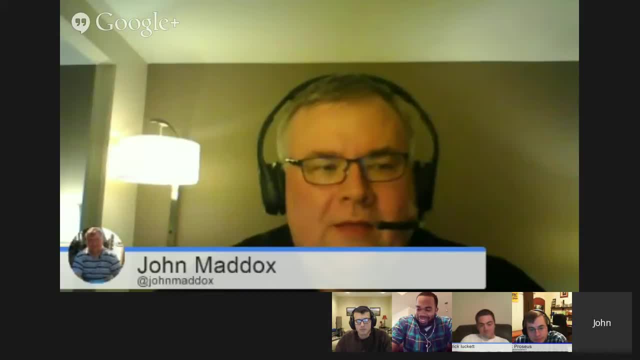 because we get more snow than we're supposed to. You know where I think that our similar situation is what happened- I think it was 2 or 3 times last year where you know, it was 33 degrees and rain at my house. 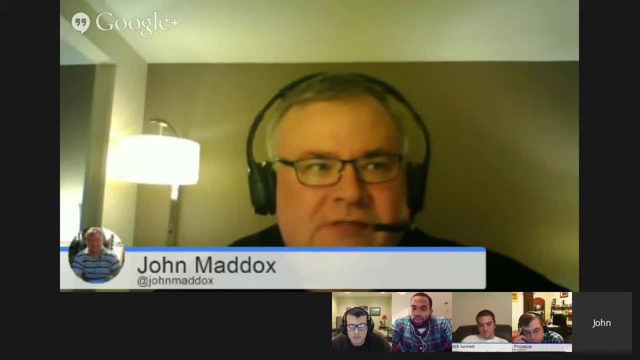 in Fayette County and, like 7 miles away, Nick Helms in Arlington had a full-blown ice storm going on, And so I think that's really a comparable situation here. So as a consumer, it's just important to be aware of again where you are. 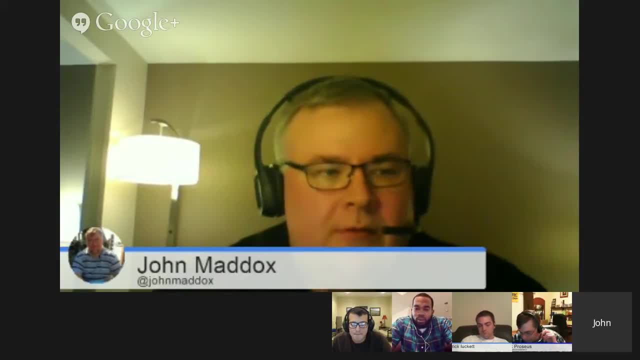 and not so much. don't get hung up on. oh, there's going to be 5 inches of snow. Just know that anything over a dusting is going to have a pretty strong impact on us, because we're different from other areas in that. 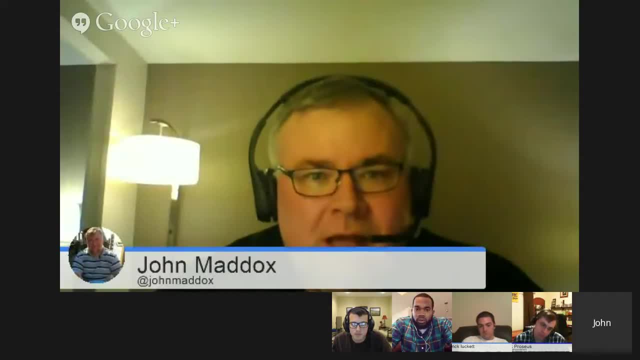 2 inches of snow. you know, last I checked, the city of Memphis owns a snow plow, So you know any sort of- you know- inclement weather like that's going to have a huge impact on your day. 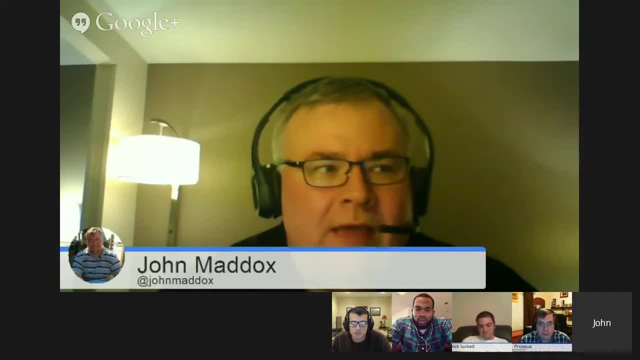 but it is. it's on us to not rely on that graphic that we saw Tuesday morning at 9 am. You know, get up 15 minutes early, Look at that forecast. You know the weather service is open 24 hours a day, 7 days a week. 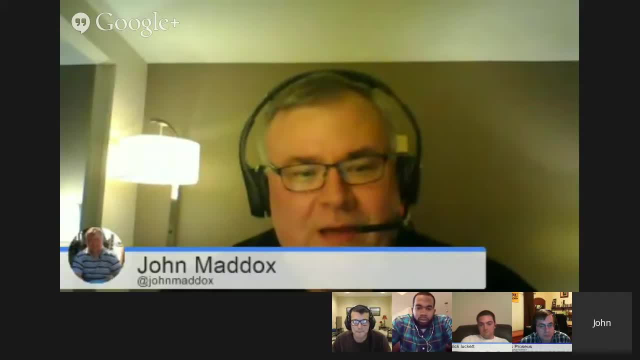 There's a new forecast that rolls out about 4 am every day, So get up a few minutes early. Look at it, And that's just what I tell people all the time. you know, and you guys are doing a much better job of this now. 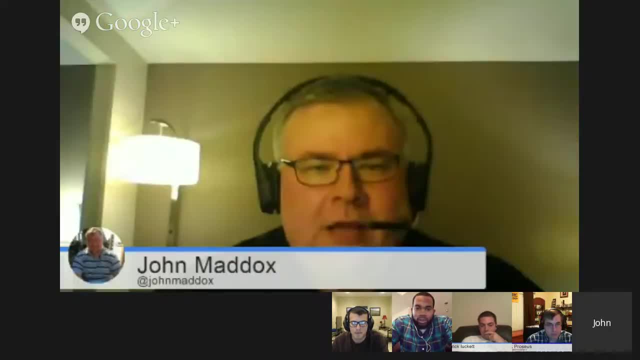 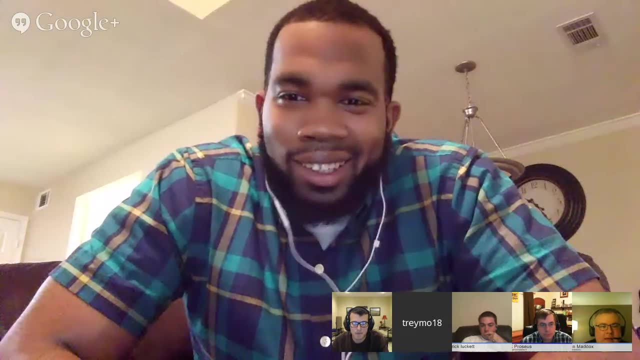 This could change This. you know, Eric John, you guys know, forecasting snow in the Mid-South is an inexact science at best, And it doesn't. you know, in New York it took a 50-mile switch Here. 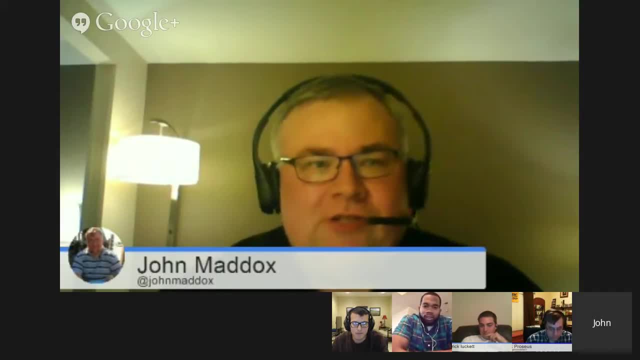 you could have a 10-mile, 15,, 20-mile switch and it changed the whole dynamic of the system for some buddy. The other thing about snow, as you guys know, is wherever that heavy band sets up is where it sets up, And you know somebody. 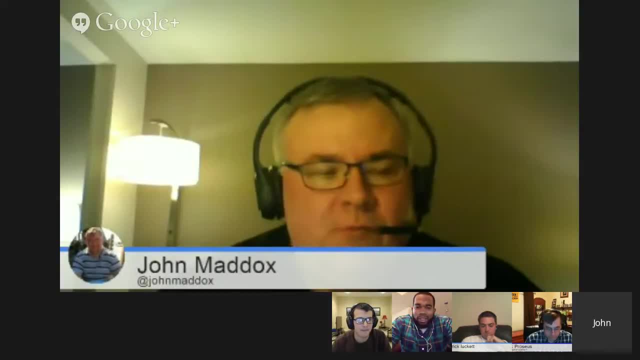 who's supposed to get a dusting gets two inches. So you know, it's just one of those things we just as consumers- it's just so important for us to stay on top of the weather and how it's going to affect me, And don't worry about. 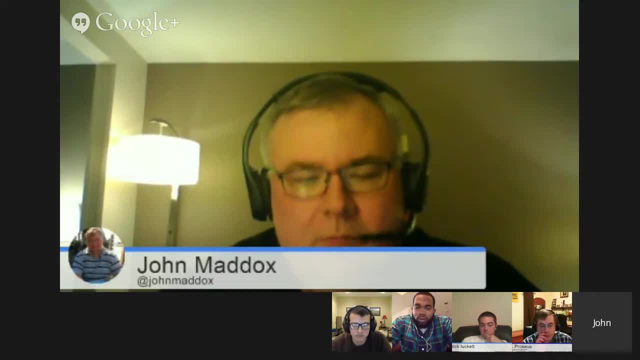 what my neighbor's getting, but worry about what you know, worry about what, how I need to prepare. And that's just not snow, I mean, that's tornado, severe weather or anything. Just you know, be prepared for yourself and keep yourself informed. 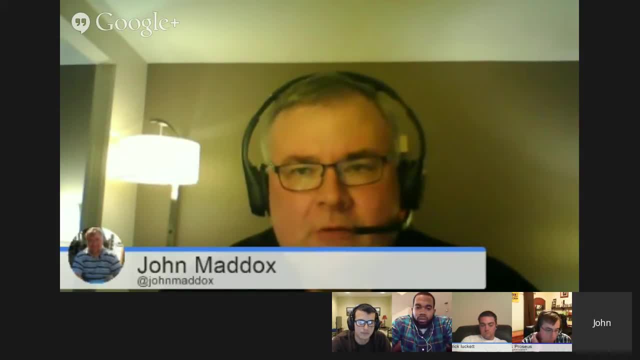 And this isn't 30 years ago where we had to rely on three TV channels to get our forecast. There are numerous sources of local live weather and please don't rely on the weather channel to give you a hyper local forecast. That drives me crazy. 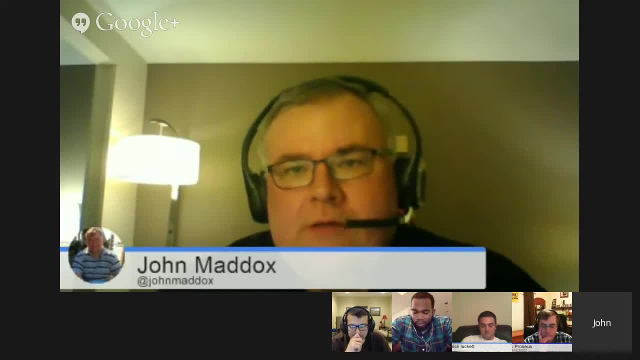 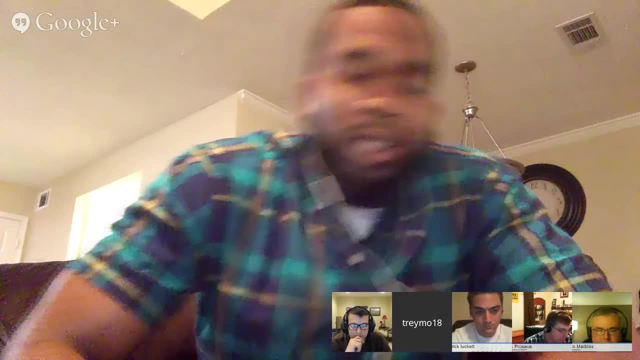 So you know, just have a couple of good sources for local weather, Know how it's going to affect you and just stay on top of it. Yeah, I couldn't agree more. John Couldn't agree more. Very good. 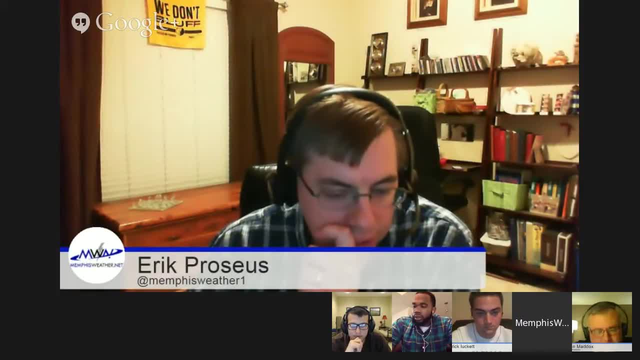 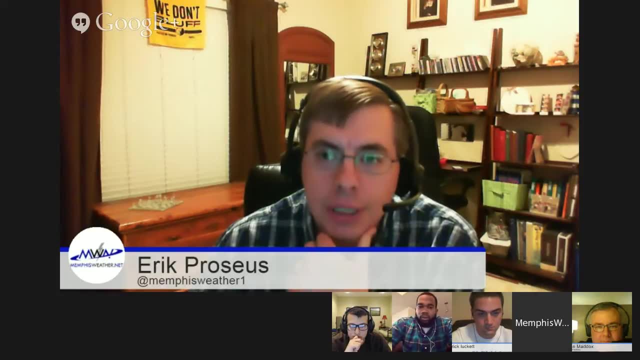 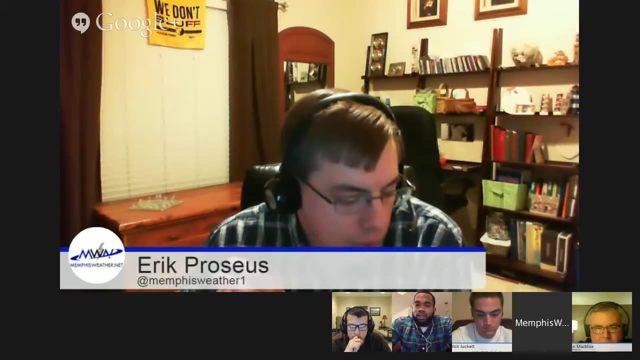 Great discussion. Yeah, there's, there's, you know it's. I think it's incumbent really on both sides of the equation to communicate effectively and to receive that information and process it and then act appropriately on that. So one of the things 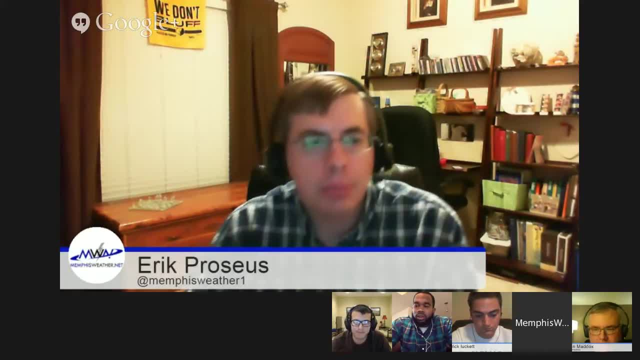 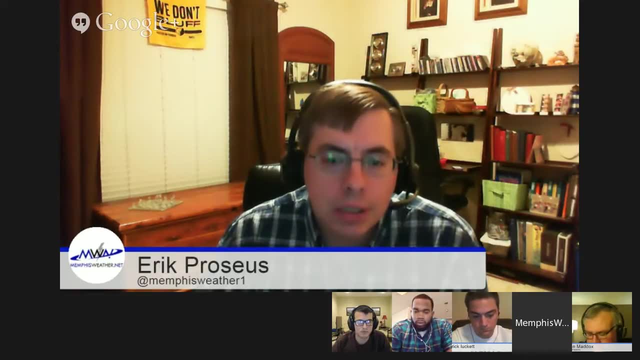 that was that William discussed just a little bit at the beginning when he was giving the briefing for the weather tomorrow night, and I'll just touch on it here again for a minute. that helps us in communicating uncertainty as far as some of the data we're looking at. 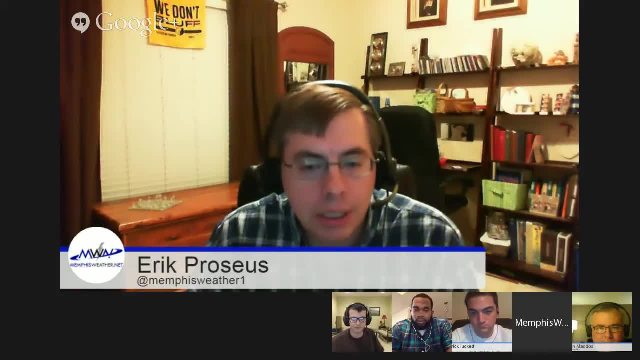 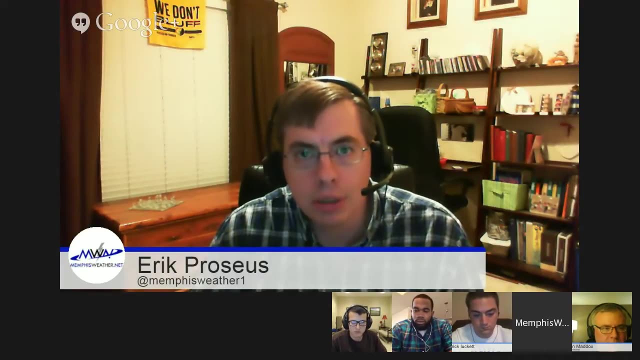 are these ensemble forecasts? And we kind of mentioned it here and there and I really probably should put together a full blog on what those are. But ensemble forecasts are basically where you have the same model, say it's the GFS model, the American model or it's the European model. 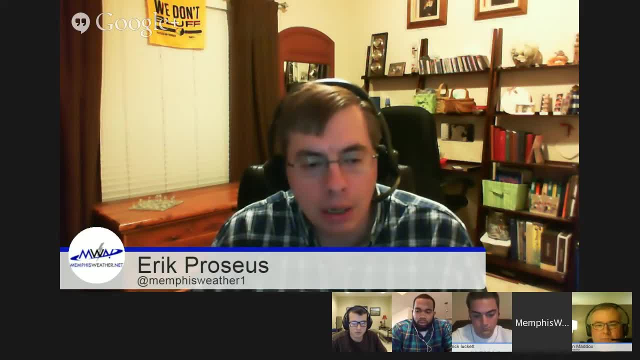 or some of the short-term models, And you basically run that model multiple times. You have the same initial conditions that are going in, but the model is tweaked slightly differently. You know the physics packages or the math, the physics that are done in the computer program itself. 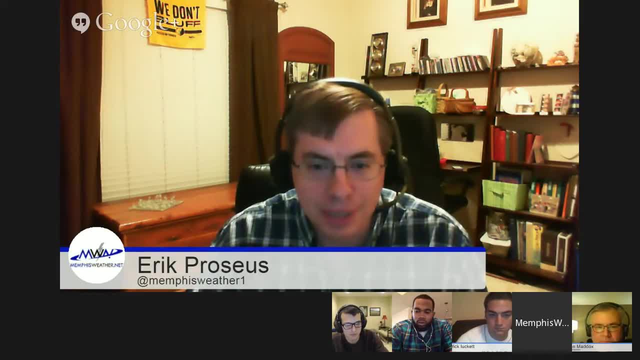 I was doing career day last week, I said this is kind of like video games for weather people. It's like this computer that's taking all this data and crunching it all around and we're playing games with it, But really it's just. 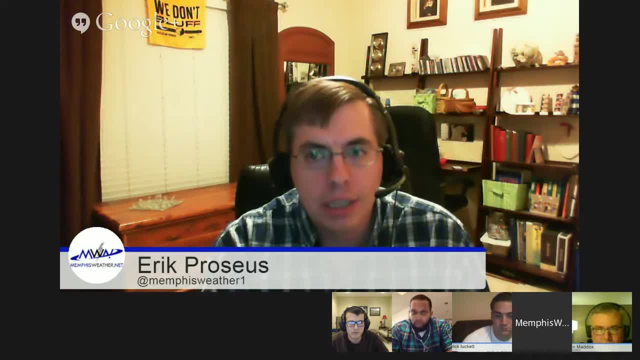 changing the equations just slightly to produce a slightly different result, And when you do that you get a range of possible options, And that's something that really until recently- I think in the last few years- hasn't gotten, even in the weather community, hasn't been. 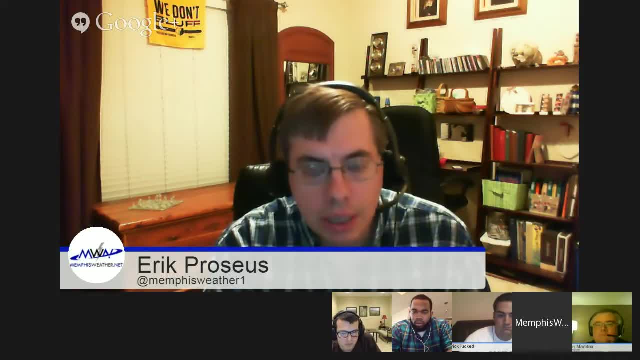 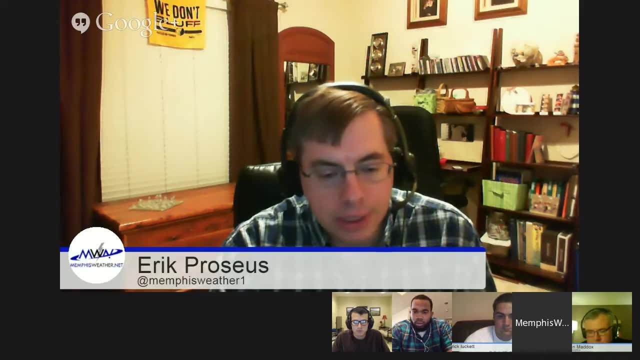 used a whole lot And we're really using it a lot now, And that basically creates kind of this window of possible opportunities. So if we have, for instance, one of the things I look at every day pretty much is the European, 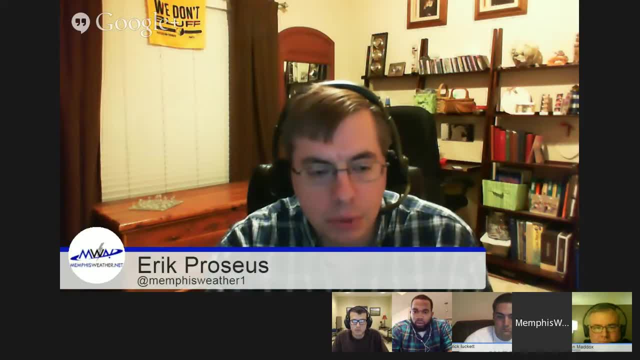 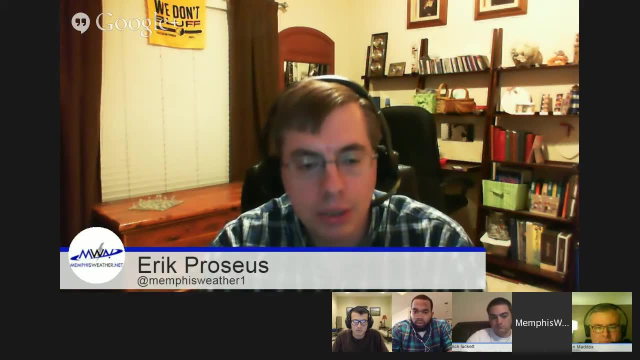 ensembles as far as temperatures and precipitation and so forth. And so if there are 50 members of the European ensemble- 51 members, which means that that model is run 51 times, And if all 51 give you the same solution with the same temperature, 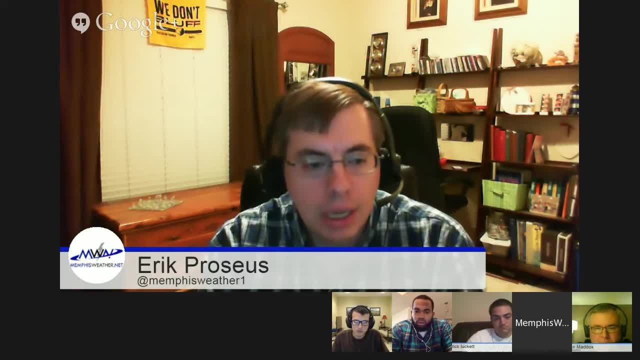 I have very high confidence that that is what is going to happen. On the other hand, if, three days from now, my range of temperatures are from 20 to 50, I know that there is a lot of- there's something coming through, whether it's a. 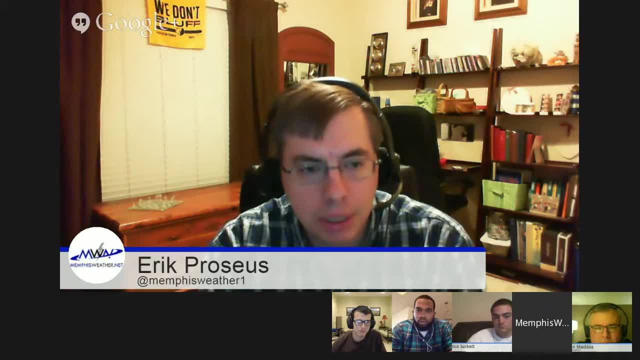 timing of a front or whatever it is that's going to create a possibility for a wide range of solutions, And so this uncertainty factor goes up and I have to account for that. I have to. you know, when I do the forecast I may pick a number. 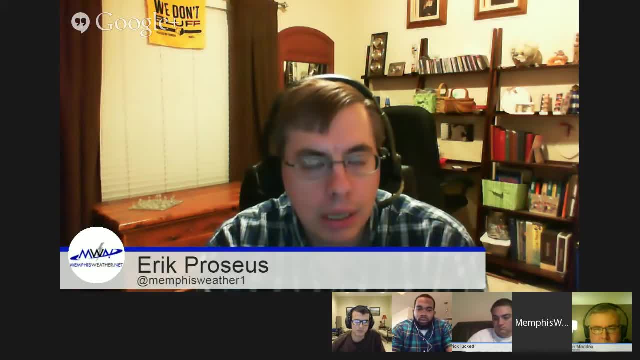 or whatever. but I have to account for that somehow by letting you know that you know if the front comes a little earlier, the temperature is going to drop, for instance tomorrow night. You know if that front were to come through here three hours earlier. 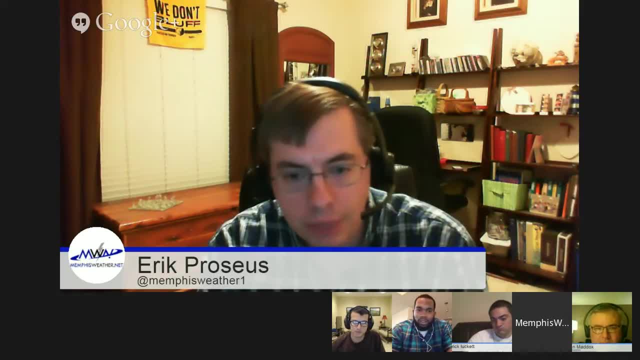 tomorrow night and we get the same precip, we're going to be looking at more snow than if it comes through four hours later. So that's a part of that communicating that uncertainty, I think, is we've got more tools basically in our tool belt. 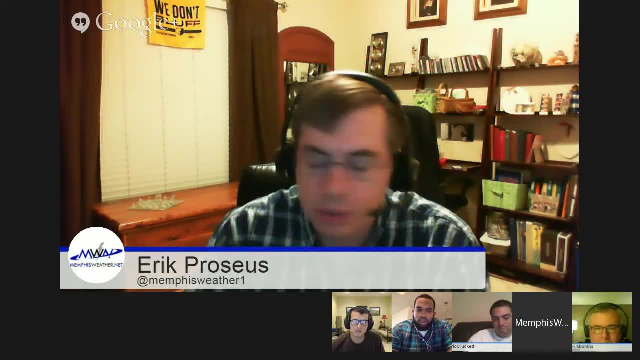 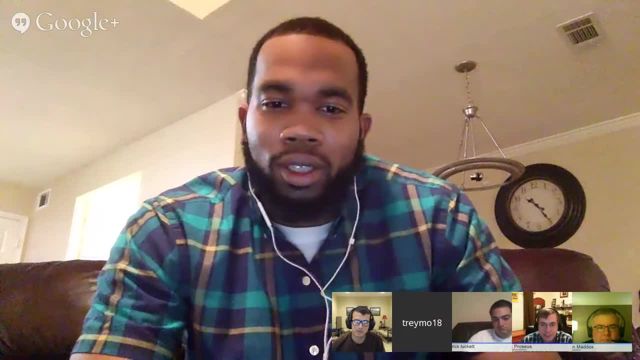 as meteorologists than we did just a few years ago. And I know you guys at the Weather Service are doing all that as well. We're trying, we're trying. It's almost overwhelming the amount of data that's coming at us these days. It's really hard to go pour through. 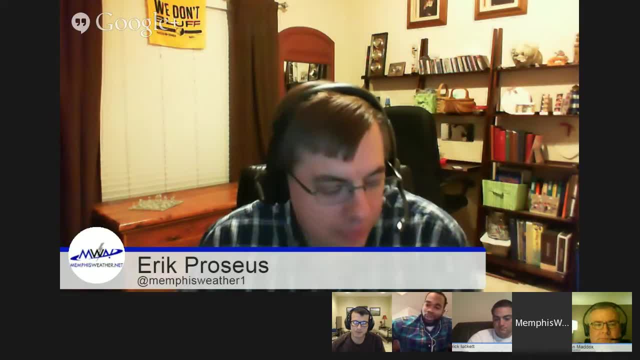 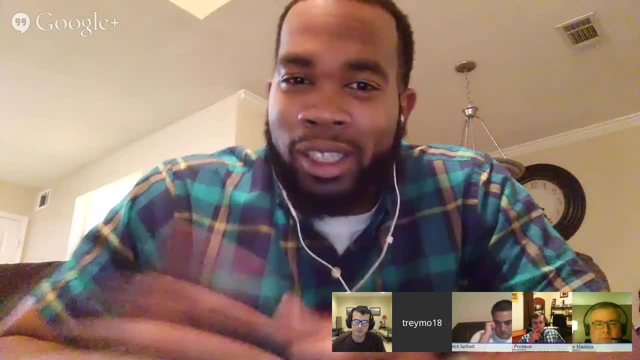 it all. You pick and choose, but One of the main things we're working on now is coordination between offices, so it's the biggest problem we're working on now, especially with the storm in the northeast. That's probably why the gradient got. 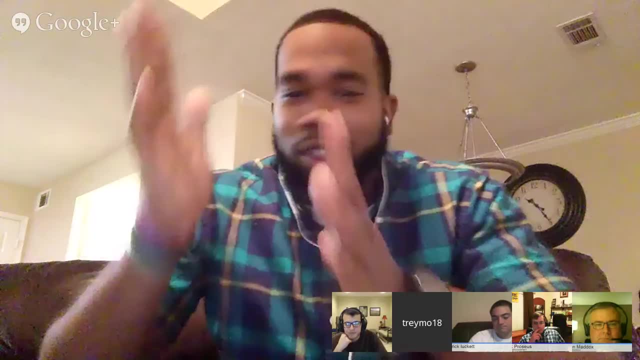 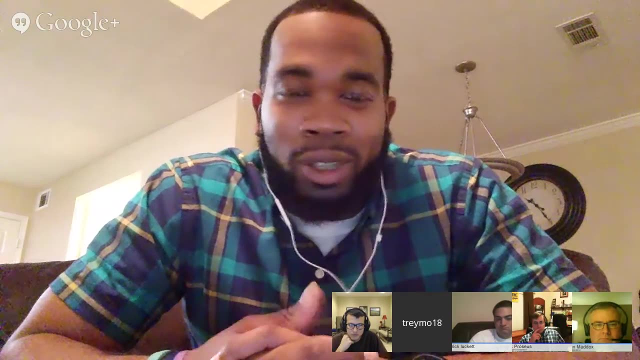 pushed back kind of. We've got all these offices trying to collaborate on the same gradient line and each office continues. It's a push it and push it back to the other office's territory or CWA. So we've got to. 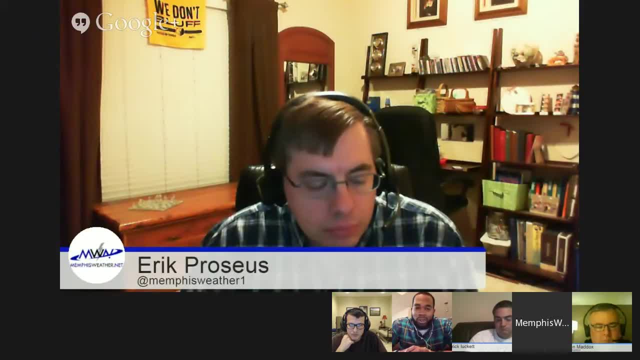 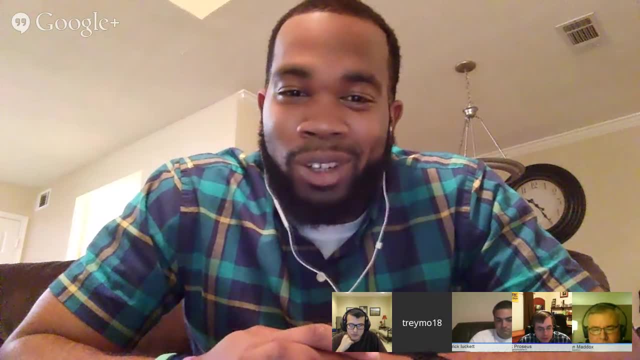 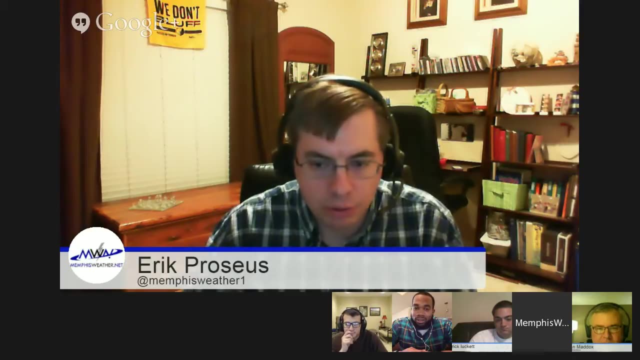 get a lot better at coordination between offices. And weather has no boundaries. It doesn't care about the CWA border. so that's what we're working on now: collaboration. And it's more visible these days as well, because you're not just tuned in to your little local forecast. 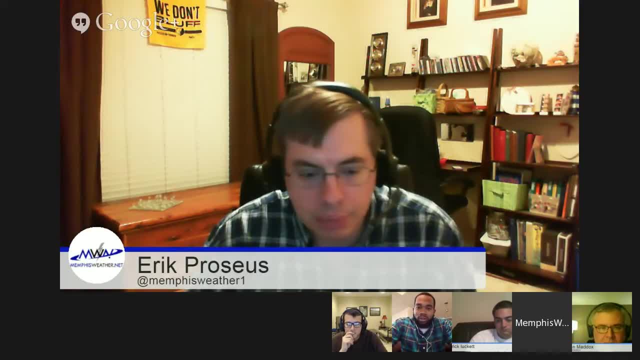 and don't know what the forecast is. 50 miles up the road You've got these graphics that are national graphics that basically blend all of your data from all the offices together. It's pretty easy to see some discontinuities in there when you're 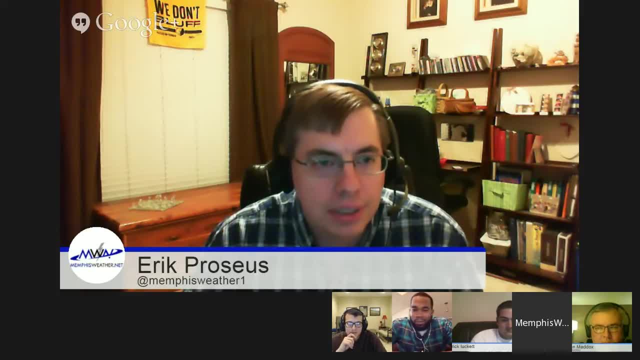 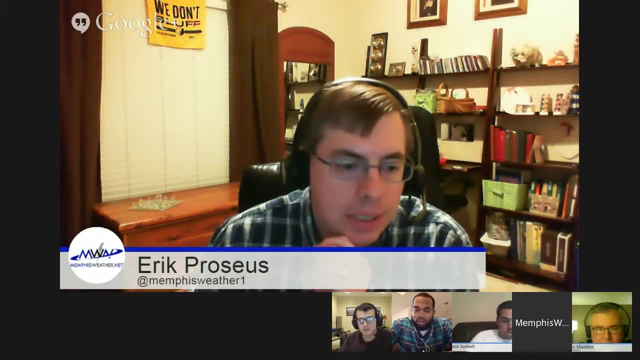 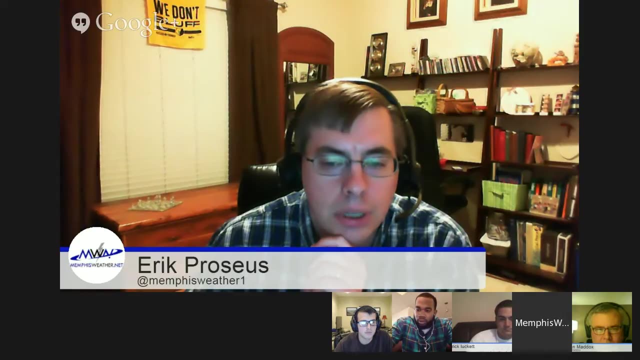 trying to time a front through or something like that. so it's a little more obvious. So I think that's most of the topics I wanted to talk about. I'm not seeing anything on the chat in particular question-wise. Either one of you, Patrick or William, see. 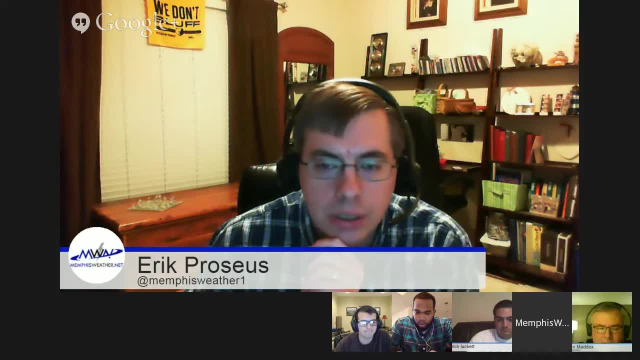 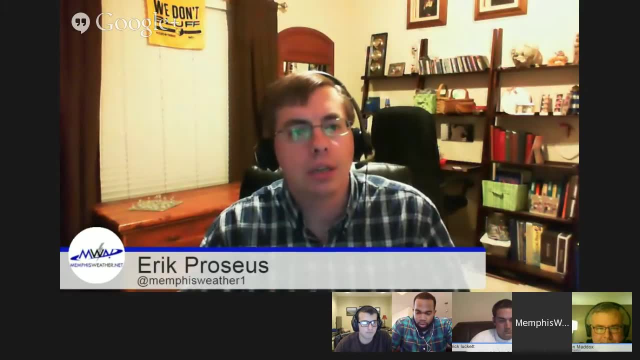 anything coming in that we need to answer while we're on tonight. I haven't seen anything. Okay, cool, I guess I'll just run around one more time here. if anybody's got any closing comments, John Maddox, I'll start with you. 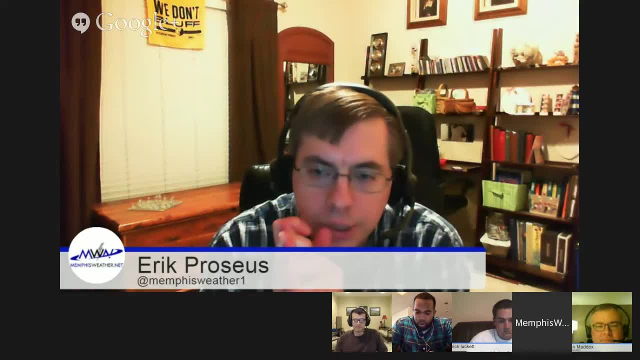 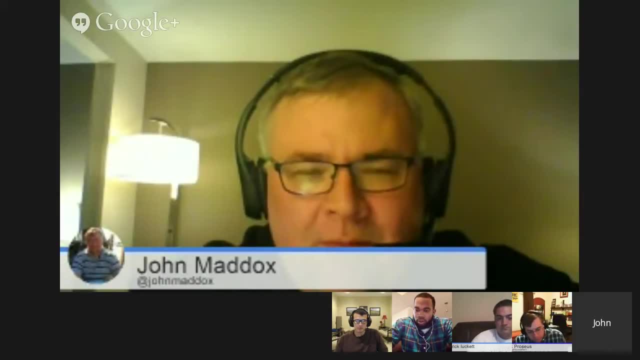 and appreciate you joining us again tonight. If you've got any other closing comments, feel free. No problem. Thanks for having me on again. Appreciate it. And John Moore, I think I'm probably correct. I'll be lucky if I see one. 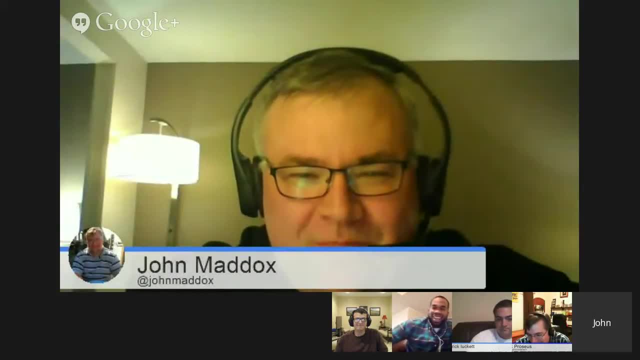 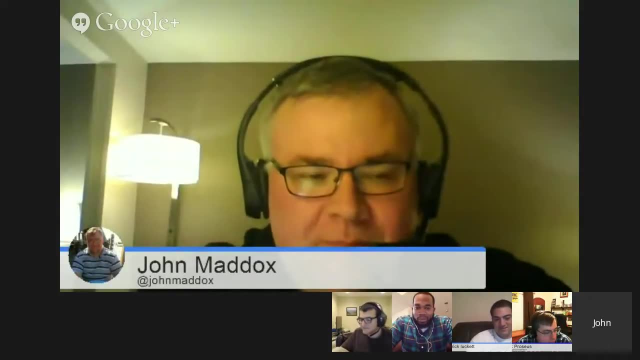 solitary snowflake down here in Tupelo on Thursday morning. That's about it. But yeah, so just everybody. just give yourself 15 extra minutes on Thursday morning. I know to some people, and me included, that seems like a lot of time. 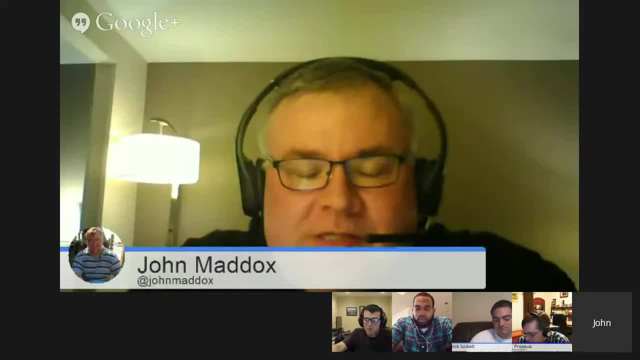 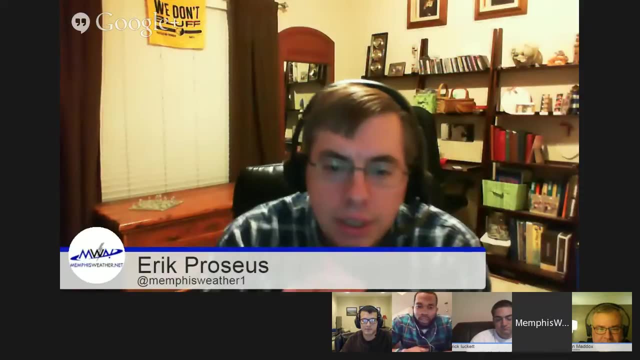 but just give yourself a few extra minutes and, you know, be prepared for even a dusting. as we said earlier, can cause all kinds of problems. So thanks for having me on, Eric. Yep, you're welcome, John John Moore. 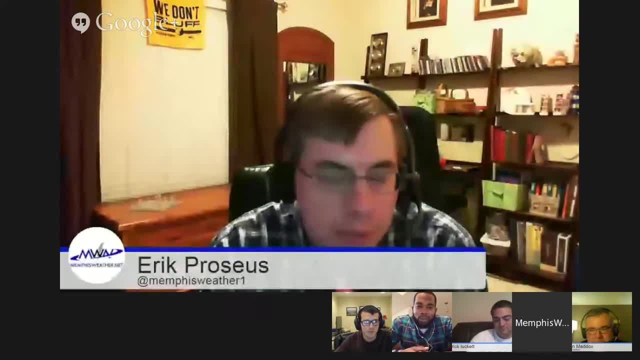 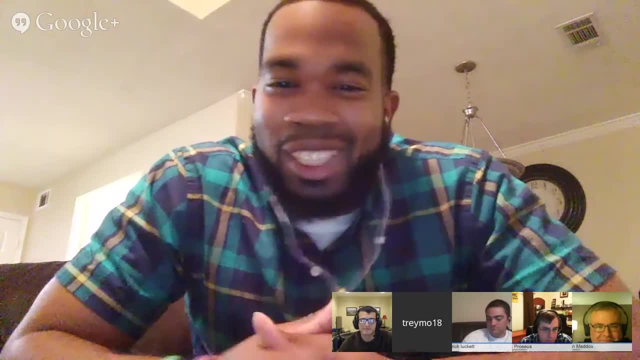 switch over to you. Thanks again so much for joining us tonight. Appreciate the weather service. No problem, no problem. Same thing John said. You want to always be prepared for the worst. hope for the best And maybe it'll land somewhere in the. 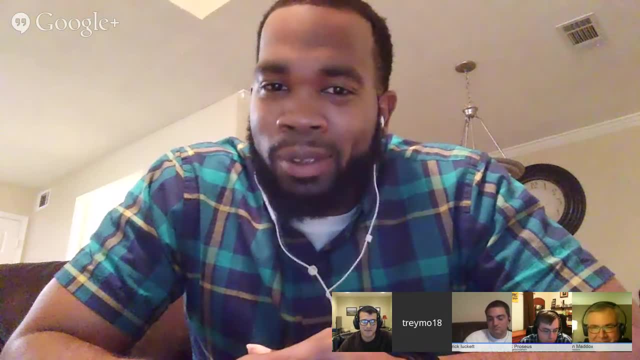 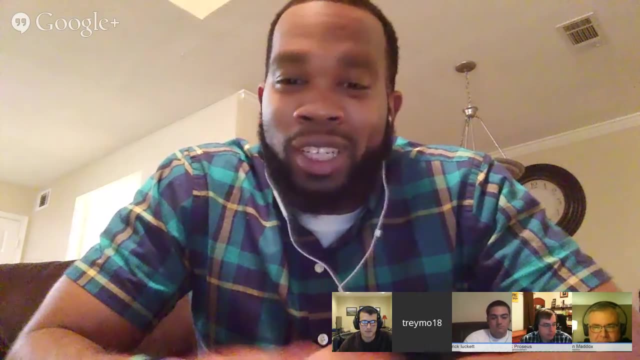 middle. And one thing I want to plug is actually: you talked about the Tennessee Severe Weather Awareness Week. Next week is Mississippi's Severe Weather Awareness Week and this is something groundbreaking we're trying now. We're going to have a Google Hangout session Monday. 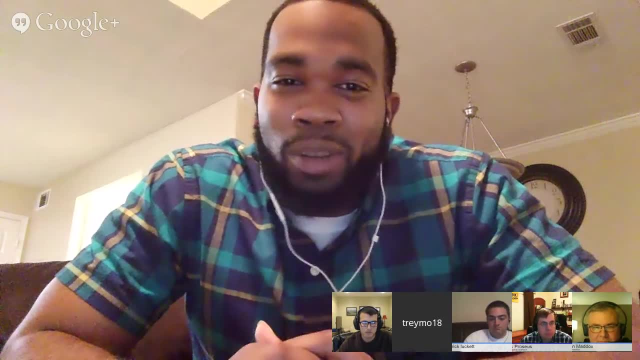 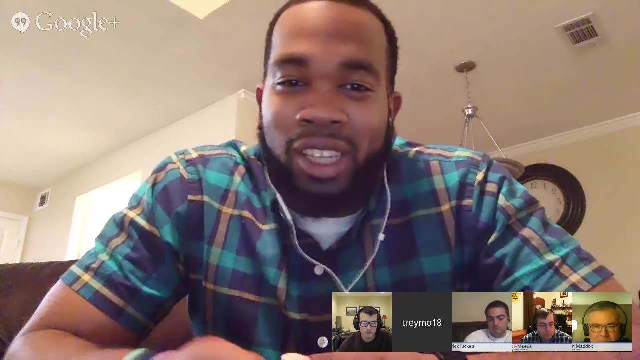 at 7 pm. We haven't started promoting it yet, but we'll start promoting it tomorrow between offices. So it'll be our office Jackson office, National Weather Service in New Orleans, and we'll have the LMRFC, which is the Lower 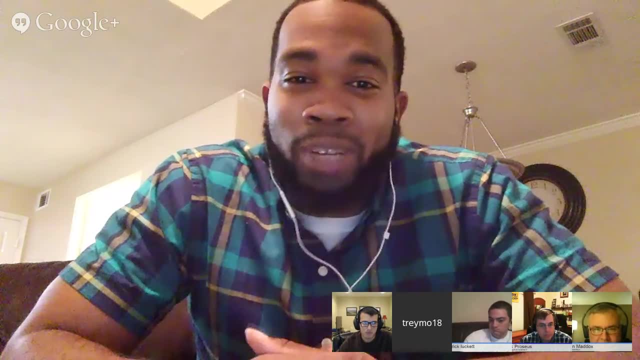 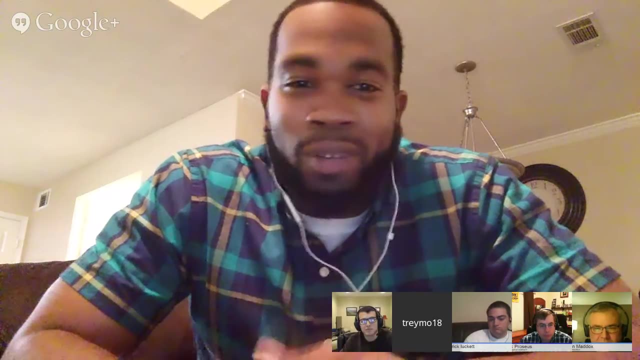 Mississippi River Forecast Center on, And even Rich Thompson from the SPC is going to give a talk also. So we'll have all those offices on Monday at 7 pm And we'll try to reach everyone in Mississippi or anyone who wants to watch, And we'll 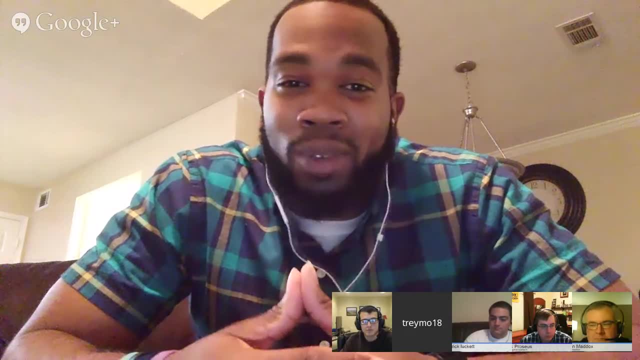 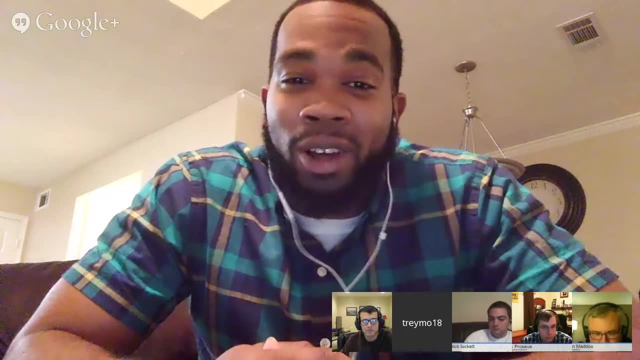 tell you what we do as a weather service and give a spring outlook of what we think is going to come And, along with some severe weather tips, tornado tips, climatology- those are going to be about an hour long And we're going to try to do. 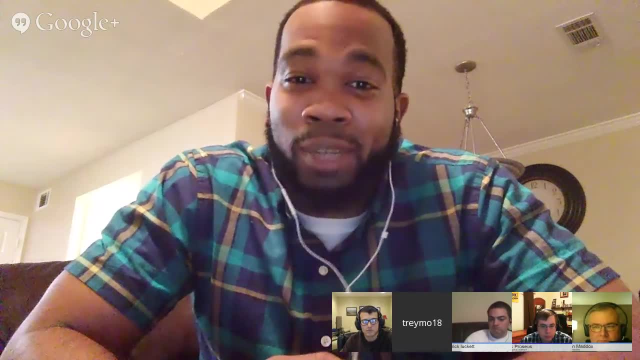 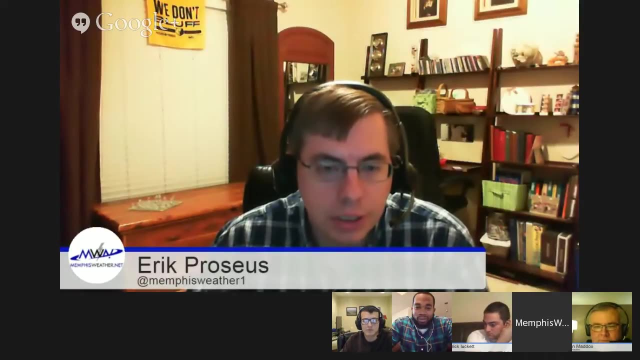 one of those each of the following weeks, I know for Tennessee especially. So I've got to talk with you about that, Eric, and try to get you involved in that one for Tennessee. Absolutely, Look forward to it. That's good. Glad to see the weather service. 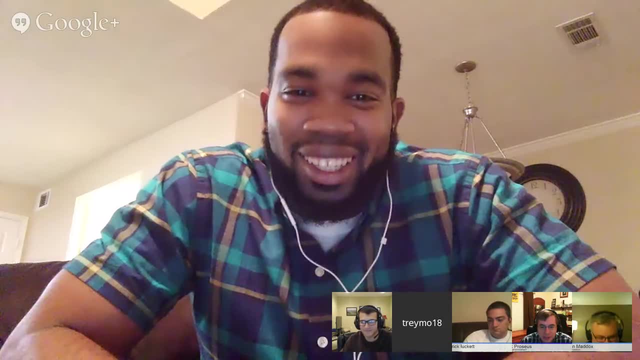 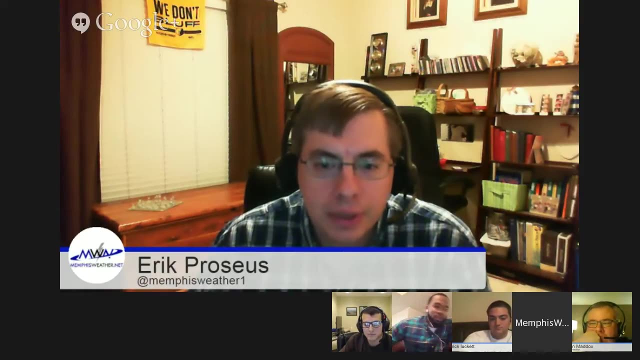 getting high tech here and finding new ways of getting the information out. So look forward to that. We'll make note of it And when I see your social media posts and so forth, we'll make sure we spread those around. Yeah, Looking forward to that tomorrow. 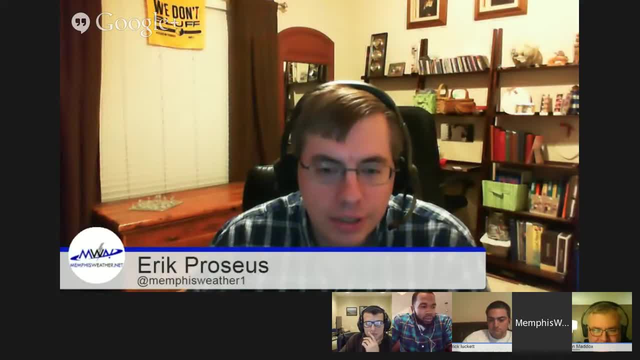 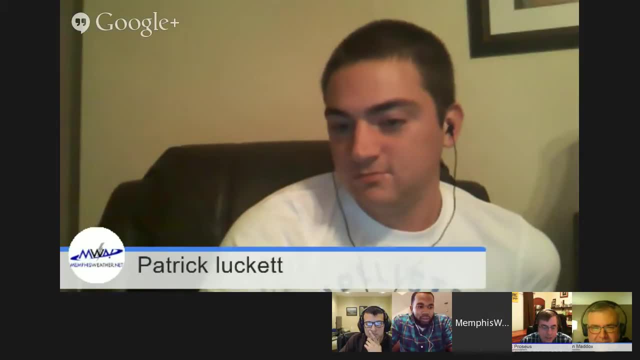 All right. Thank you, Patrick. any closing thoughts or comments? No, I think we had a good discussion tonight. Good Appreciate you joining, as always. Thanks for tweeting out as well, And for those that couldn't join, appreciate that. 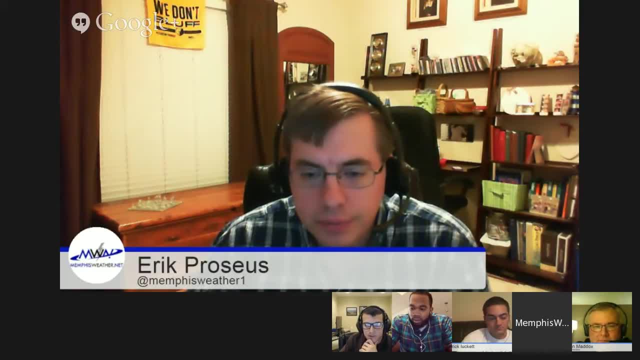 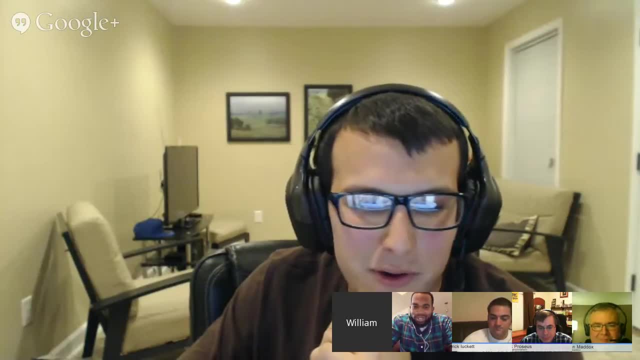 And William, anything closing in you? Well, I guess I'll just say, John, that sounds pretty cool And I'm sure I won't be the only one tuning in here in Starkville. We'll probably get quite a few weather weenies here tuning into that. 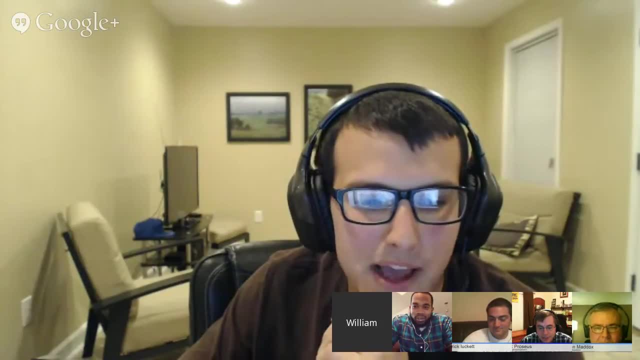 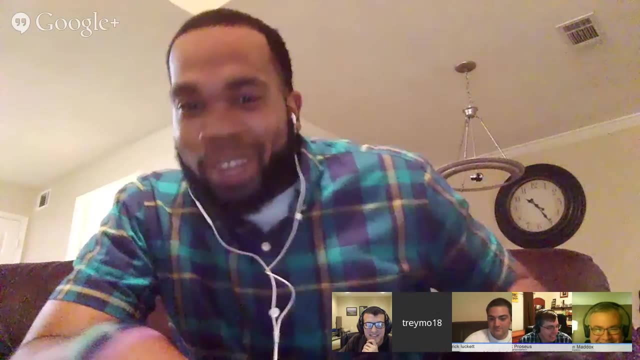 So but yeah, good discussion And I'm excited to see what happens And hopefully it falls within the weather service's control And I'll see you in the weather service range. Yeah, We got some big-time weather hitters. Some big-time heavy hitters are. 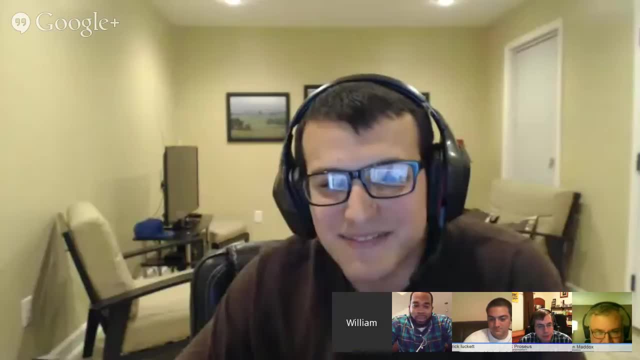 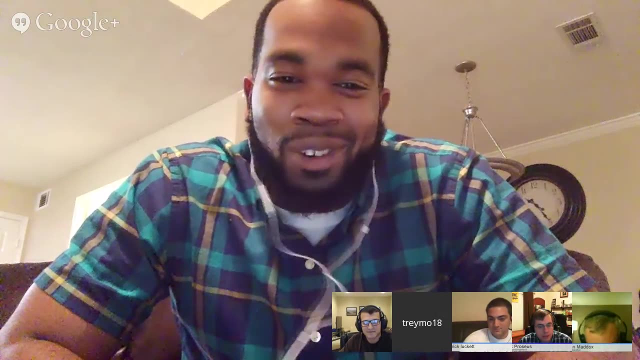 going to be on there next week. We got Rich Thompson from SWC. I'm pretty sure I knew WCM Gary Woodall is one of the best WCMs in the weather service, one of the best meteorologists in the weather service overall, in my opinion, Guy's. 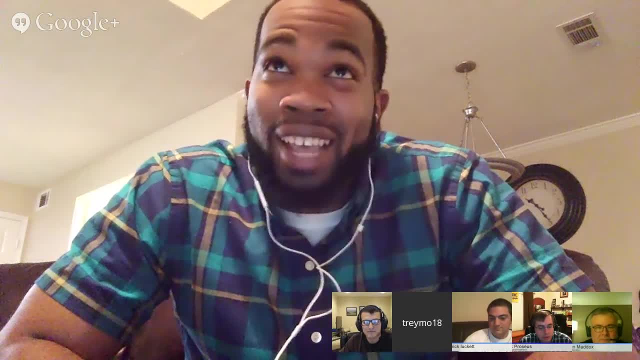 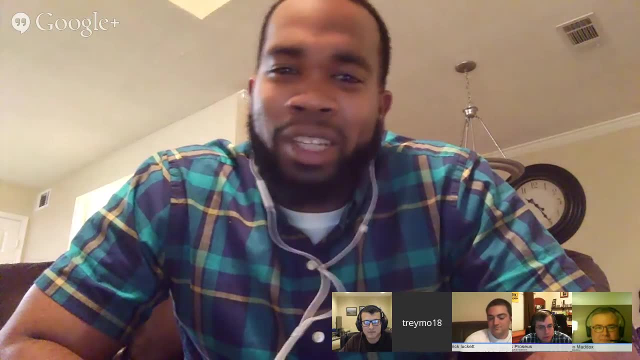 great, And we're going to have Joanne Cullen from down in Jackson. She's going to give a brief talk, And I'm not sure about New Orleans yet, but I believe it's going to be. Frank Rivette is going to give their talk, So I'm going to give. 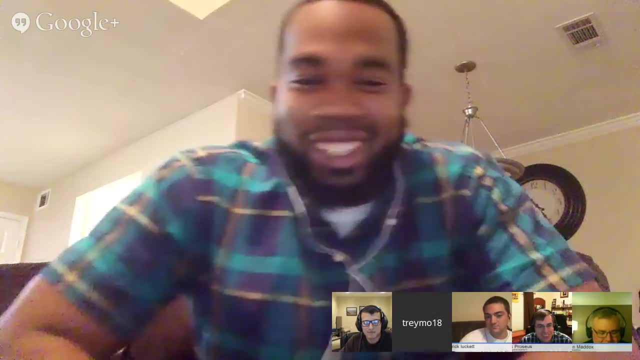 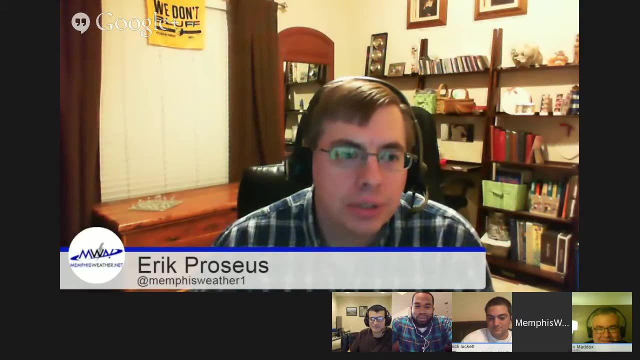 a brief talk. So yeah, we got a bunch of weather all-stars on deck for next week. Excellent, Excellent, That sounds great. All right, Well, I'll appreciate you guys joining in tonight again, And for those of you that may be tuning in late, didn't. 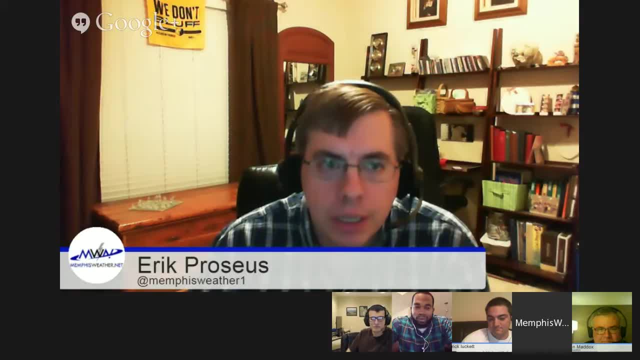 get to watch the whole thing. this will be on YouTube on the MemphisWeathernet official channel, So feel free to watch that. I will post out a link as well. And yeah, Tennessee Severe Weather Awareness Week is coming up in three weeks or two.